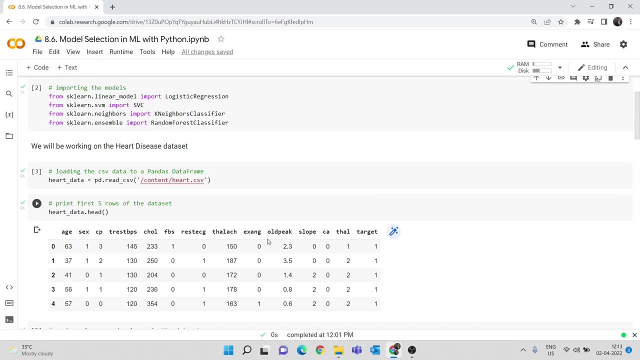 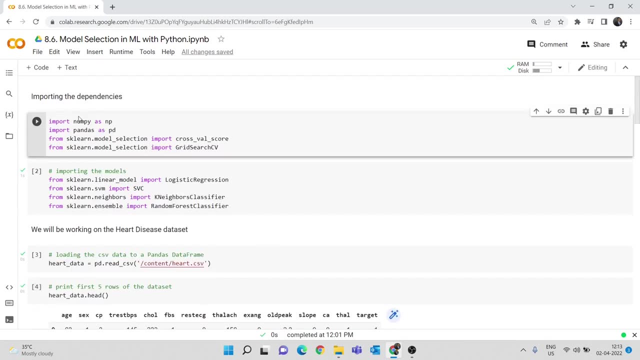 problem and in this case we are going to take 5 models and compare their accuracies and see how we can perform this model selection. So that is what we are going to do in this particular video. So these are the steps that I have already done in that video as well. 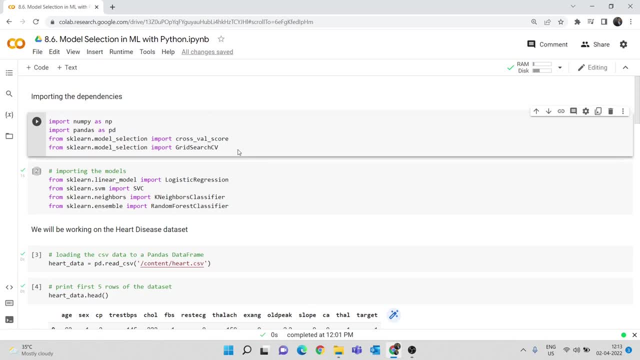 but I will quickly explain you what are all the steps that we are doing here. So the first step is importing the dependencies. Dependencies are nothing but the libraries and the functions that we need. So first of all, I am importing the numpy library and Pandas library, and from sklearnmodel-selection we are importing 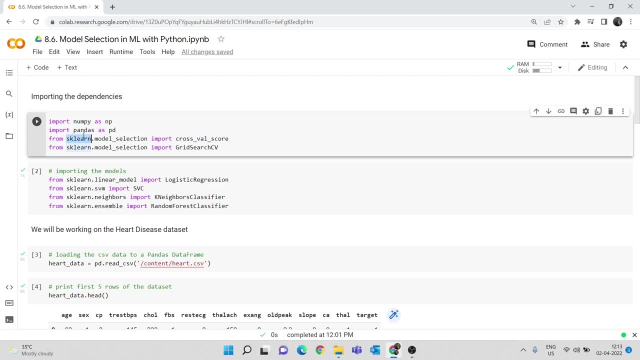 crossvalued score. so in sklearn library we know that in sklearn we have various functions for training our models, several models like logistic, regression, selective machine, etc. So there is also a module called as model selection, in that we have a function called as crossvalued score which is basically gives us the crossvalidation score of a particular 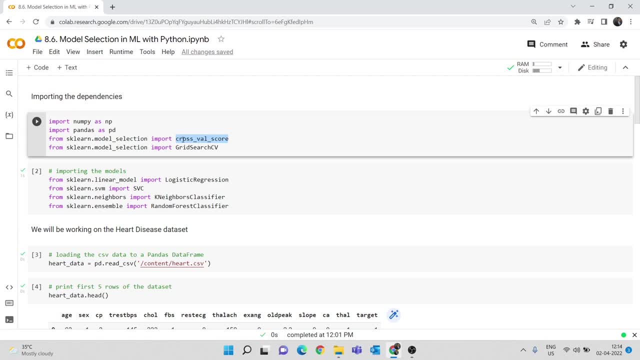 model and we have already seen this. while we have discussed about this k-fold, crossvaluable, cross validation and all of those things, i hope that you have seen those videos. if not, i'll give the link for that video as well. in this video description for this rdesis prediction also, i'll 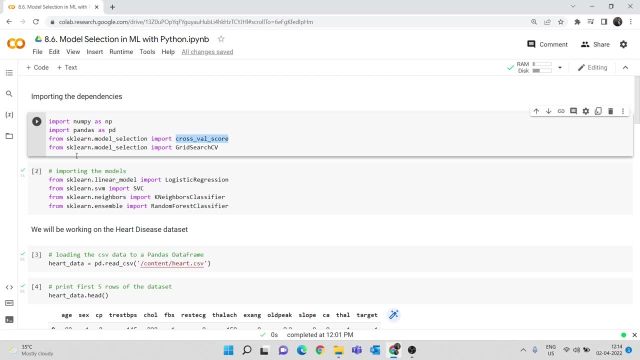 give the video in this description, okay, so i'll give the link for that. and then we are importing this grid search cv. so grid search cv is what we call a hyper parameter tuning technique, where we pass, like, several hyper parameter values and this grid search cv will try to tell us which. 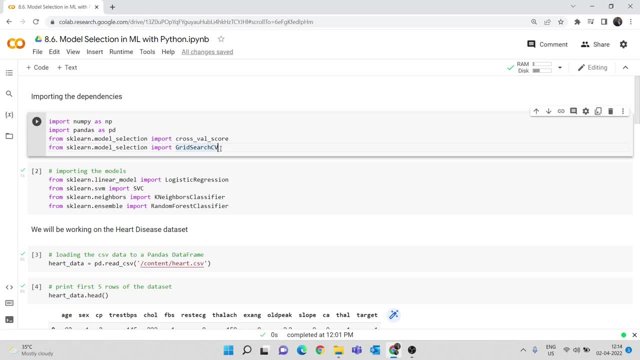 hyper parameter is the best that we can consider best, in the sense when you use those hyper parameters you will get the highest accuracy for that machine learning model. so we are importing these four dependencies first of all, and later we are importing the models that we are going to use. 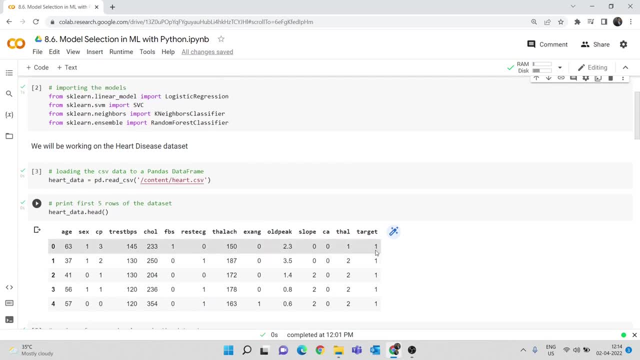 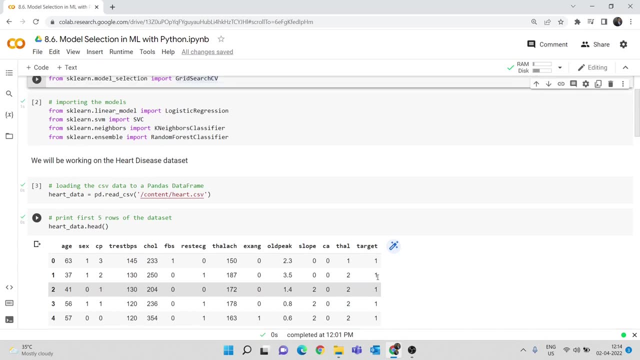 so in this case, as i have told you, this is a classification problem because this contains the target variable as either one or zero, one being a person as rdesis, and zero being a person doesn't have any rdesis. so this is a classification problem. so we are importing five classification. 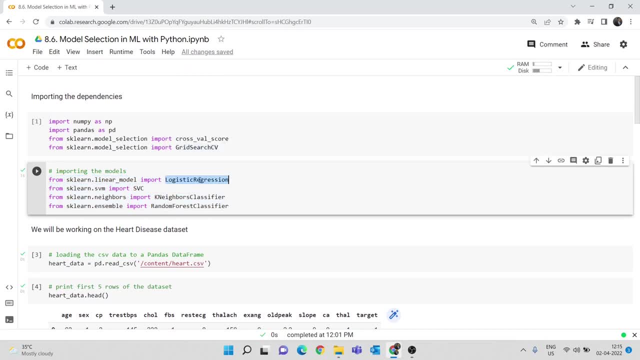 models that we have. the first classification model that we are importing is logistic regression, which we are importing from ssr scale and dot linear model. then we are importing the support vector classifier, then k nearest neighbor classifier and random forest classifier. so these are all the five models that we are going. 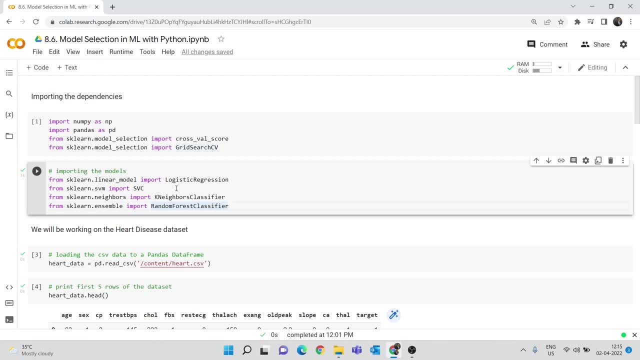 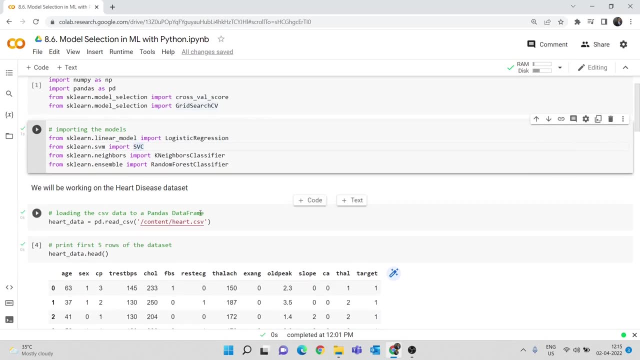 to take and we will be, you know, comparing their accuracies. okay, so i think like there are like four uh models, not uh five models. there are like four models which you are going to use and, as i have told you, this is the rdesis uh prediction data set. i'll give the link for this data set. 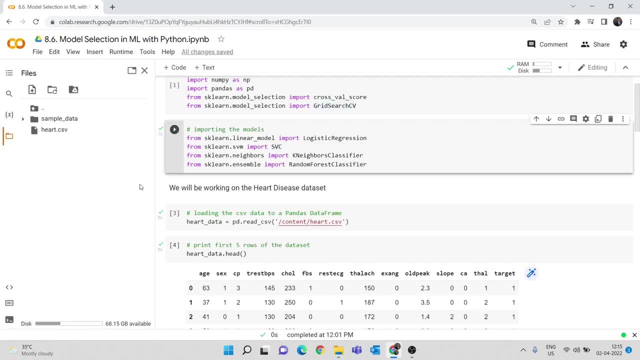 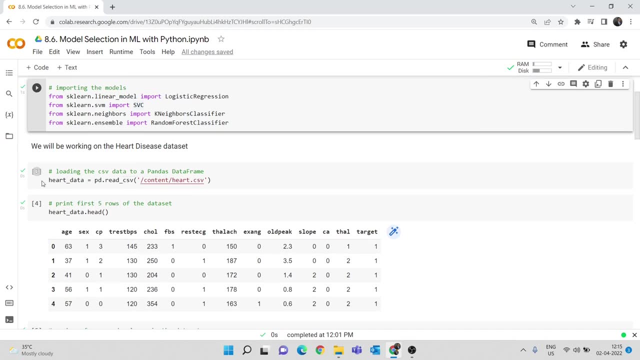 in the description of this video as well. you can download that file and upload it here. so i have already uploaded this file, so you can upload it here and and do all these processings. so once i upload this uh file, i'm reading the csp file to a panda's. 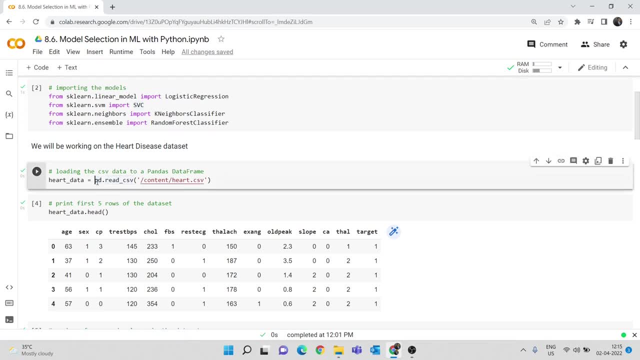 data frame using this read csp function. so we know that this is a very common and basic uh function that we use and i'm storing this data in a data frame called as art data. okay, so in this i have to give the path of the csp file. after that i'm printing the first five rows of the data frame. 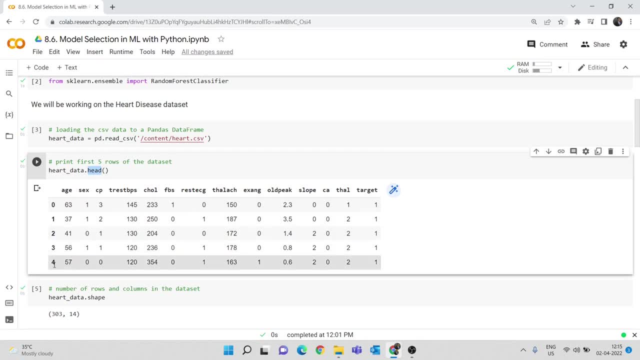 that i've created using the seed function. so these are all the first five rows that we have. so if you want a clear, detailed explanation on what are all these different columns that we have and the other things, you can watch that, uh, our decision prediction project. so here i'm just. 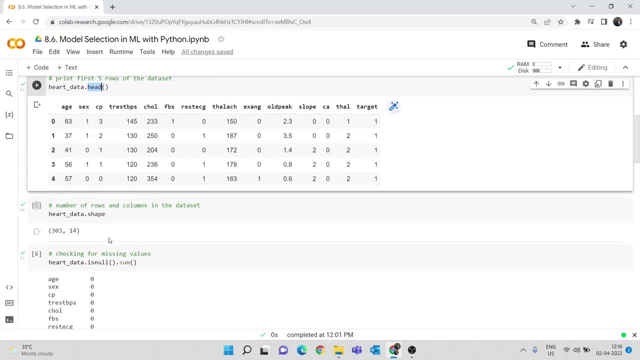 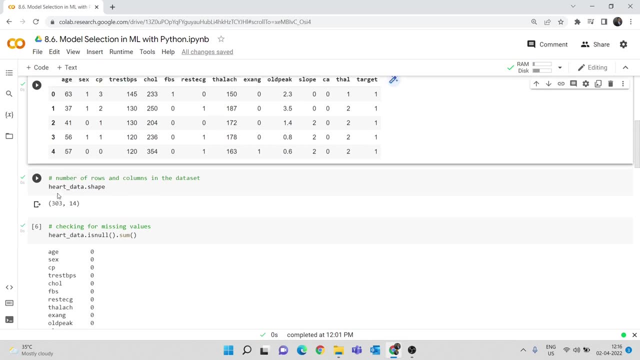 quickly going through all the steps that we have done and then we are checking the shape. so how many rows and columns are there in this particular data frame? so, as we can see, there are 303 rows and 14 columns. okay, 303 means 303 data points, or 303 different people are there in this data frame. 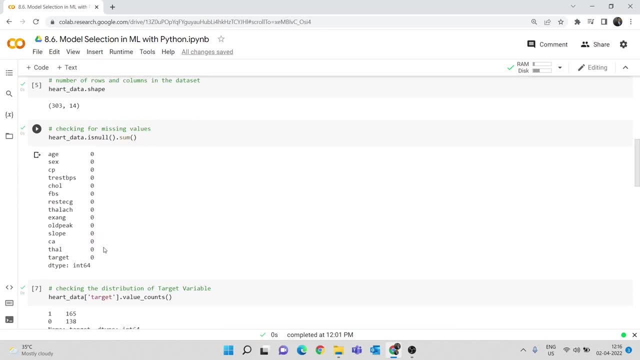 and we are checking whether there are any missing values. fortunately, there are no missing values in this data set, so we can move on to the next step. then we are checking, uh, the distribution of the data frame. here, as you can see, i'm mentioning the data frame name and the target column name, and 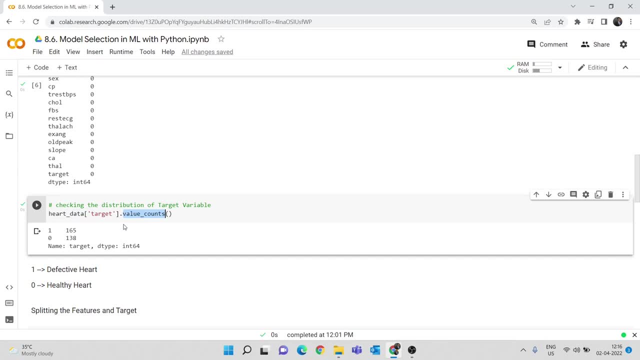 value form. so this is the function that tells me how many values are there in each class. so there are like 165 data points in one class and 138 data points in the class 0. so the distribution is almost equal. so we don't have to do anything. so in case the distribution is not even in that case, 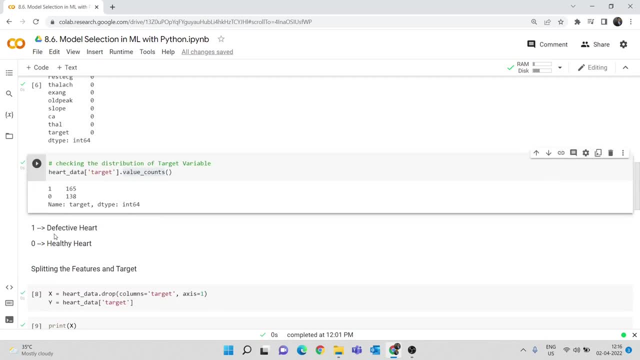 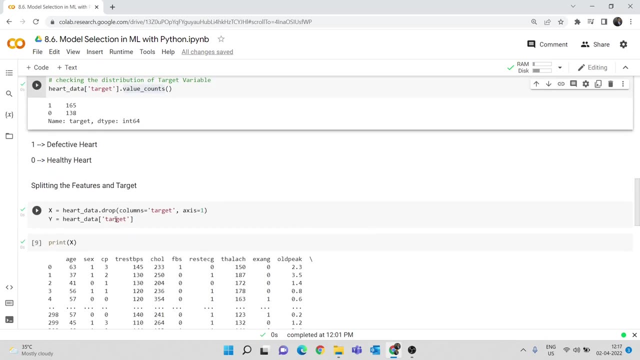 we have to do up sampling, down sampling and so on. so here, 1 means defective art, that means like a person is suffering from uh art. this is 0 means a person doesn't have any artists, and so on. so now we are separating these features and target features are nothing but these columns. so we 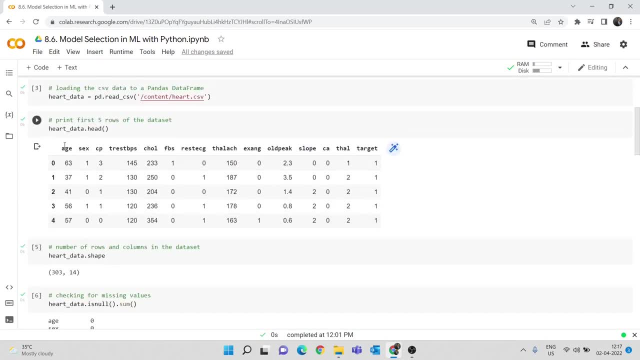 have this eh, 6, cp, you know bps and so on. so we have various columns here and one column is this: cholesterol and so on. so based on these factors, we have to tell whether a person will be having- you know our disease or not, whether the value is one or zero. so these columns from eh to this. 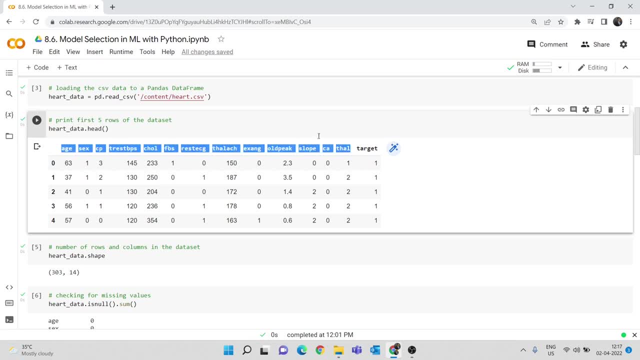 uh. last before column is my features, because with using these values, i'm going to predict whether the target value is one or zero. okay, so i'm going to separate all these values separately and target uh column separately. so that's what i'm doing here. so i'm storing all the features in my x. 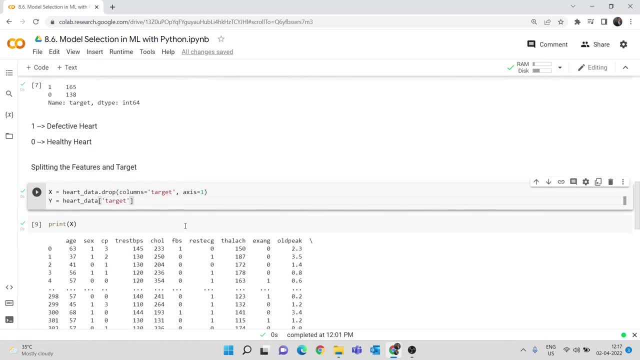 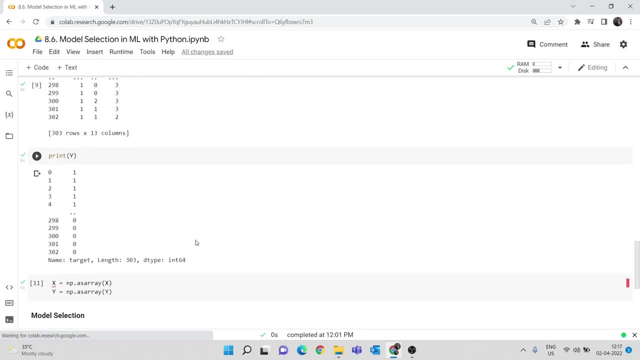 and i'm storing my target column in this point. okay, so i'm separating it and you can see i'm printing my x. so these are all the columns. now it doesn't have this target column and y as the target column. so these are all the things that we have done so far and after this, we can perform our. 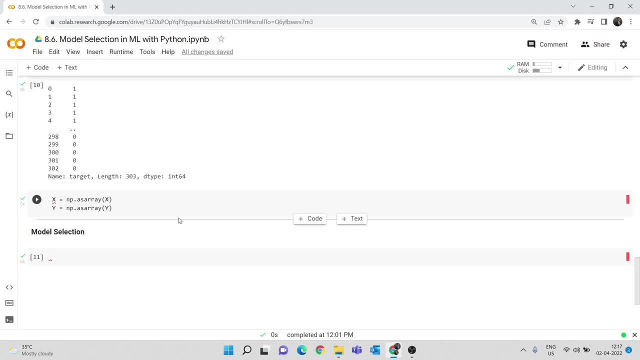 model selection. uh, steps that we have. okay, so you don't have to separate the data, screening data and test data. so we will do that in the later part of the code, but you don't have to do that. so i'm separating my features and target as x and y and after that i am converting it to a numpy. 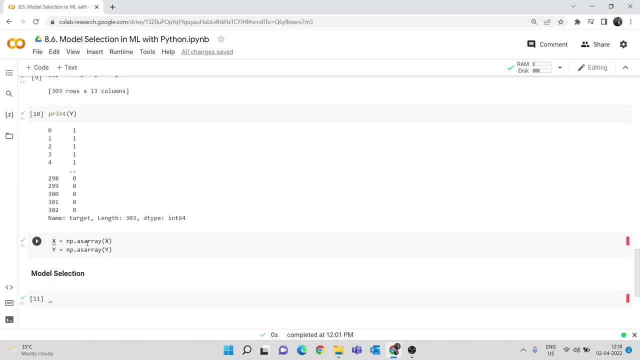 array. so instead of having it in the form of data frame or a series, i'm converting it to a numpy array, and you can do that by using np. so np means numpy library, using as array function x. so i'm converting this x into a number array, y into a number. okay, and now we will do this. model selection. 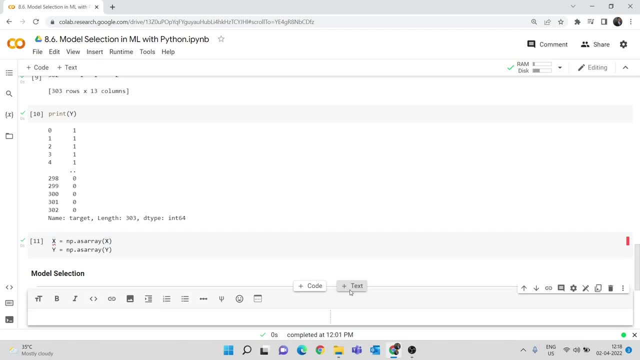 so in this model selection, we will perform like, uh, two ways, like two things we will do here. one is like comparing the models with the default hypertext parameter values, and then we will also compare the model, or we will, you know, select the models with the different hyper parameters. okay, so first thing that we will do is i'll just make 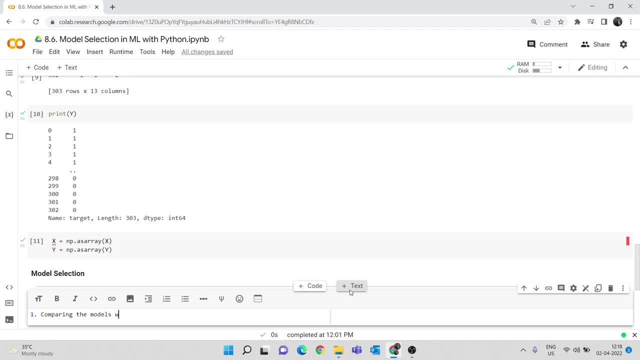 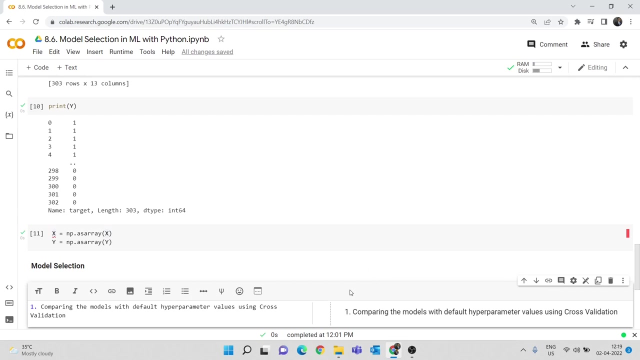 a text here as comparing the models with default hyper parameter values. okay, so default hyper parameter values using cross validation. so this is why i've imported cross valscore function- cross validation. okay, so this will be the first step and later we will compare the models with different type. 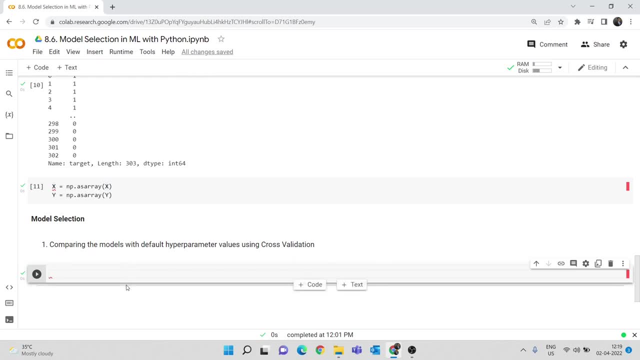 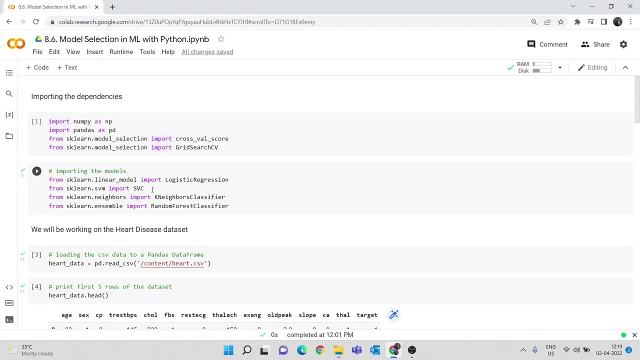 of parameters as well. so there are like two parts for this particular video and first of all let's try to create a list that contain all these uh models. so we have imported this. models right, logistic regression, svc k, nearest neighbor and random forest classified. so here i'm going to. 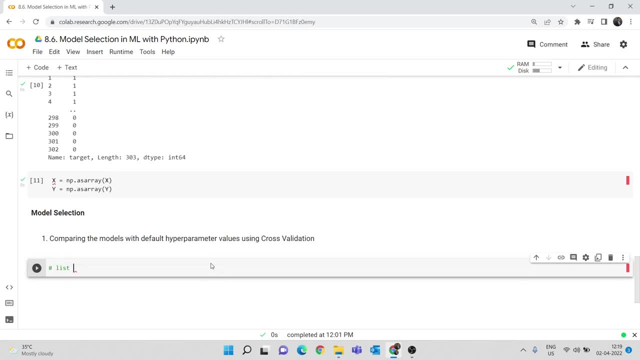 create a list. so this will be a list of the models that we are going to create, and then we are going to create a list of models. you can also try other classification models as well, if you want. so models is equal to. so this is the list that i'm creating. the first model is logistic regression. 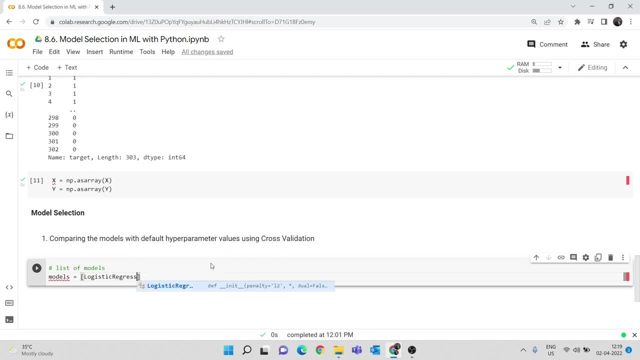 okay, so logistic regression. so this is my first model, and the second model is support classifier, which is svc, and k- nearest neighbors. so k neighbors classifier is my third model and finally, i have my random forest classifier- random forest classifier. so these are all the four models that i'm taking and i'm going to like give a few values to it. so, in this logistic, 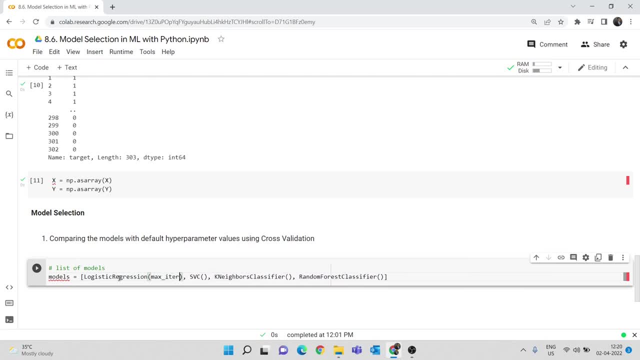 regression. i'm going to give this max hitter. so max hitter basically represents the maximum number of iteration and- and i'm going to give this- maximum iterations is equal to 1000 and support classifier doesn't work. if you just mention this svc, you have to mention at least one kernel value. 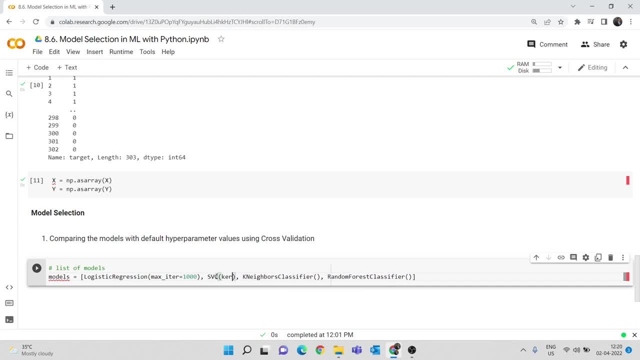 okay, otherwise it won't work. so i'm going to say kernel is equal to linear, so it is the most default to and the basic kernels that we have. so apart from this, we also have this, you know, polynomial kernels and other type of kernels. so kernel is equal to linear kernel for support, it to classifier, and then we have k nearest. 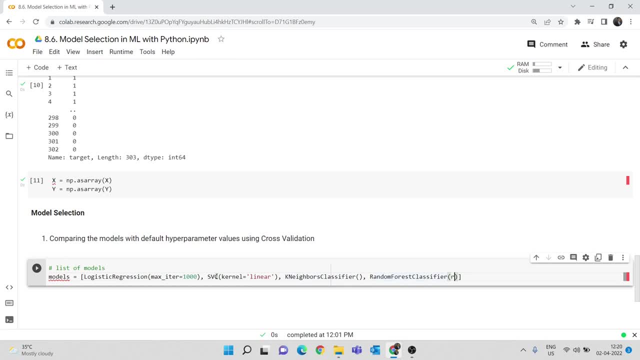 neighbor. so we don't have to give any parameters here and random for us we will set a random state. so if you don't include this random state, you will get slightly different accuracy score each time you run this. so i'm setting my random state. so if you give some, 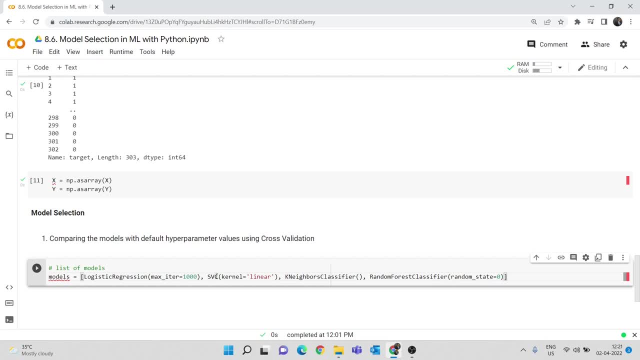 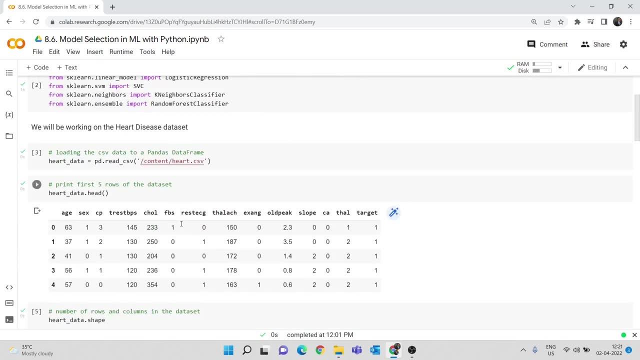 random state. your accuracy value will be the same if you train random forest less than multiple times. so that is the reason and the reason i'm giving this max heater is that we are not standardizing the data. in this case, as we can see we have, we are using. 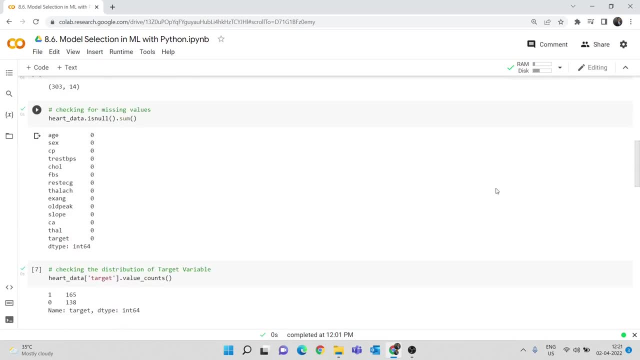 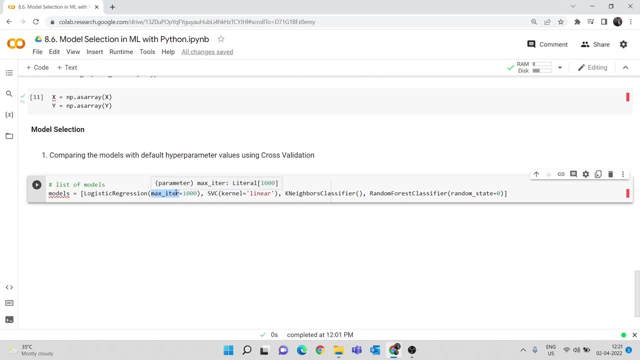 the data in this same format. so it will give us an error if we don't, you know, standardize the data before using it in logistic regression. so we are increasing this max heater, but the correct way would be will be, you know, in order to, will be to standardize the data, but we can't use it using 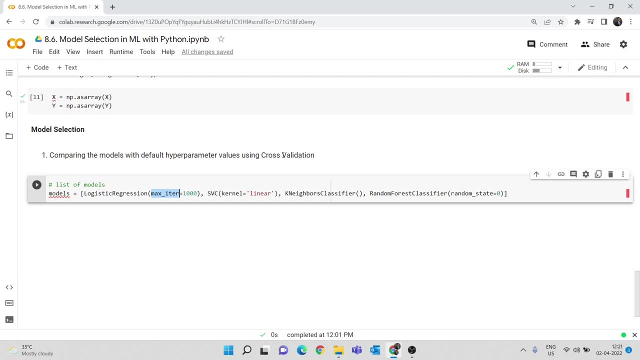 this cross validation directly. so we have to use something called as pipeline. so we have to build this pipelines and pass this- uh, you know, standard scalar and grid search, cv and so on. so it is a bit complex. we will discuss about that later, but for now, understand that we are using this maximum. 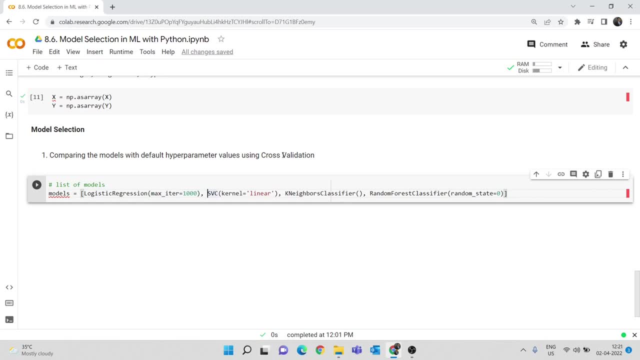 meter so that it doesn't give us any warning. so that's the reason, but we will discuss about this pipelines later on. so here i've created a list called this model and i have like four models here. first is the logistic regression model and the supported classifier model k-nears neighbor. 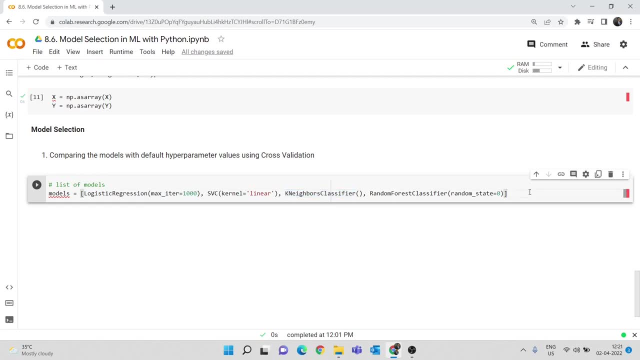 and random forest classified. so these are all the four models that i am considering, and now i'm going to create a function that will compare the accuracy score of these models. so, if you remember, we have already done this in our machine learning challenge, so i'll you know, take the same process and implement. 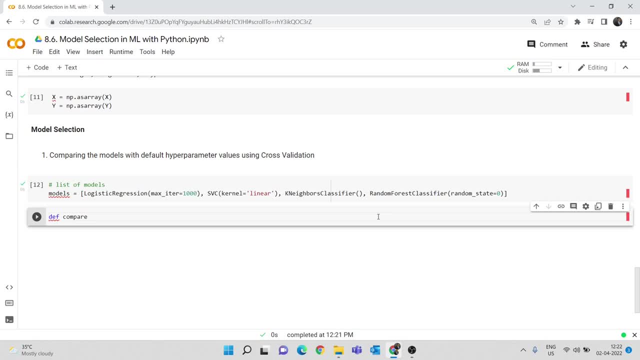 here. so i'm going to create a function called as compare models using the cross validation score. okay, compare models using cross validation. so this is the function that i'm creating. so you have to mention this parenthesis here, and here i'm going to. you know train models individually, so for this, 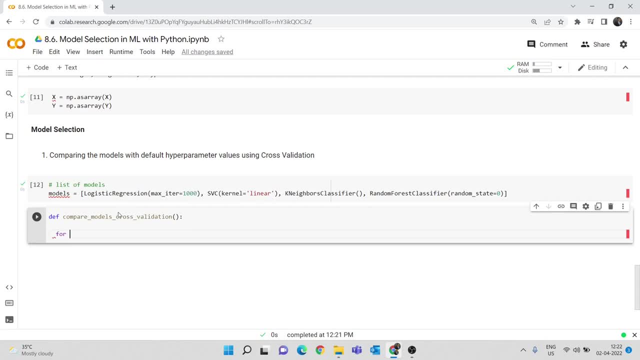 uh, i'll create a for loop. okay, for model in models. so i'm creating a for loop here. so when this, when we call this function, this for loop runs, and when this for loop runs for the first time, this model will take the value as logistic regression and it. 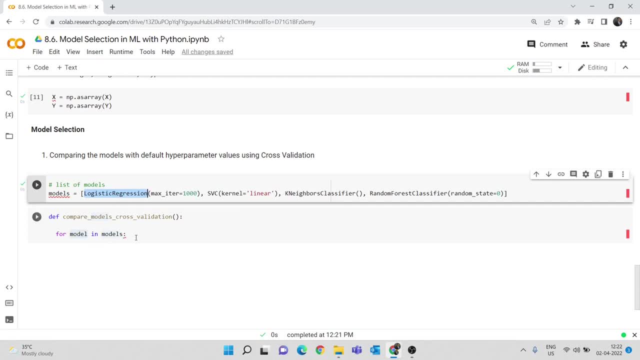 will you know, train uh with the given data set and it will print us the cross validation score. the second time the for loop runs, this model takes the value as supported classifier and so on. so this process kind of happens every time we run this. so for model in model, so i'm iterating this for 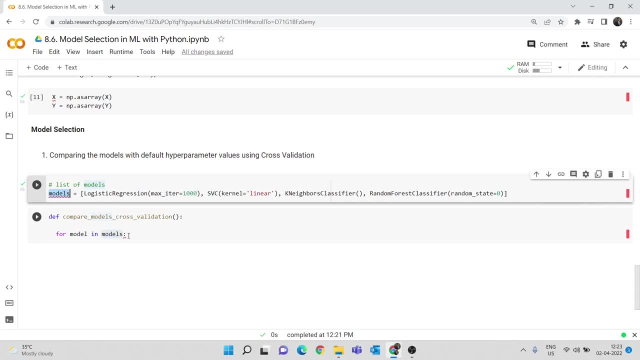 loop through this list called as models, and each time it will take one model at a time. so this is how it works. so for model in models, i'm going to say a cv score, so i'm creating a variable called the cv score, and now i'm going to use the cross val score function. okay, i'll copy this so. 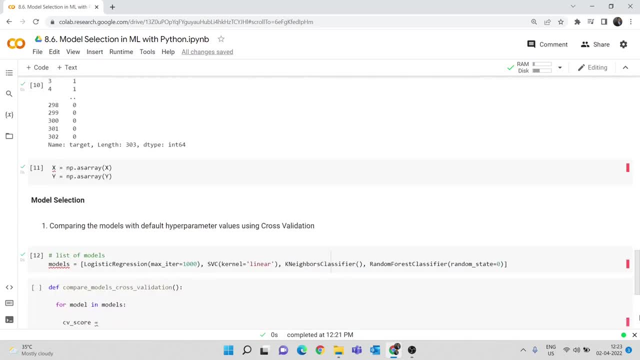 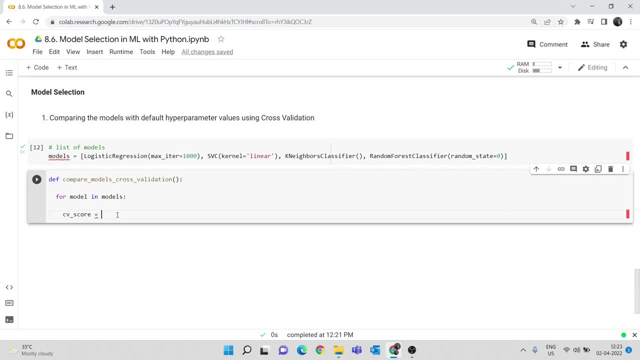 this crossbar score which are imported from model selection. cross validation score is nothing, but your data will be splitted into, you know, five holes and each time different data fold will be used as your training data and test data and if you don't know about this, i'll give the link. 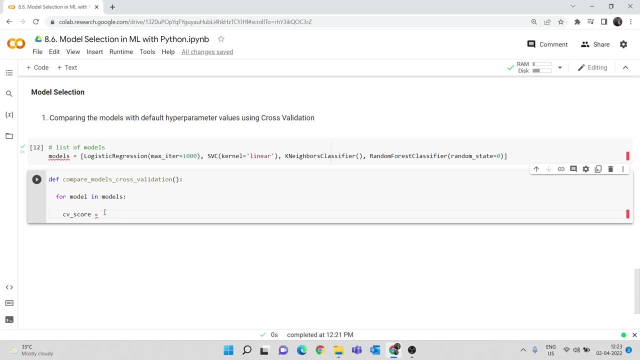 for this cross validation video. you can check that out and this is like very, very important. cross validation is one of the important topics that we have in machine learning. i'll you know, paste this cross value prospect score, a function that i imported, and here the parameters that we have to give are estimator, as you can see. so estimator is nothing but. 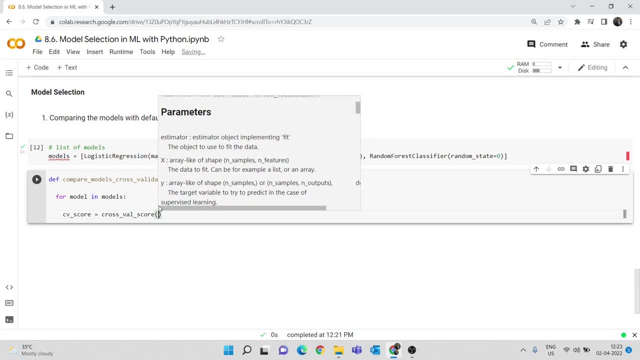 uh, the model that you are creating and the x is my features and y is my target. so I am going to say model: okay, so model x, y and a cv is equal to 5. okay, so the for loop runs for the first time. so this model will take the value as logistic regression of max hitter 1000 and it will go here. so we are. 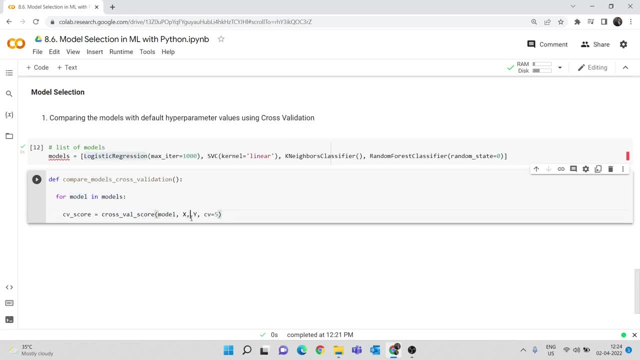 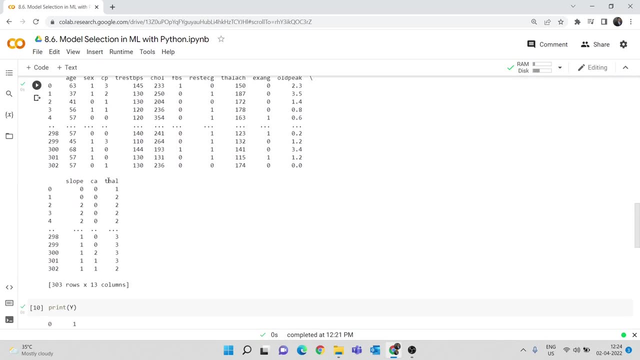 using this cross validation score function, so it will basically give you the cross validation score for logistic regression for this data. x and y, and x and y is nothing but my uh r disease data set that I have splitted into features and a target. okay, target is what you are going to. 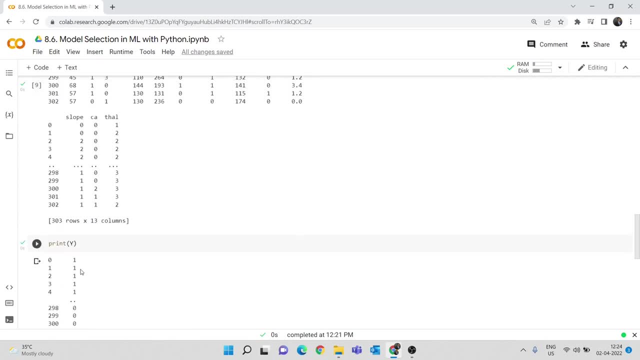 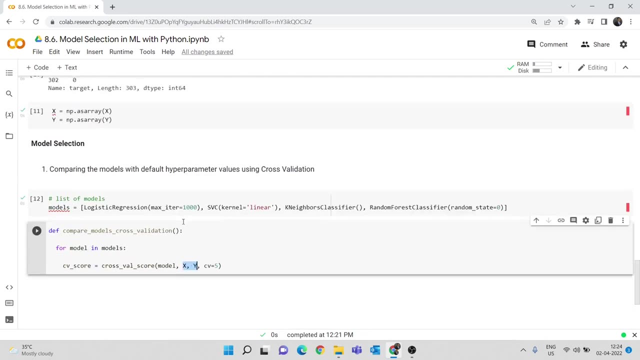 predict and feature is the values through which you are going to predict this target. okay, so here I am going to predict uh- whether a person is having uh r disease- using the factors like age six and so on. okay, so we have this cross validation score model x: y. cv is equal to 5. cv is equal to. 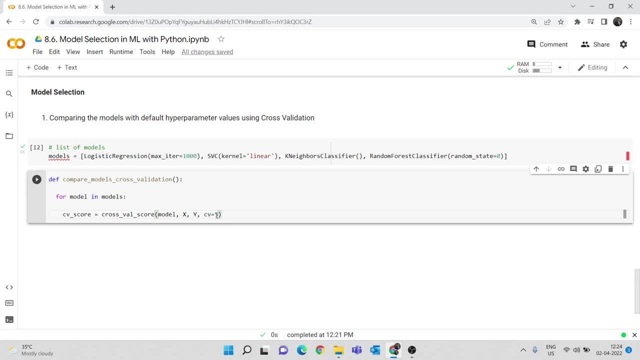 5 is nothing, but your data will be splitted into 5 folds, so you will be having like 5 chunks of data, and each time different chunk of data will be used as your test data set. so that is how this cross validation works, and you can also like change this CV. 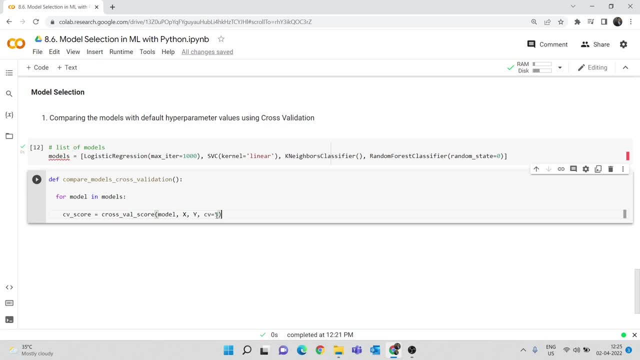 into three or five or some other values as well, depending upon your data set. so this CV score will basically give you five. you know accuracy score and from that five accuracy score we have to find the mean accuracy score. okay, so it also print this accuracy score if you want. 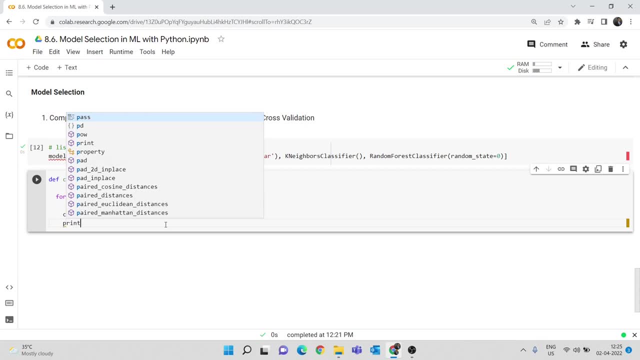 okay, so let's print that, but let's print that at a later point of time. so I'm going to say mean accuracy. mean accuracy is equal to sum of CV score divided by length of CV score. so this is how you can kind of find the average value of this cross validation score. I'll explain you later. 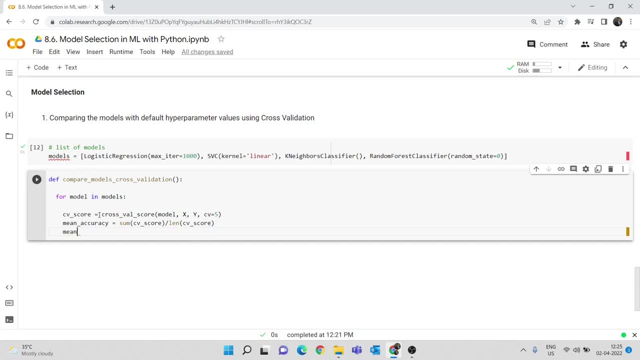 on how this you know particular code block works, and this mean accuracy is equal to accuracy into 100, and the next thing I wanted to do is I'll copy this mean accuracy test. it here is equal to round mean accuracy by two factor. now let's print this print. so just give me a minute, I'll explain you what we are. 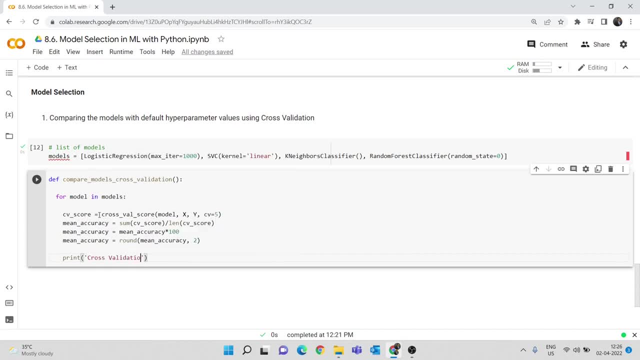 doing here. so let's print this print. so just give me a minute, I'll explain you what we are doing here. cross validation accuracy. accuracy for the model is equal to CV score. okay, so this is the first print statement, and next let's print our final accuracy. 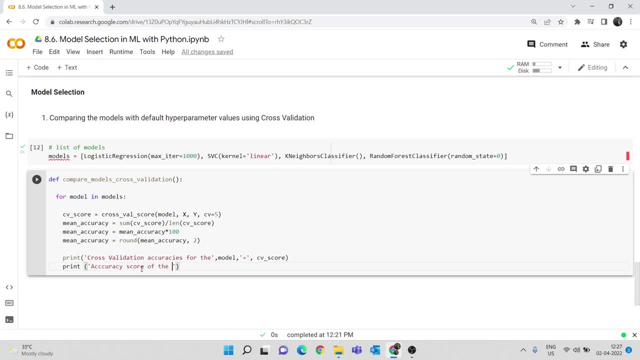 accuracy score of the model model is equal to my mean accuracy percentage is equal to my mean accuracy percentage. okay, let's run this one. so what we are basically doing here is let's say that the for loop is running for the first time, and when I say for model in models, 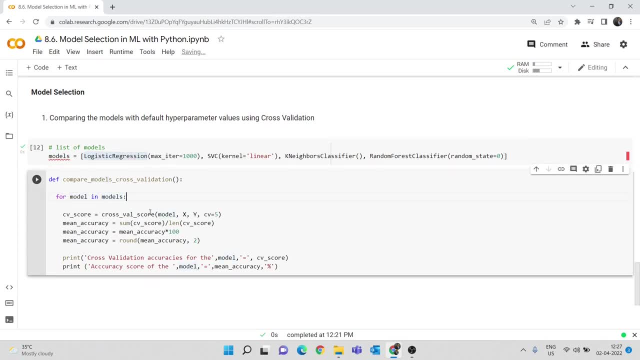 so it will take the logistic regression, as I've told you before now. I am passing this logistic regression model to this cross vag score function and I'm passing my data, which is my features and target, and I'm saying like I want five, five folds of data. so I am mentioning CV is equal to five. so what happens in this? 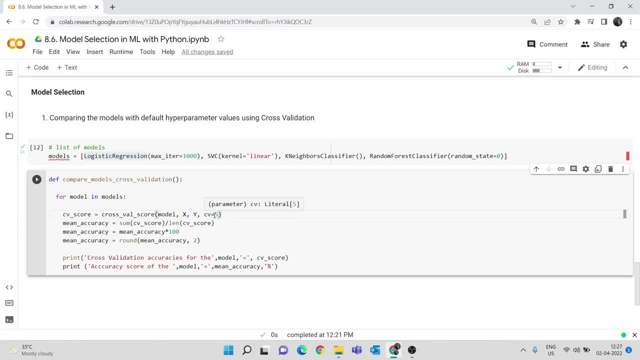 particular step is: your data will be splitted into five folds and your data will be trained using this logistic regression model. so this logistic regression model will be trained with the data that we have passed, and this will happen for five times. with each time there will be like different test. 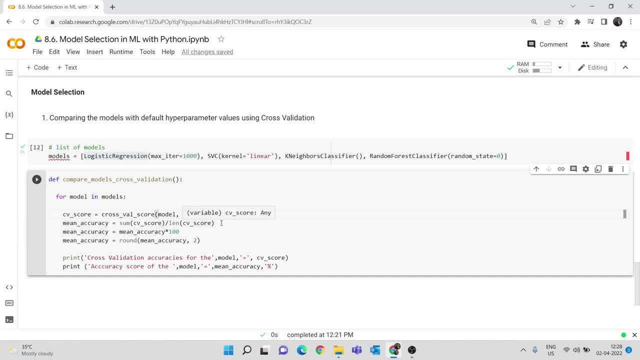 data because of this five folds that we are creating. so the result of this particular CV score line is that you will get like five accuracy values, so it will be in the form of a list. so from this five accuracy values, we are going to find what is the average of these five values. so that will be the final. 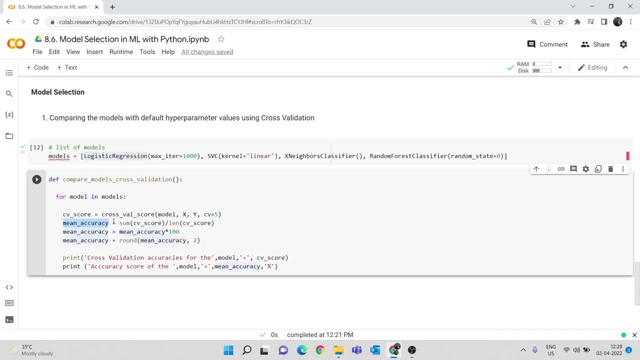 accuracy that we will consider. so for that only we are using this mean accuracy. so mean accuracy is equal to sum of CV score divided by length of CV score. so this is nothing. but we take like, let's say, that there are like five accuracies. one is like 80 percentage, another one is like 85 percentage, 83. 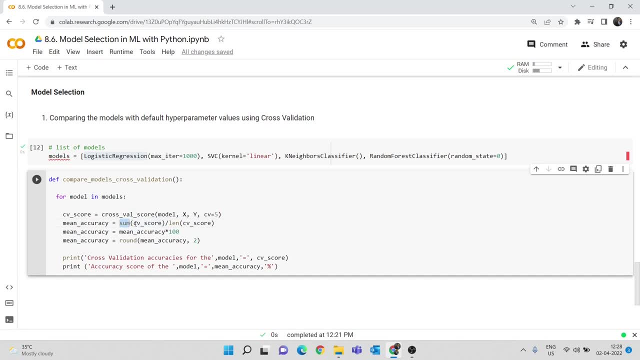 percentage and so on, and we are adding all those values and dividing it by the total number of values that we have. so in case like there are like five values, like 80, 85, 83, 84 and 83, so we will add all those values and divide it by 5. 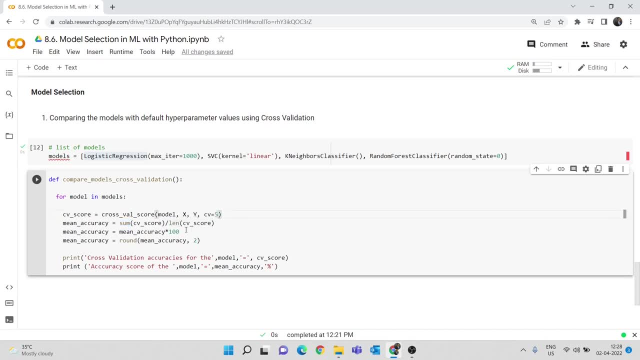 because there are like five accuracy values. if you increase the cross validation fold, you have to. you know this will change us when the length of CV score changes as well. and now we are calculating the mean accuracy. so here I am multiplying the mean accuracy by 100, because the value 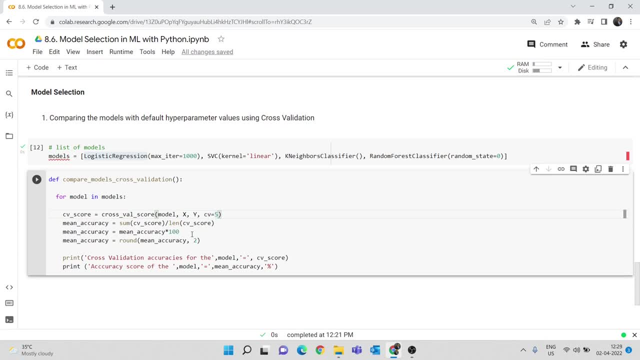 will be in the range of 0.9. so if a model has 90 percentage accuracy, it will be represented as 0.90. if model has 85 percentage accuracy, it won't be given as 85, it will be a printing as 0.85. so we are multiplying it with 100 in order to 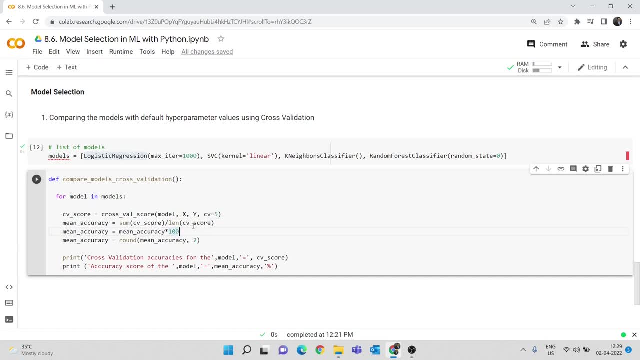 convert it to a percentage. so this is just simple percentage conversion and this step- mean accuracy, sum by length- is for calculating the average, this is for converting it to percentage and I'm going to say: mean accuracy is equal to round of mean accuracy, comma 2, and the reason we are using this. 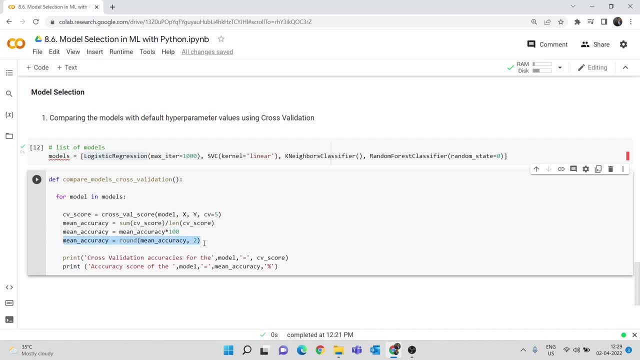 particular step is there will be like several decimal point values. so I'm going to say I want only like two values after the decimal points. I'm saying like round, I'm going to round this mean accuracy value and they want only like two decimal places. you can also give like three, four, depending on how many. 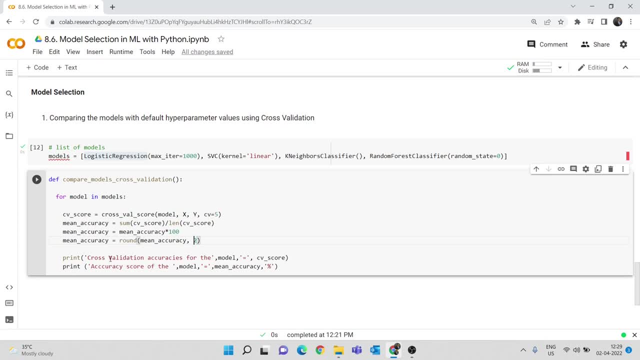 values that you want. and finally, I am printing my cross validation score. so I am going to say cross validation accuracies for the model. So this is my variable that I have created here. So this follow prints for the first time it will print cross validation accuracy for the. 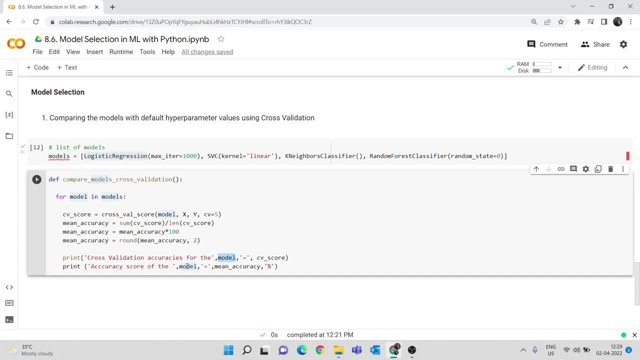 logistic regression is equal to some cross validation values and again, so this is not in the string, so we have not enclosed this in quotes, So this is actually a variable that we have created. So here it will say: accuracy score of the logistic regression model is equal to the. 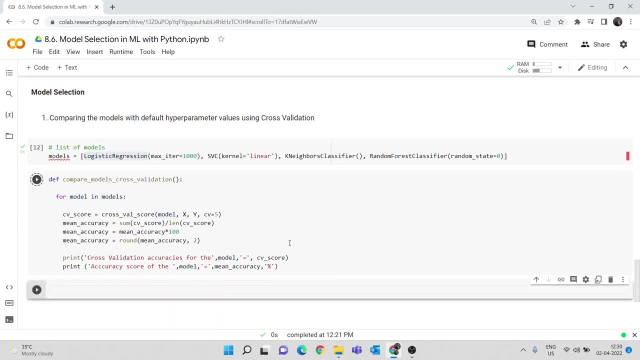 mean accuracy and so on. So let's run this step and see whether this works. Okay, so we have created this function. now we have to call this function. So I will copy this and I will run this one, So this will print me these results. okay, let's see. 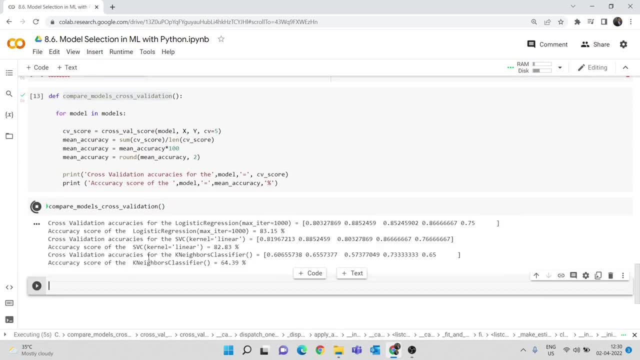 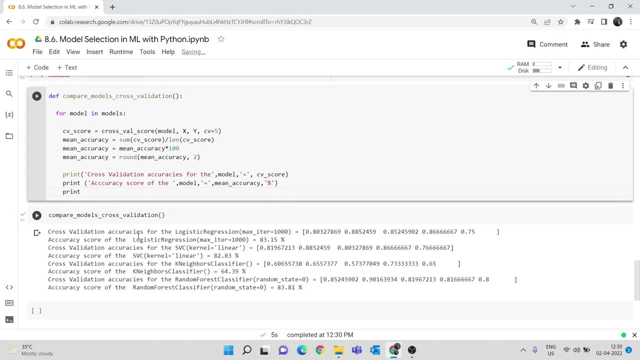 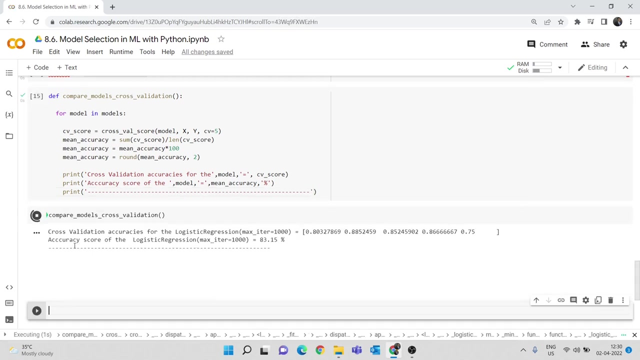 So all the splitting of data will happen inside this, okay, so let me just add one more line to it so that this results are kind of splitter. I am going to say print. I will just print some dotted lines here, okay, So I will. I will run this again now, so the result will be the same. so we just have this dotted line. 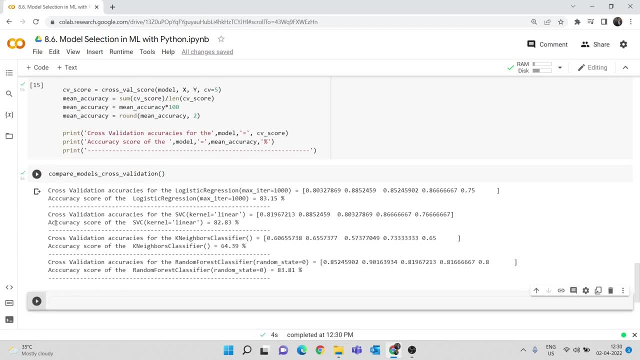 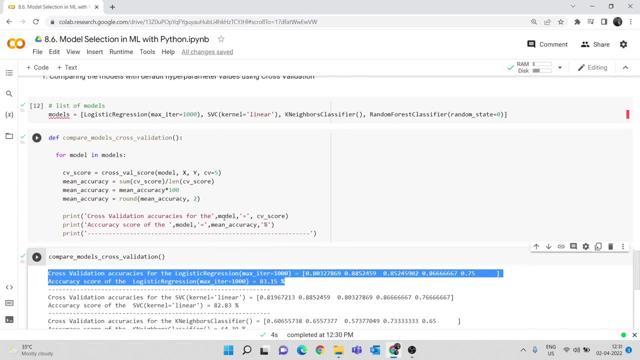 in between. okay, So, as you can see, this is the result when the follow prints for the first time. so it will take the value for this model as logistic regression, So that is what is replaced here as well. so cross validation accuracy is for logistic regression, as you can see. 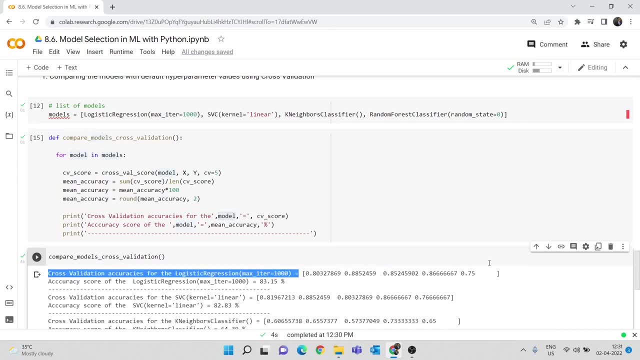 So cross validation accuracy for the logistic regression is equal to these five values. okay, So for the first fold of data, we are getting the accuracy as 0.80, which is 80.3%, this is 85.3%, and so on. 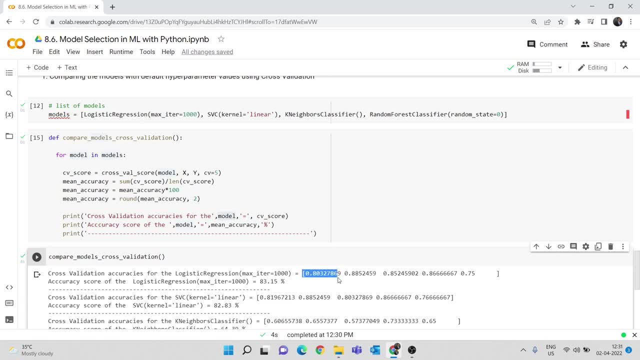 As you can see, there is a clear difference between them. so we have like accuracy score in the range of 80. we also have accuracy score as 75%, and so on. So this is why cross validation score is always preferable instead of trained test spread. 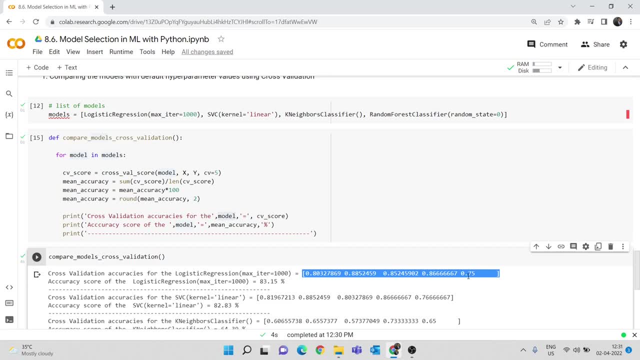 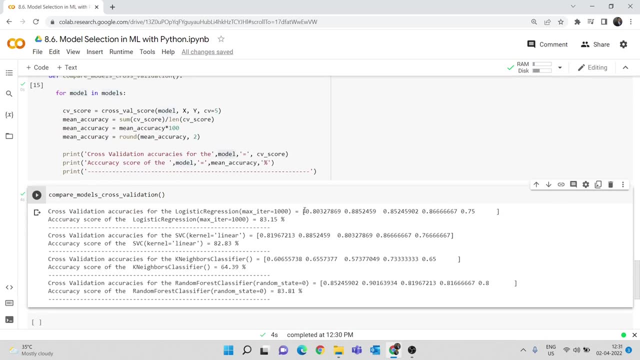 because trained test spread will give you like only one accuracy score, but this is like more reliable as we have like multiple accuracy score and we are taking an average of it, and the average of all these five values are this: 83.5. so that is what we are doing in this. 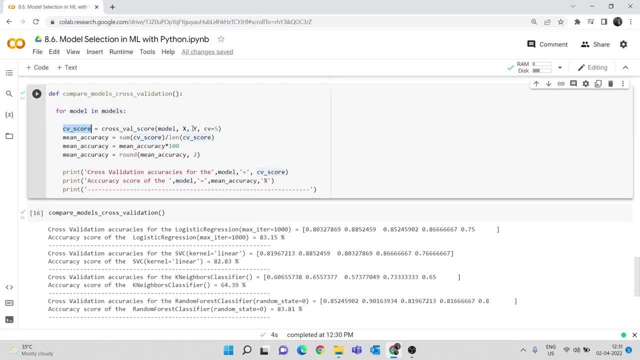 particular step. So when I say CV score is equal to crossvalve score of model xy, CV is equal to 5. this is the result that I get from this particular line. so this is the. so this is the value of this CV score. so these five values are the value of this CV score, and I am adding all these values. 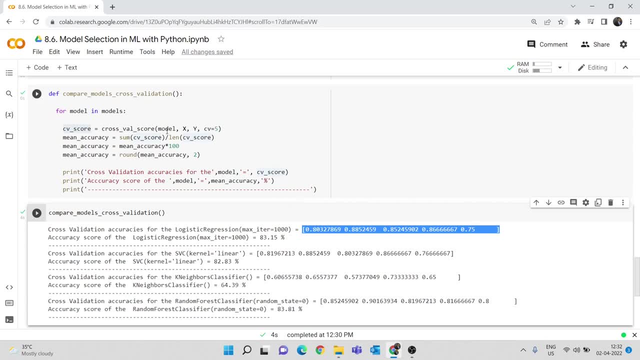 using the sum of CV score, dividing it by total number of values, which is equal to 5, and then I am multiplying this value by 100 and I am reducing the decimal places. as you can see, there are several decimal places and I am reducing the decimal places- is equal to 2. 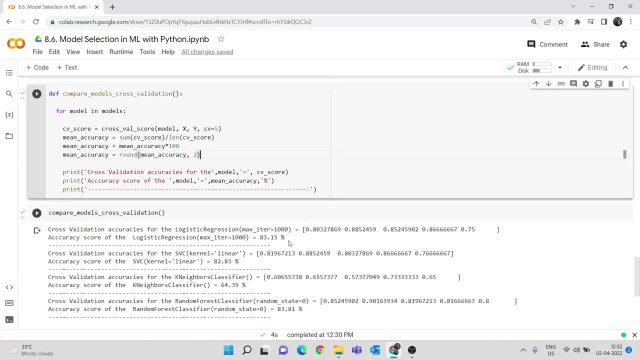 so this is how we are converting this value from 0.80, or whatever we have, to this particular percentage value, which is 83.15 percentage. so we have two decimal places here because we have two here. so if you, you know, replace this two with three, you will get three decimal places. so it is completely up to you. 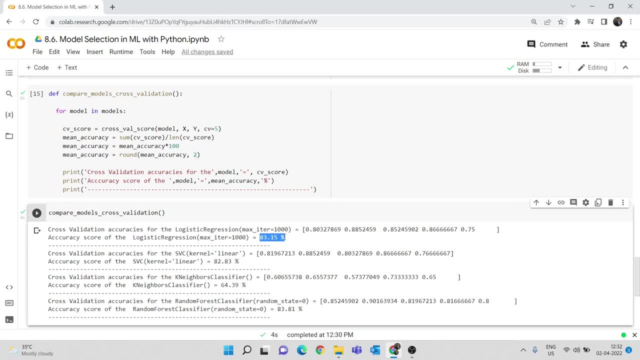 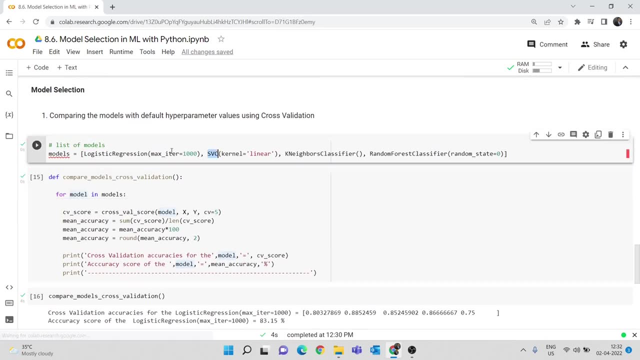 it will round the values. so this is the final value for this logistic regression cross validation and once this for loop runs for the second time, this model will take the value of this SVC, which is my second element of my list called as models. so this is the cross validation. 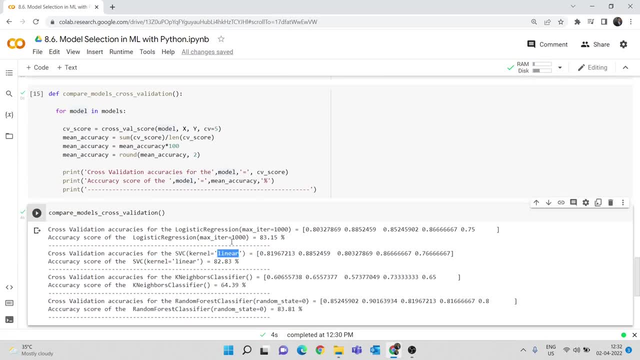 score of support vector. machine classifier with linear kernel. so these are like some of the basic hyper parameters we choose for these models and this is the value. and then we have the average of these values is like 82.83 percentage. so this is the cross validation average value. 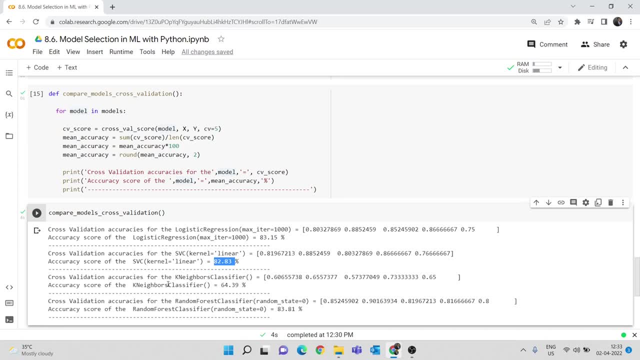 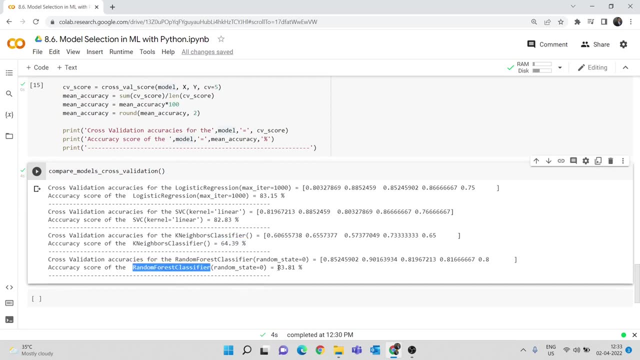 for logistic regression. this is for support vector classifier- and finally, as we can see, k nearest neighbor as 64.39, which is very less, and then we have the like accuracy score for random forest classifier as 83.81. so this is how you can. 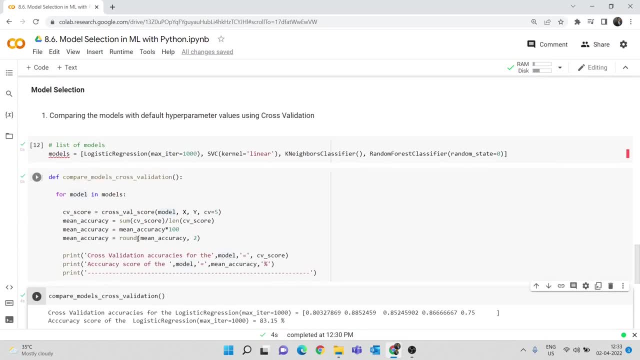 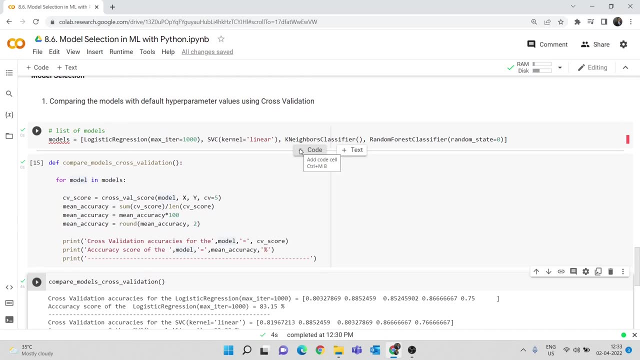 compare the accuracy score of different models using this particular simple function. so you don't need to train your model separately in order to do this. you can just create a list with all the models that you want to compare and you can just build a simple for loop like this and you will get. 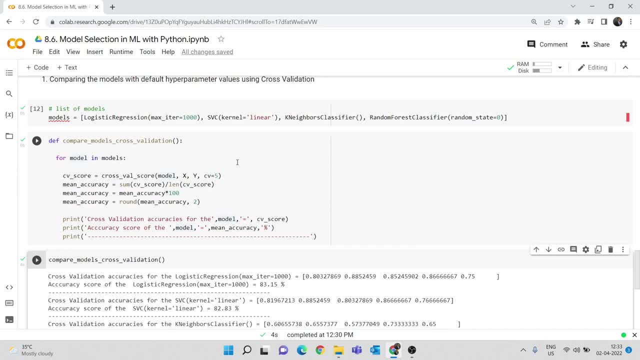 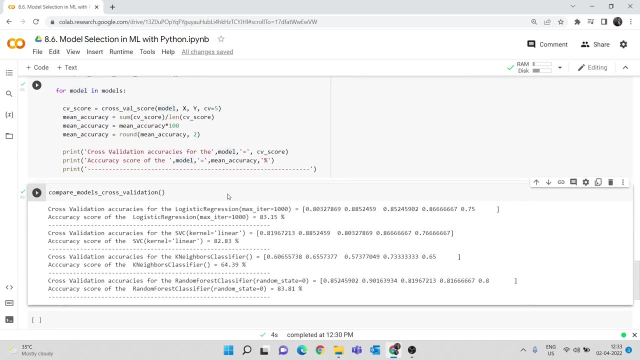 a result like this, so you can save this code as a template and you can use this for any other use cases that you are working on. so this kind of saves a lot of time and this is a pretty good way of doing this model selection. and the thing is here we are doing this with the default hyper. 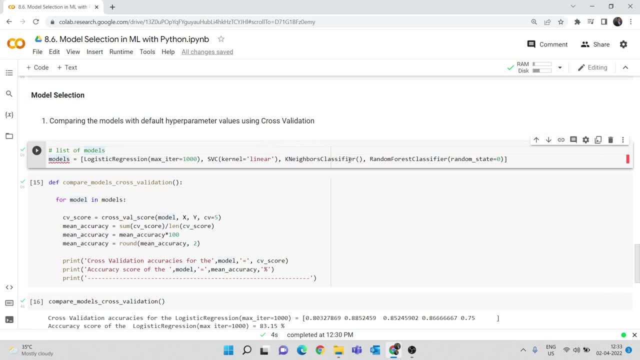 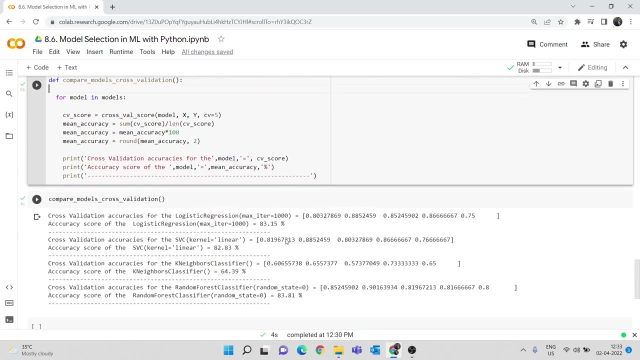 parameter values which we are having. so we are not doing any hyper parameter tuning on all those things. we will do that in the next part of this video. okay, so we have the list of models and we are comparing this model. so within this we have to see which model has the highest accuracy. so it is obvious that logistic 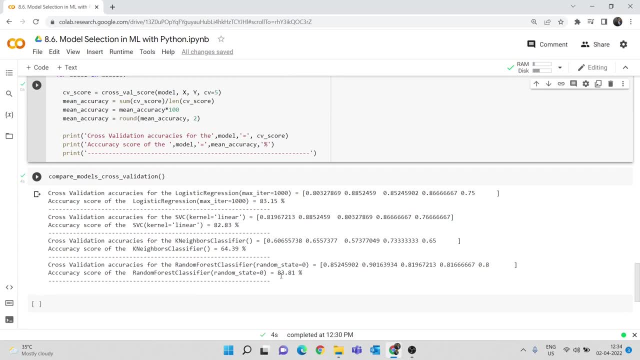 regression and k nearest- sorry, logistic regression and random forest classifier as the highest accuracies and among this random forest classifier as the highest accuracies, as we can see, which is 83.81 percentage. so this is like very close to logistic regression as well and k nearest neighbor. 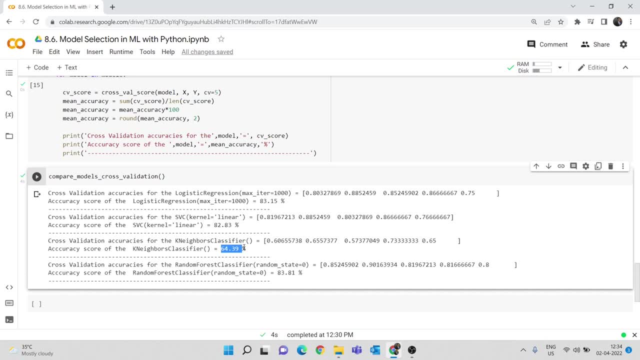 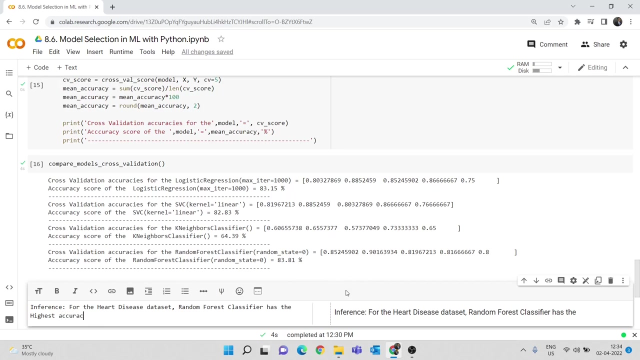 accuracy, which is like 64 percentage. so here i'll create an inference. okay, let me put this as inference. as for this particular art, this is dataset for the art, disease dataset, random forest classifier, the highest accuracy value. okay, so as the highest accuracy value with default hyper parameter. so we are not changing any of the hyper parameter values yet. 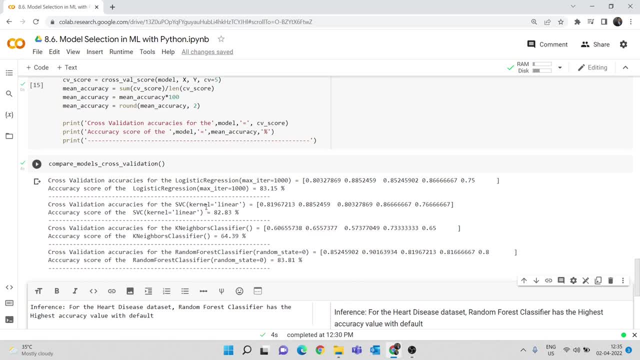 except for this maximum meter in logistic regression alone. so kernel is linear, is like we have to give at least one kernel value, so that's why we are giving it so with default hyper parameter values. okay, so let me put this random forest classifier in bold letters. okay, so this is, uh, the influence that we are getting and the important. 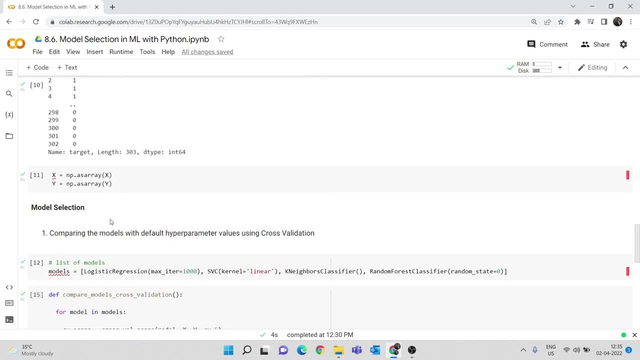 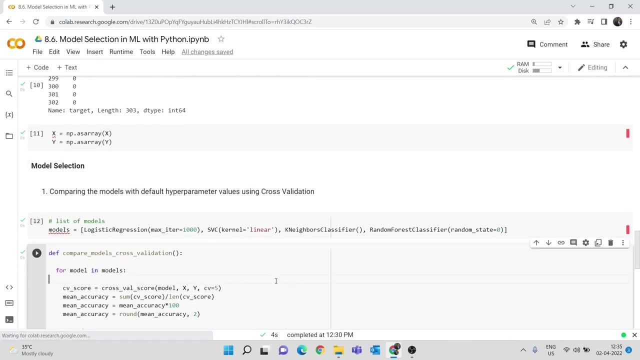 thing that we have to note here is we are not doing any hyper parameter tuning. so this is what i have mentioned here as comparing the models with the default hyper parameter. we is using cross validation because we have used this cross well score, and now what we are going to do here is we 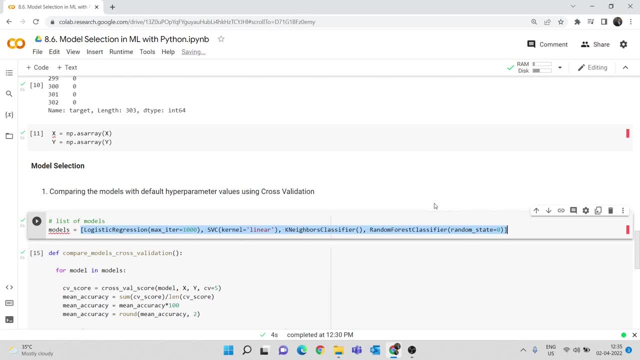 will take all these four models and we will check this models, for you know, different accuracy score for different hyper parameter values. okay, so it's like doing hyper parameter tuning as well as model selection together. okay, so this is the next part of the code and, uh, you know, this is again interesting thing, uh, that we have. so let's see how we can do this. 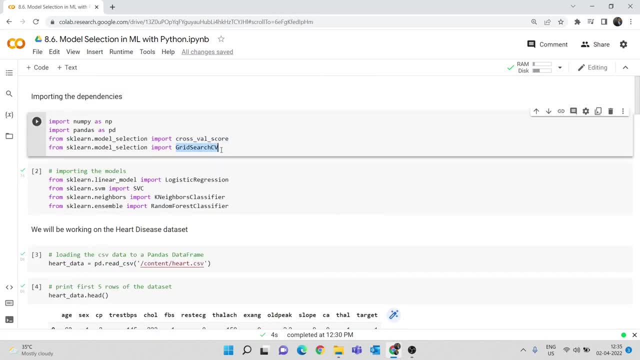 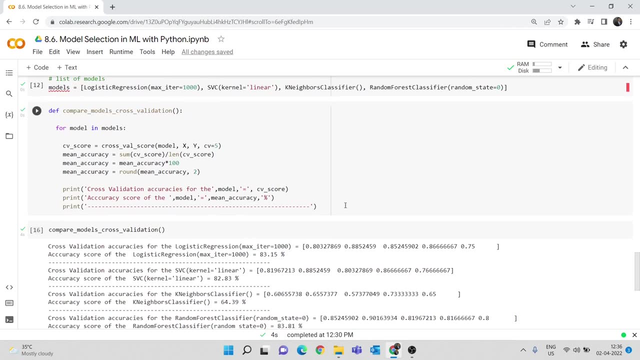 so in this case, uh, instead of this cross validation score, we will be using this grid: set cv, as we have to, you know, do this hyper parameter tuning as well. okay, so in case, this is like enough for you. so in case, like you don't have to do any hyper parameter tuning, you just wanted to compare the models with. 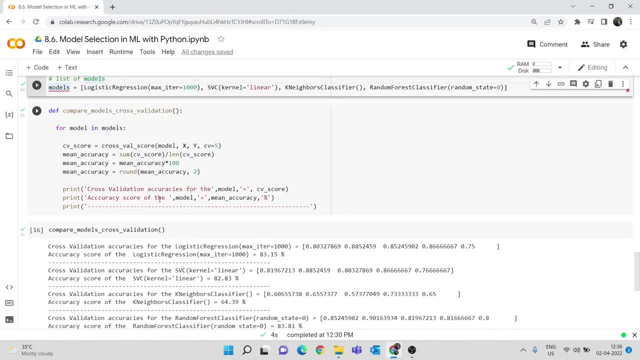 default hyper parameter values alone. in this case, you can use this particular code snippet and after this, what you have to do here is like: you have this x and y right, so you have to split this uh, x and y into training data and test data. so we have already discussed about this, so you can also 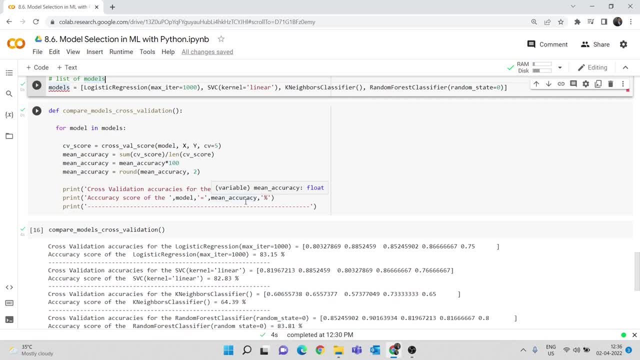 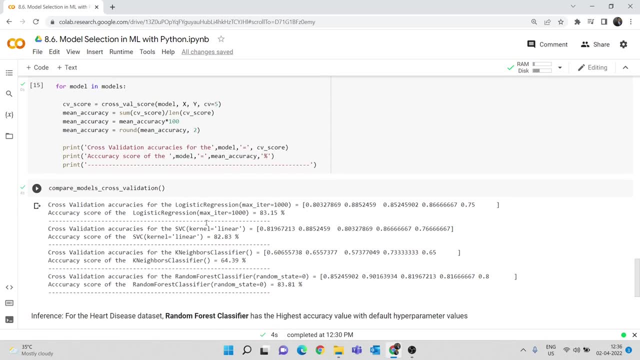 refer my R-distance prediction project video in order to understand how we can perform this train test, split, train the model and so on. so, after splitting the data into training data and test data, you can, instead of like using logistic regression on spc, you can use this random forest. 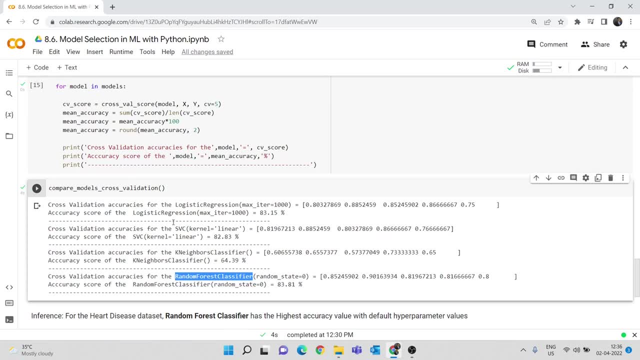 classifier. so this step is just to you know, understand which model has the highest accuracy, and you, we cannot like use this any mean. we cannot use this further. so this is just for comparing the model. so once you do this, you can train your- uh, you know- random forest classifier after splitting the data into 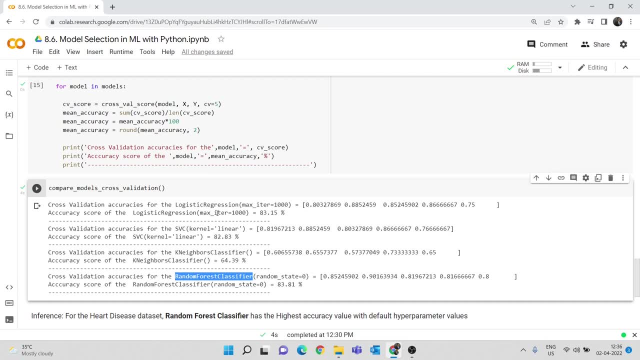 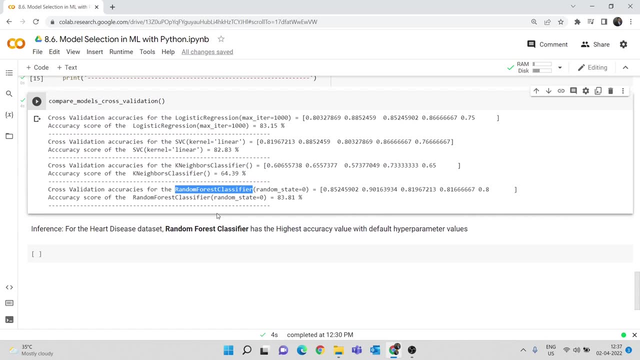 training data and test data. so that will be the next thing that you have to do. so i'm not covering that train test split, as we have done that several times before. so once you perform this cross validation, you have to split your data to training data and test data and train the model. do the 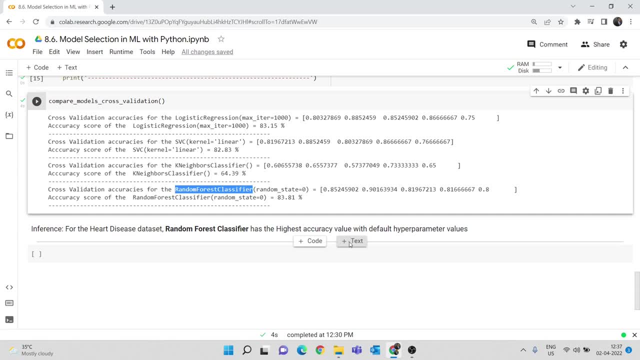 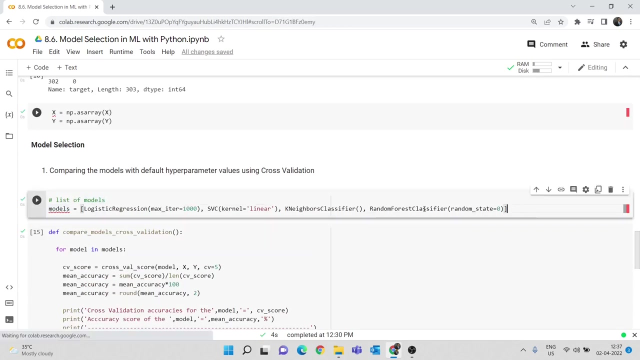 model evaluation and all those things, and the second part of the code that we are going to do here is is comparing the models with different, different hyper parameter values using grid search cv. so okay, now let's create another list. so it is again the same list, but 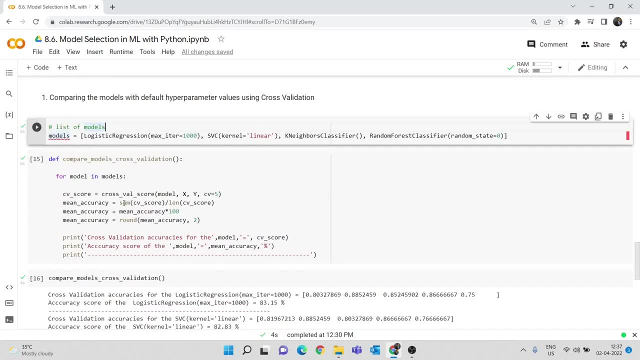 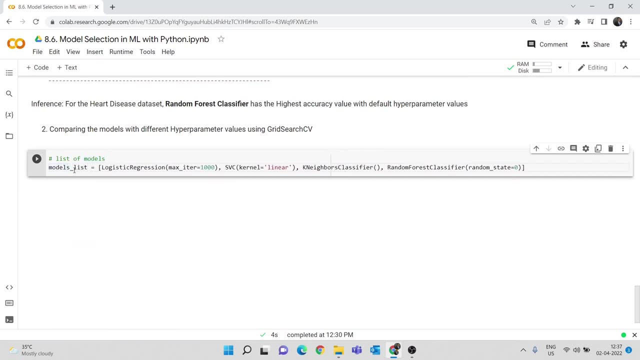 i'm just i'll just copy this and create a new name for this. you can have the same same name, but i'm just creating a new one, so let's call this as models list. so models list and logistic regression. i'll just change the uh maximum meter to ten thousand. so if 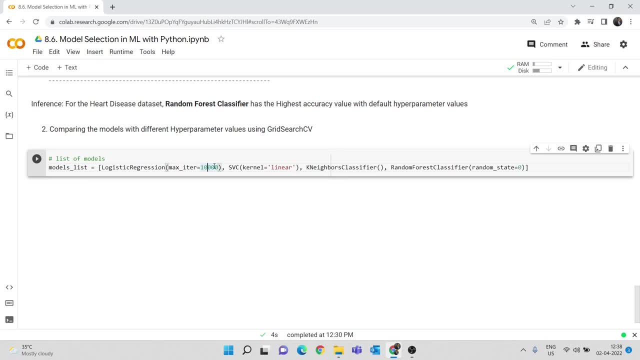 i just use this thousand. it is giving me some warning, so that's why i'm using this maximum meter. but the correct way of doing this will be to standardize the data and do all these things again. for that we need pipelines. so let's not go in detail about that. let's change. 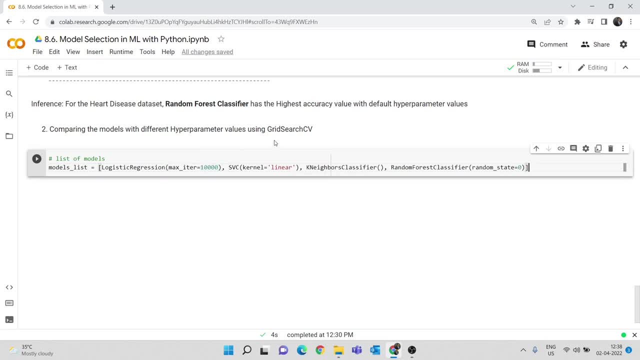 this maximum meter value alone. okay, and uh, then i'll just uh, remove this. kernel is equal to linear. okay, because that's what we are going to check here. so we'll be checking the supported classifier for different hyper parameter values, like different kernel values, so we have different. 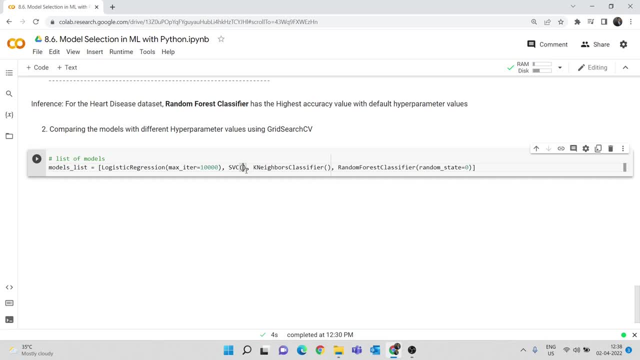 kernels like linear, poly, rbf, sigmoid, etc. so we will be comparing all those things as well. okay, so, okay. so we have created a list of models. first is logistic regression with the maximum iteration, support classifier, k, nearest neighbors and random forest classifier, so you can also change this random state. 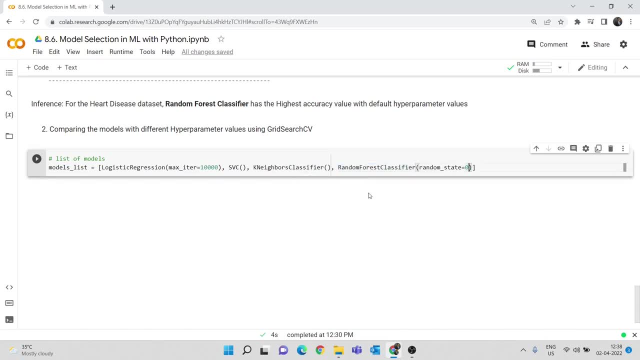 uh value, if you want, but please include this so that we don't get different results each time we run this code. so now the next thing that we have to do here is so here we have created a list that contains the name of all the models that we are going to use the logistic regression classifier. 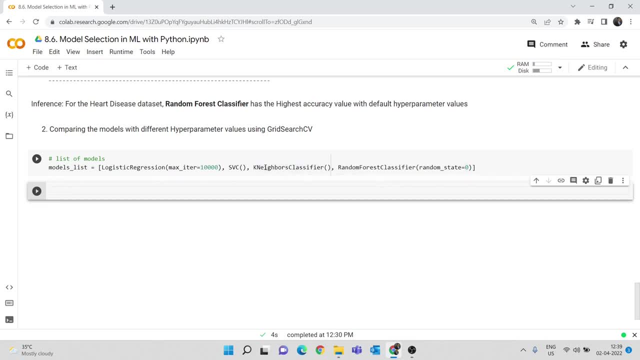 spc, etc. now we have to create a dictionary that has all the hyper parameter values, so that is the next important thing. so here we are creating- okay, so creating a dictionary that contains hyper parameter values for the above mentioned models. okay, so let's name this dictionary as: 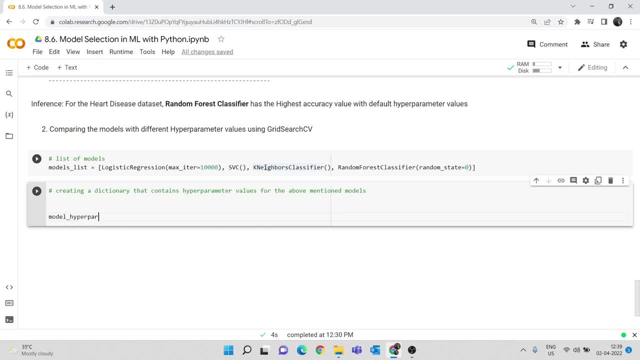 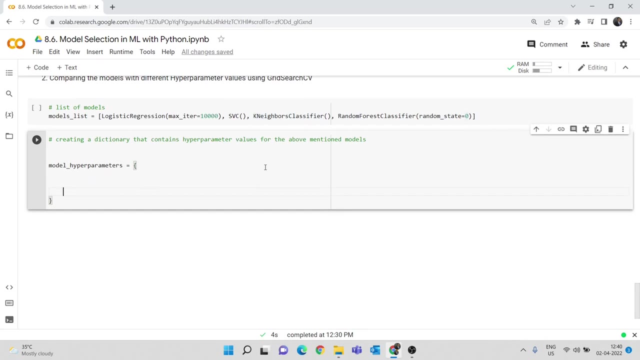 model hyperparameters. okay, so this model hyperparameters is equal to: as we know, we have to enclose the values of a dictionary in curly brackets. so i'll create this: curly brackets. and so we know that a dictionary is a key value pair, so it contains a key and some set of values. right? so the first key that i'm going to. 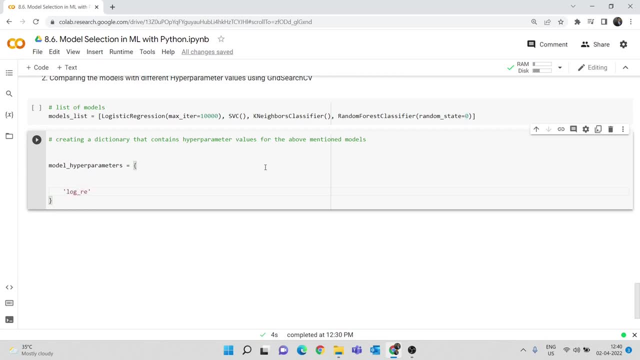 create is logistic regression. so logistic regression- i'll just mention this in short form. so logistic regression, hyperparameters- okay, So this is the first key that we have, and here we are creating another dictionary. okay, So I am going to say logistic regression, hyper parameters is C colon. I will explain. 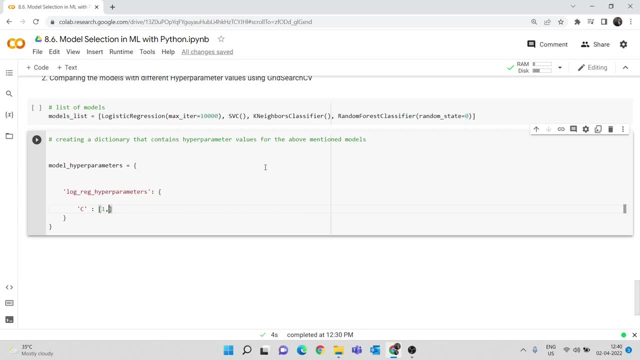 you what we are doing here. So this may seem a bit complex, but this is actually very simple. let me just complete this and explain you. So here you have to mention what are all the different hyper parameters that we want to consider. So here for logistic regression. 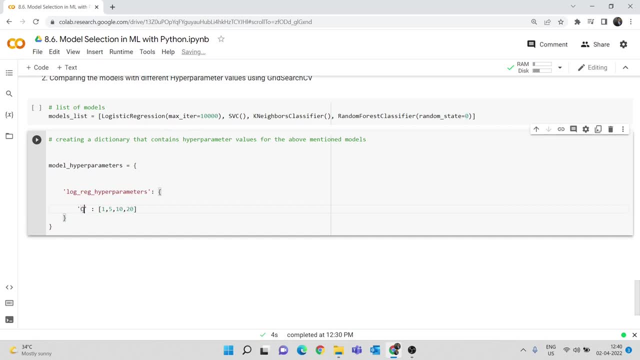 model, I am going to change the different hyper parameter for the C value. okay, So that is what I am mentioning here. So C can take values like 1,, 5,, 10 or 20, and so this is my first thing and there should be a comma here. So this is my first set of values, and 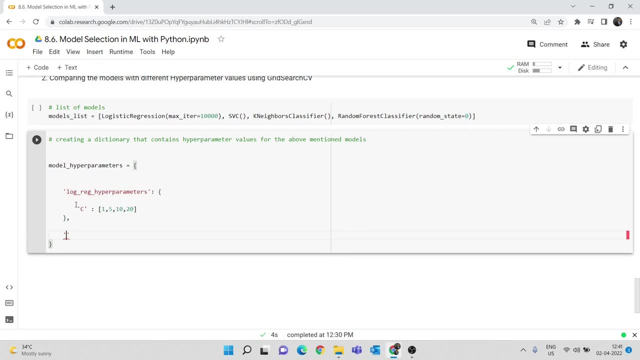 the next model that I am considering is support vector classifier. right, So it will be SVC, support vector classifier hyper parameter. So SVC hyper parameters. So again, we have to create another dictionary within this. and those values are two things. one is kernel, and for kernel I am going to consider different. 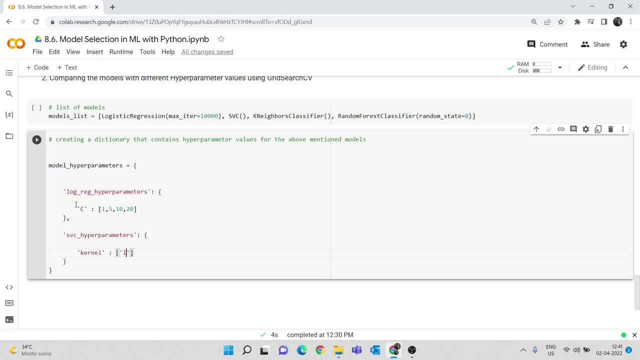 kernels like linear kernel, polynomial kernel, which is represented as poly, and RBF. So we have discussed about this. different types of kernel: So we have discussed about the different types of kernels in our support vector classifier video So we can check. 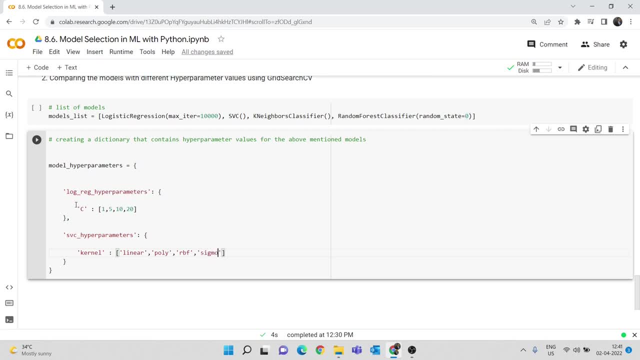 that out, So it will be in the seventh module of our course. and then sigmoid kernel. So these are all the four kernels that we have: linear, poly, RBF and sigmoid. And finally, let us also change the C values. So for C values, again I am going to say 1,, 5,, 10 and 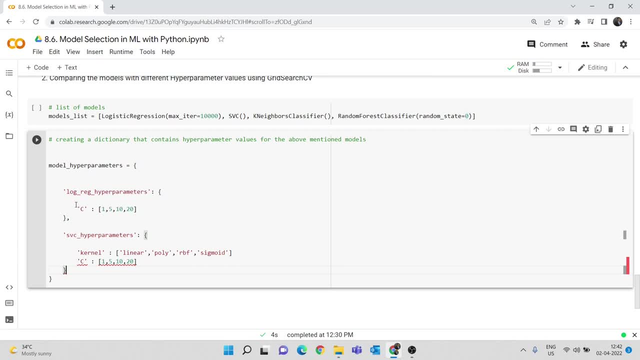 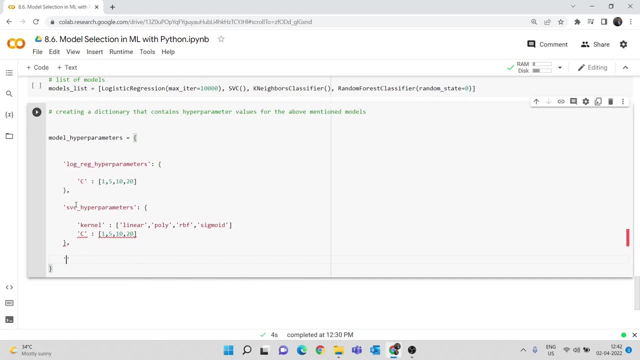 20.. So these are the different C values that I am considering. So another comma here. and the third model that we have is k near Amplified neighbor, right. so for k nearest neighbor i'll mention this as knm hyper parameters. so we have also discussed about this k nearest neighbors as well. so it kind of 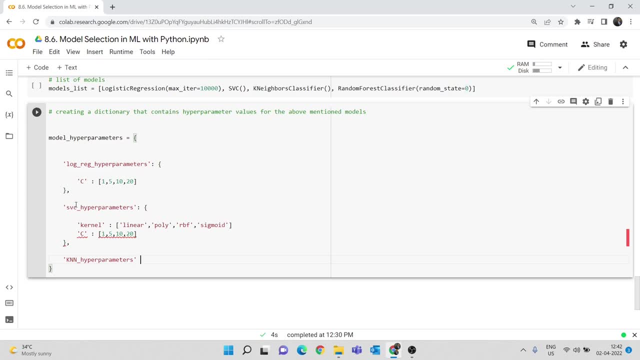 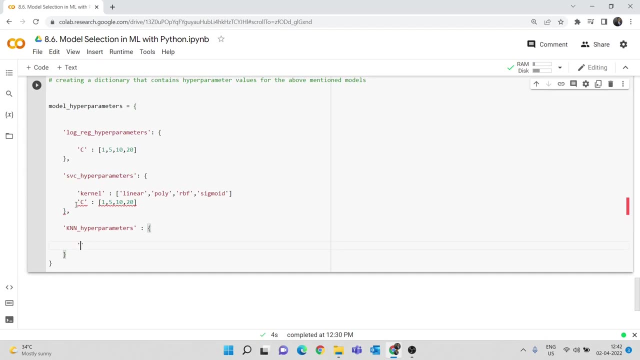 checks how many nearest neighbors are there to a particular data point in order to determine its labels. so, knm, hyper parameters, and in this case, the hyper parameter that we are going to consider is n, neighbors. so, yeah, neighbors, okay. so, if you are not sure how i am, uh, you know doing. 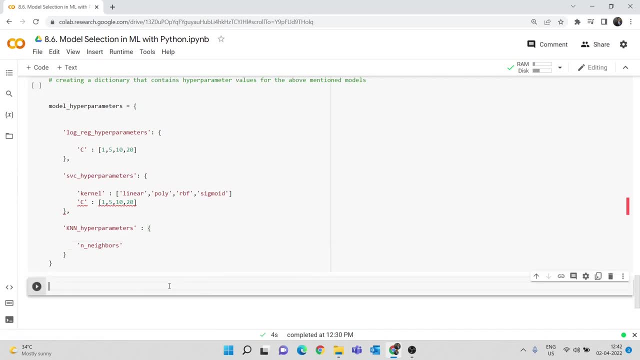 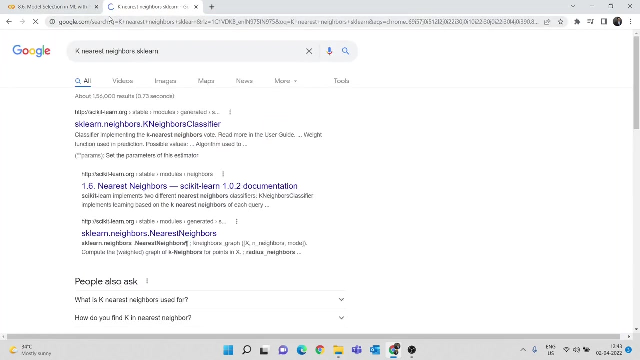 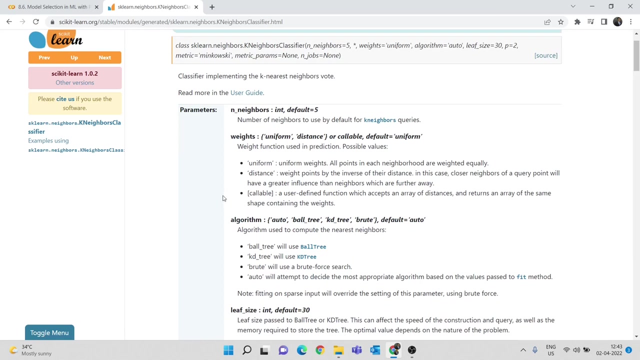 this c kernel and n neighbors is, if you, you can just search it. so i'll say: you know k nearest neighbor, um, let me just search this in google. so this will take us to the documentation of this k nearest neighbor classifier we can see. so these are all the different uh hyper parameters that you, that we have. 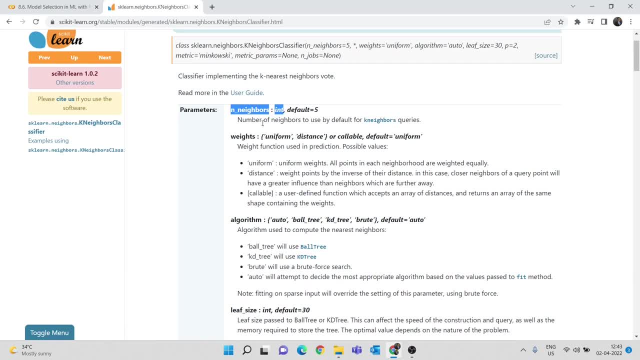 and n neighbors is basically the number of neighbors uh, that we, you know, we consider for determining a particular data point. so if you don't understand this, you have to watch my k nearest neighbor intuition video. so basically, k nearest neighbor works, is, let's say that there. 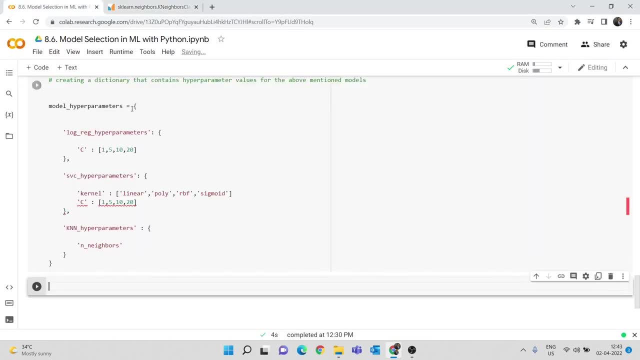 are like two groups of values. so here we have like uh data with labels as one and zero right. similarly, when we are training this model and and predicting a new value, this knn model will say: uh, this particular new value that you are predicting is closer to which group of data, whether it is 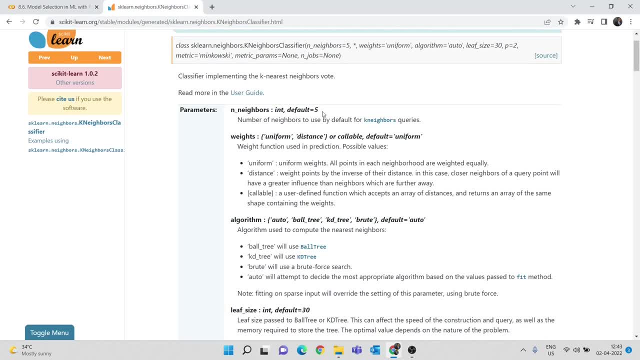 close to one or it is closer to zero. so when you say five, it will like: consider the five nearest data points to it and uh, it will say like which, uh data points are maximum. okay, so if you want a- you know detailed explanation on this. please watch the k nearest neighbor uh video that. 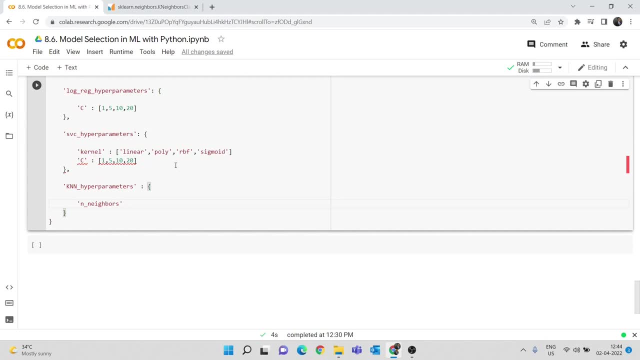 that i have created. so in this case, the default value is five and now i'm going to consider, like different values for it. so i'm going to check for different values, such as: uh, three neighbors, five, nine, five neighbors and ten neighbors. okay, and this will be, this will be. 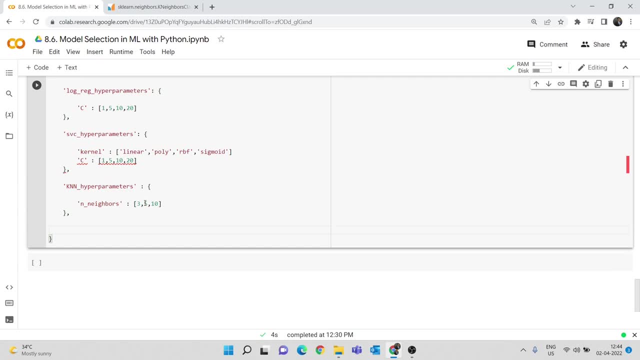 the hyper parameters for my third model. and finally, we have the random forest classifier and i'll create the key as. let me just include another space here. okay, so this will be random forest classifier. okay, so this is my. okay, let me just put this as random forest hyper parameters. 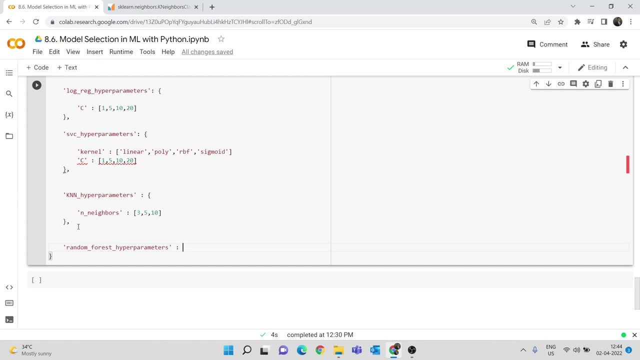 okay, hyper parameters. and here the hyper parameter that we have to consider is my n estimators. n estimated, this n estimator is equal to 10, 20 and 100. okay, so this n estimator is nothing but the number of decision trees that you need. so we know that we have a machine learning model called as decision tree, where it kind of build: 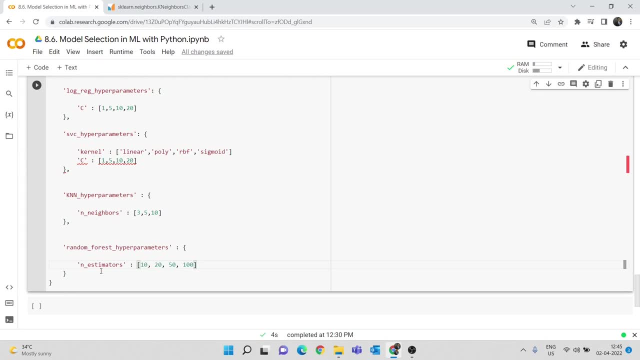 this tree and so on. what meant, what is meant by this random forest classifier, is that this model contains multiple decision trees. so that is how this random forest classifier has been built, and this n estimator kind of tells it like how many decision trees should be there in this random. 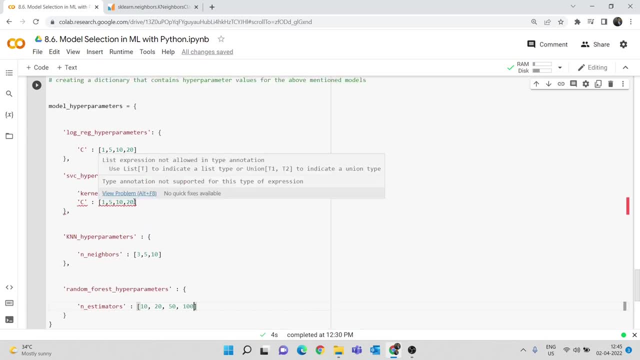 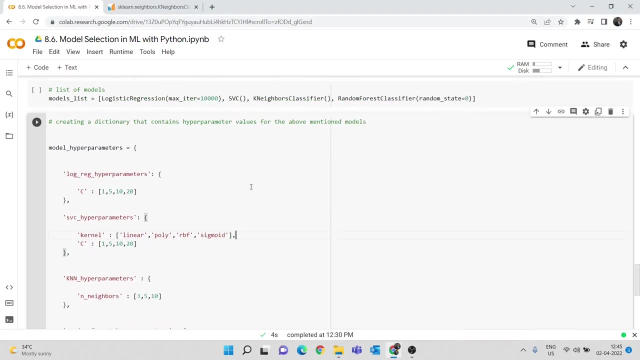 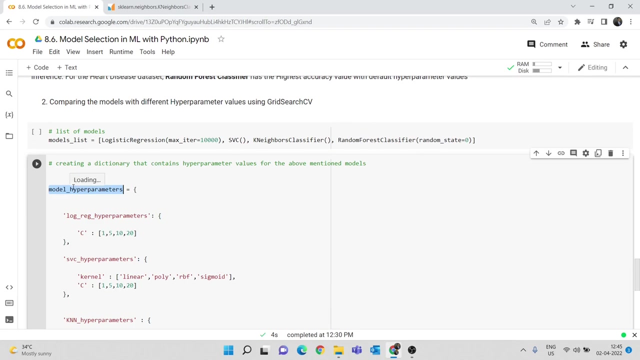 forest model and so on. so this is how this works and yeah, okay. so there should be a comma in this place, just a second, okay. so let's try to understand what we are exactly trying to do here. so here i'm creating a dictionary called as model hyper parameters. so what is this dictionary, is it? 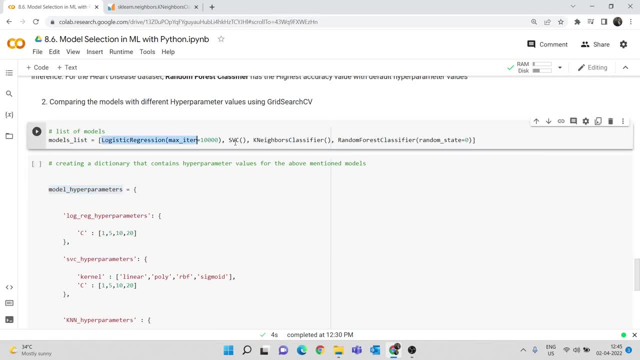 contains the different hyper parameter values for all the models that we have listed here. okay, so that is the idea of this, and so this is a dictionary and we are creating another dictionary within this. so we know that a dictionary is a key value pair, so there will be a key and a set of values to it. 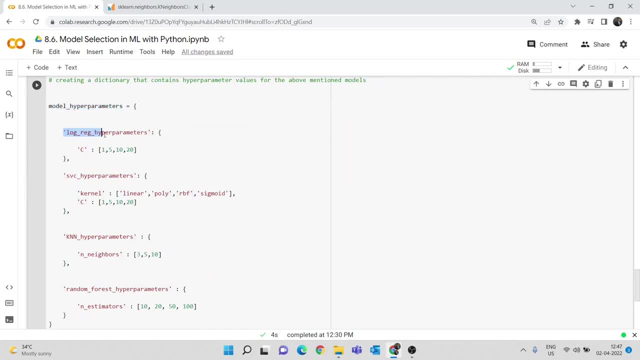 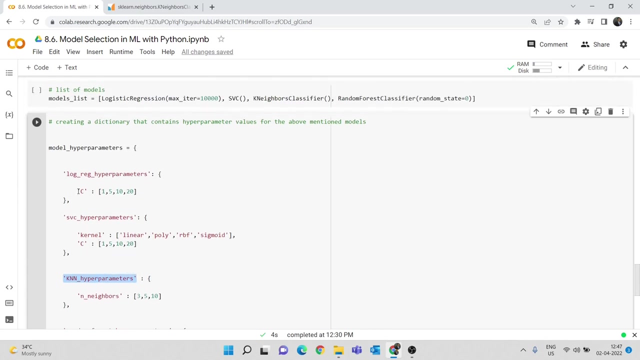 so for this model there are four keys. the first key is logistic regression hyper parameters and the second key is SPCA hyper parameters. third one is k nearest neighbor hyper parameters and finally random forest parameters. so all these four things represent a particular key and the second represents the corresponding values for this key. so this one is the value for this first key. 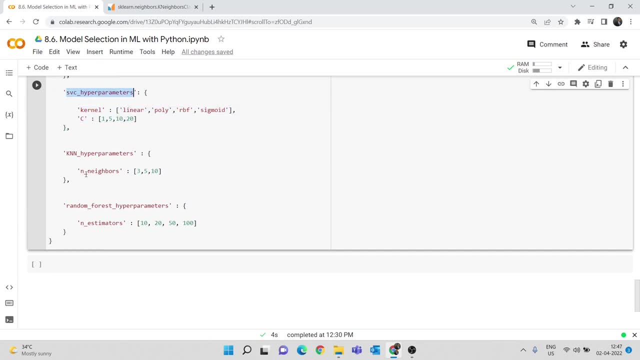 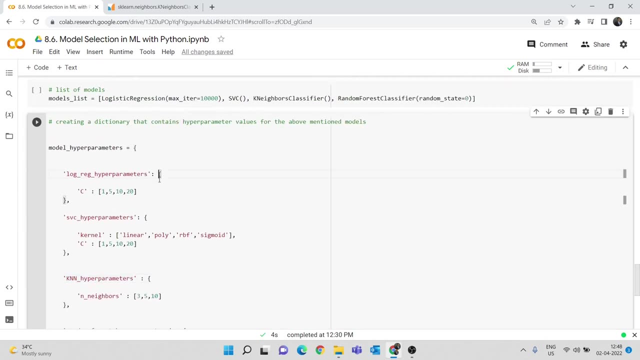 and these two things are the value for second key third one is like: n neighbors is the value for this one, and so on. the only difference is that, instead of having values or list, we are creating a dictionary itself as a value. okay, so if i build a simple dictionary in this case, just a second. 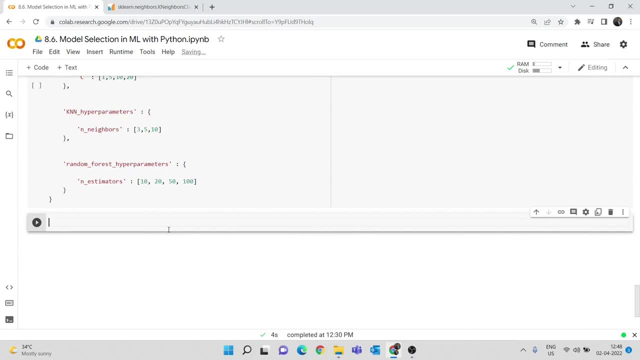 okay. so let's say that i'm creating a, my dictionary let me just put this as a. so a is my dictionary that i'm creating. so here i can say name, so like let's say that name of a person is john. okay, and there is like another key here called as age, and i'm going to say age of this person. 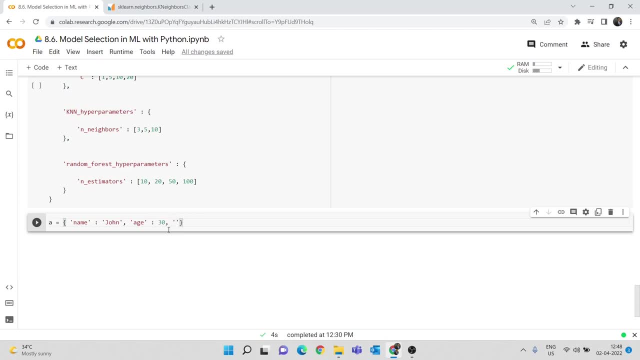 john is, let's say, 30 and let's say the country he belongs to. okay, so country he belongs to is, let's say us. so this is the dictionary that i am creating, and i can also like print this a and c. so this is my dictionary here. 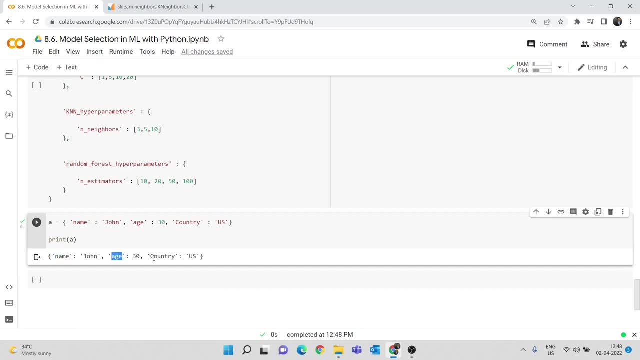 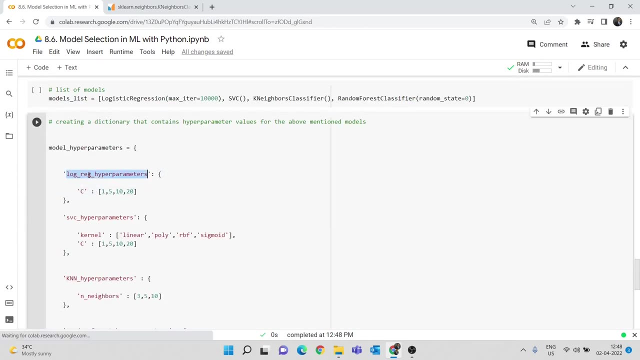 we have three- uh, you know- keys. one is a name and then we have this age and country, right? so this is how we create a dictionary. so this uh keys are similar to what we have created here. so this logistic regression, hyper parameters, is similar to the key name and and then we have this svc. 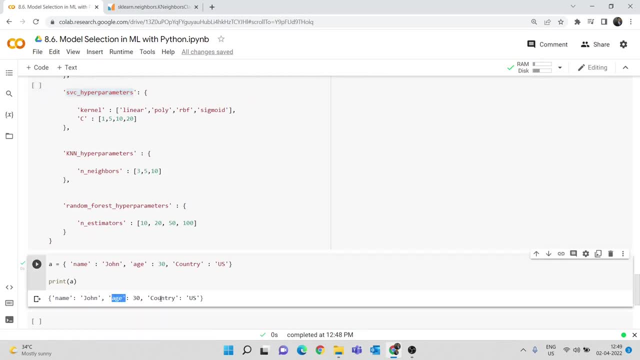 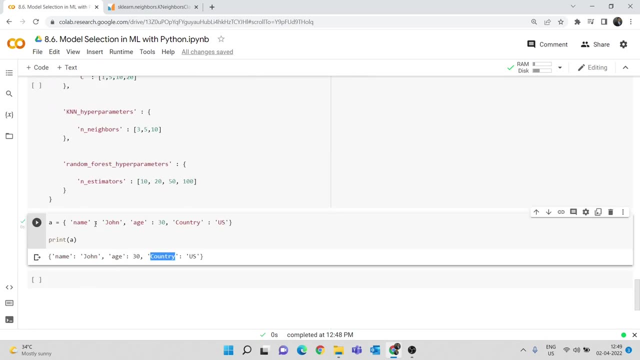 hyper parameters, right? so in this case we have three keys: name, age and country. so, similarly, we have four keys: logistic regression, hyper parameters, svc parameters and so on. the only difference is that the value for this key name is in the form of a string, right? so this is the key and the value is: 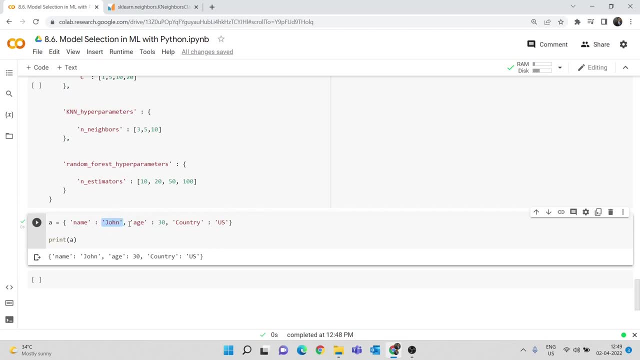 john. the value for this key name is john, and it is in the form of a string, and the value that is associated with this h is 30, which is an integer value, and country is again a string. so the only difference is that, instead of having string or age as my value, i am having another dictionary within. 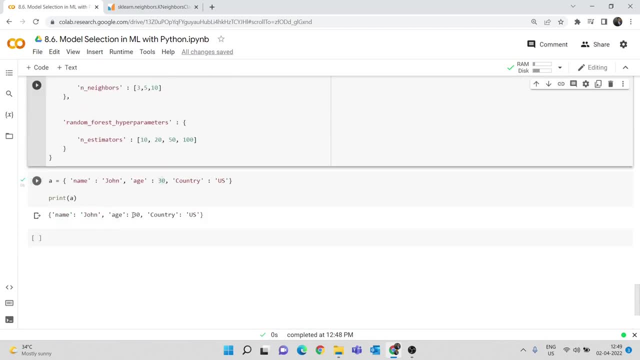 this. okay, so this is the dictionary that i'm considering, with four values. so this is just like saying uh, like uh instead of like john. so what i'm going to say here is: like there can be a list with uh, there can be john, and let's say there is like this: sam. 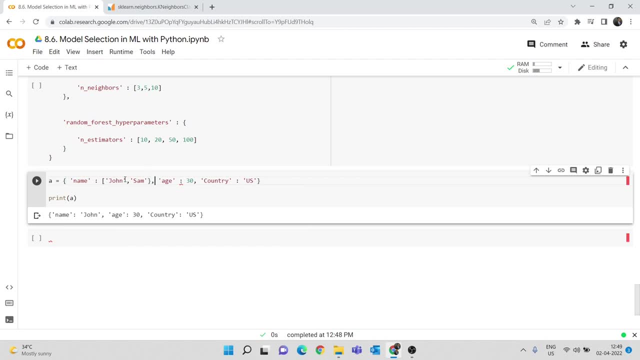 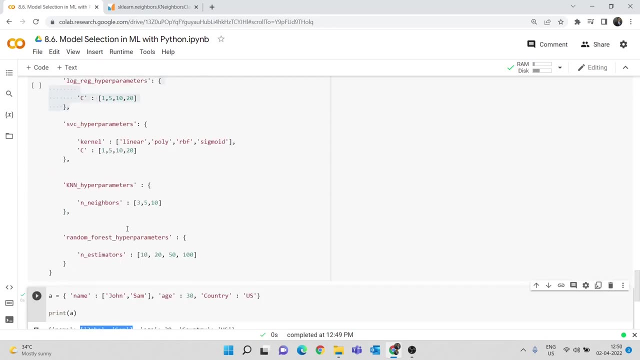 so this is the name of different people that we have, so you can also like create this list like this, so i'll run this one. so, instead of having string, i have created a list here. so, similarly in this case, uh, instead of having a integer or a string or a list, i have created another. 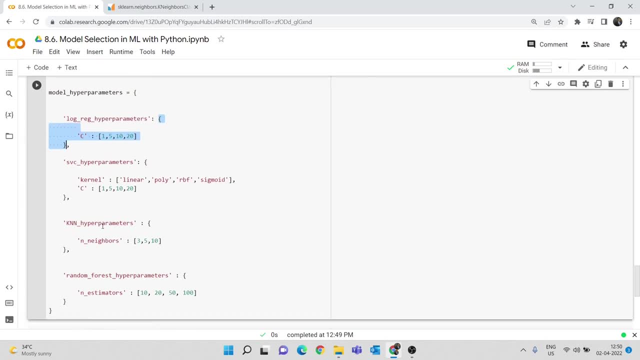 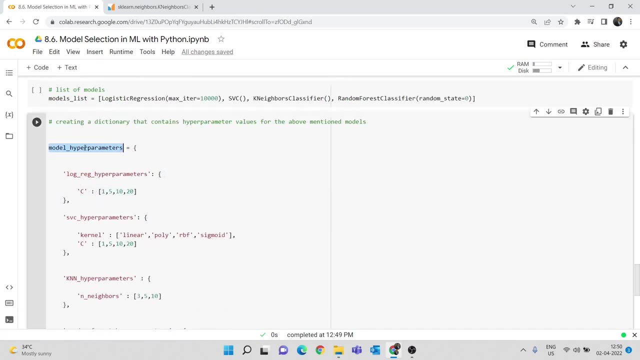 dictionary as my value, so this will be the correct way of- uh, you know, specifying your hyper parameter values. so this is actually a dictionary, but we are just using it in a different form. so we have the dictionary called, as a model, hyper parameters and, within that model, hyper. 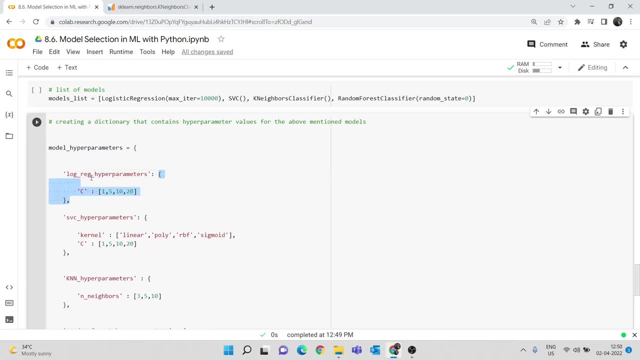 parameter. we have multiple dictionaries, okay. so this is the dictionary associated with the first key value and this is the second dictionary value associated to this, spc, hyper parameters and so on. so i hope you understand this. this is like very important, but this is like very simple thing that 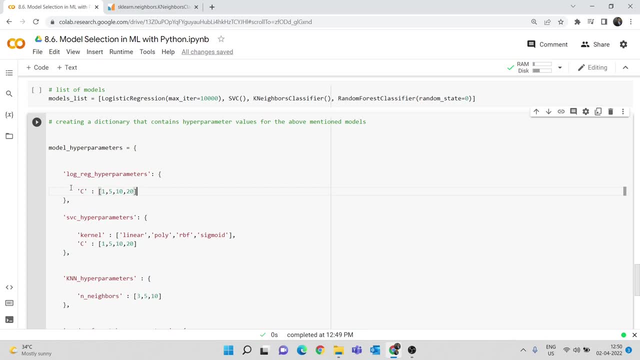 we are doing so in case you wanted to try multiple hyper parameters, so in this case we are going to try multiple hyper parameters, so in this case we are going to try multiple. for logistic regression, we have considered like only one hyper parameter, which is like c value. 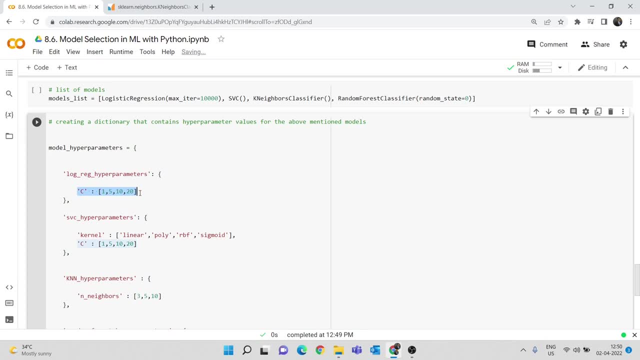 but logistic regression, all just other hyper parameter values as well. in that case, how you can do that is like how we have done this for support vector classifier, for support vector class, where i'm considering like two hyper parameters: first one is kernel, second one is like c. so that's why i have to include this comma here. so i'm just saying like there are like two. 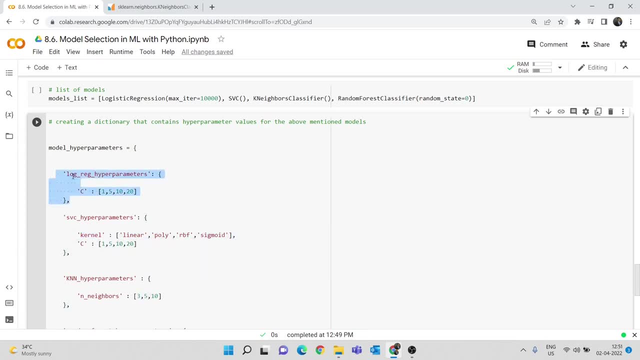 set of hyper parameters for which i have to check. so this is my first key value pair. so i have separated with this comma. this is my second key value pair, so this is my first set of values. this is my second set of values. this is like third set of values, so all these things should be separated. 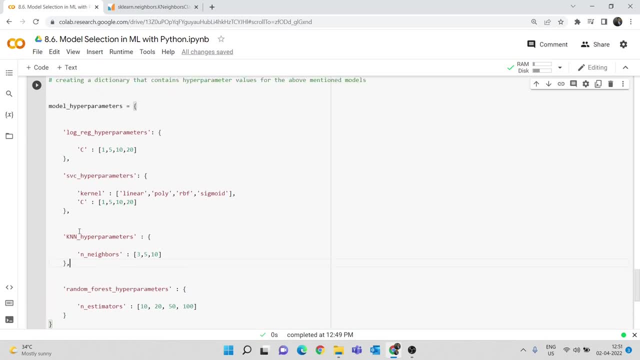 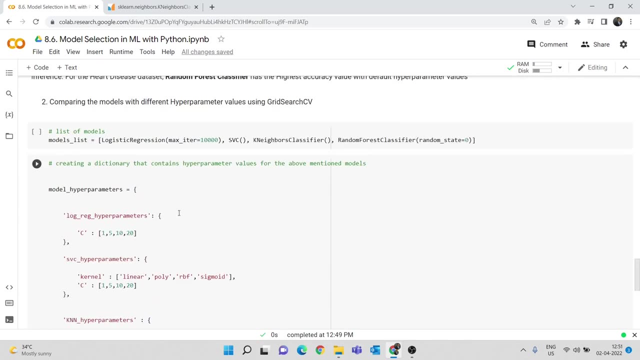 by this comma and this is like very important. if you remove this, it will be- uh, you know, it will basically show you an error. okay, so i hope you understand this part. so we are just creating a list of models and we are creating hyper parameter for the listed models. the only important thing here. 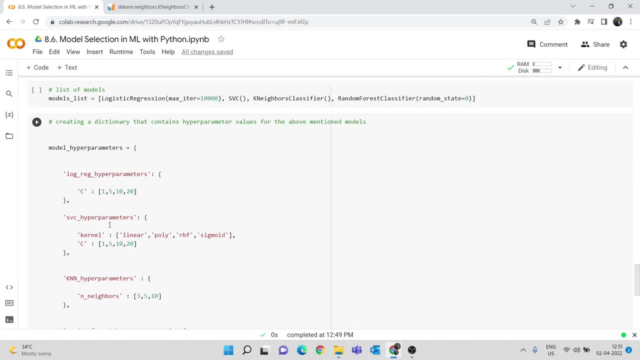 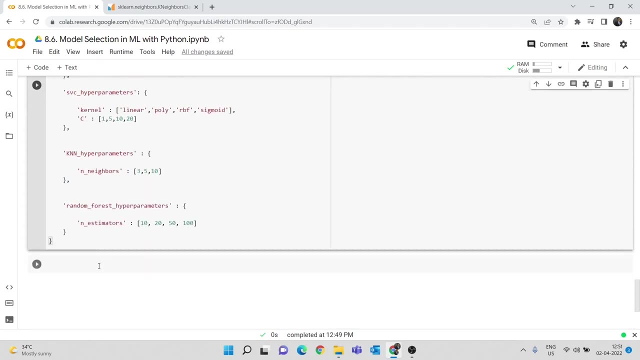 is. we are creating, uh, it in the form of a dictionary so that we can use it efficiently. okay, so model hyperparameter parameters is the dictionary that we have created, so i'll copy this and paste it here so you can also check the type of this model hyper parameters. it will tell us that it is in the form of a. 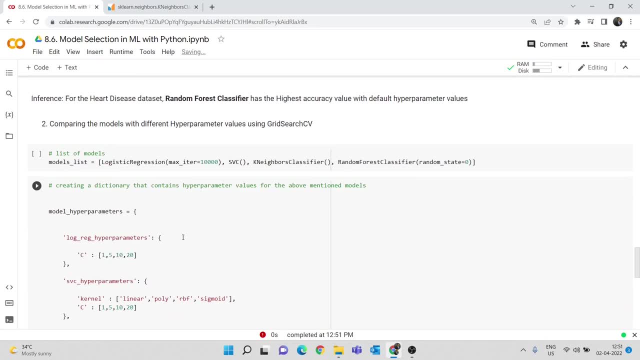 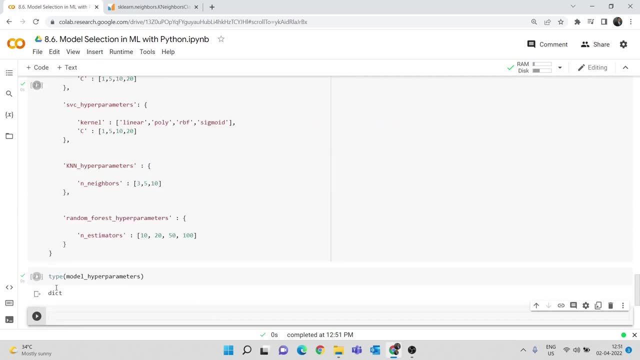 dictionary name is not defined, okay, okay, so i have to run this cell first. so it seems like i didn't run this. okay, so i'll run this one. okay, dict, so d-a-c-t, which stands for dictionary, and i can paste it here and i can say keys: okay, so let's print this: keys of this dictionary. 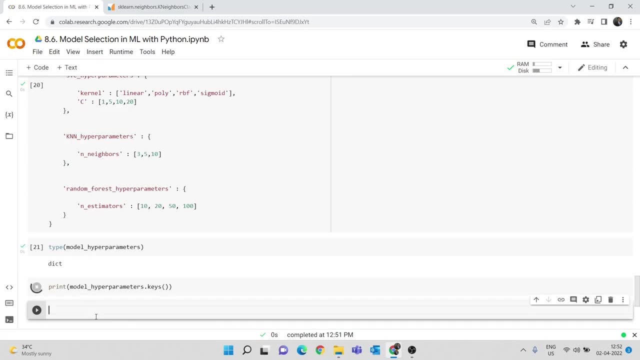 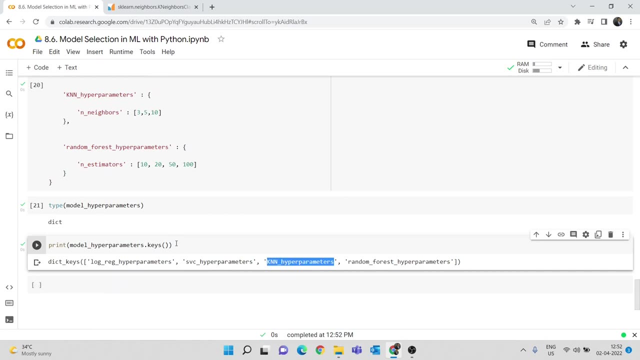 let's see what is the output we are getting. so when i say model hyperparameterkeys, so these are all my keys: logistic regression hyperparameters, sbc, hyperparameter k, and then hyperparameters and so on, and they can also check the values of this or items of this. so 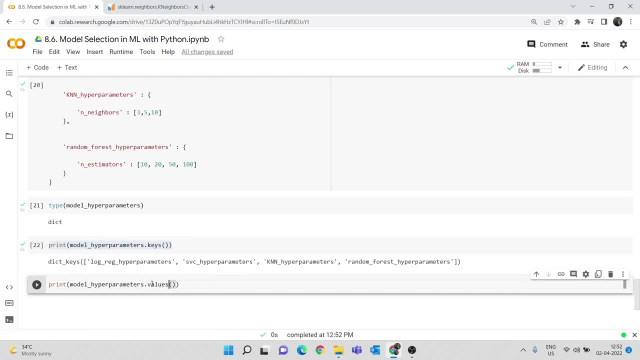 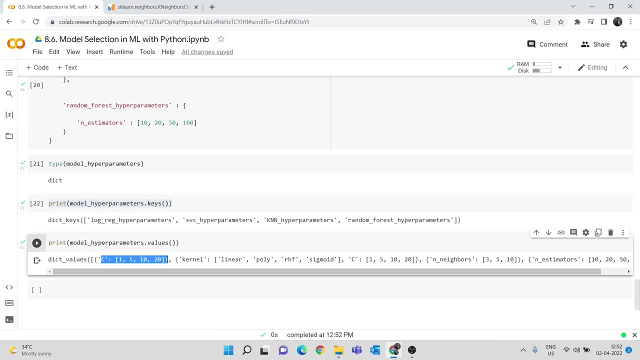 let me just put this as model hyperparameters, dot values. so these are the values. so the value for logistic regression hyperparameters is the c and the value for sbc hyperparameter is this one: kernel and kernel and c. as you can see, all these given in a dictionary format. so this is how you can analyze the dictionary that you have created. 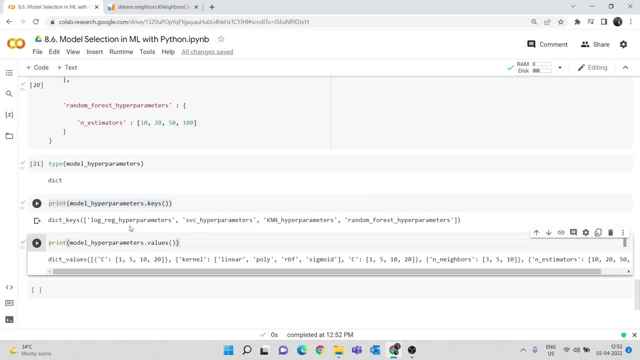 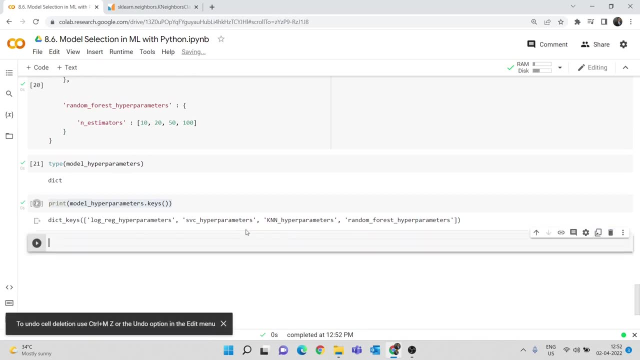 so when i say: you know, let me put this as keys, as okay, i'll just remove this one. so i just want this keys alone, i'm going to convert this keys into a list, so let's create a variable for this model. keys is equal to list of. 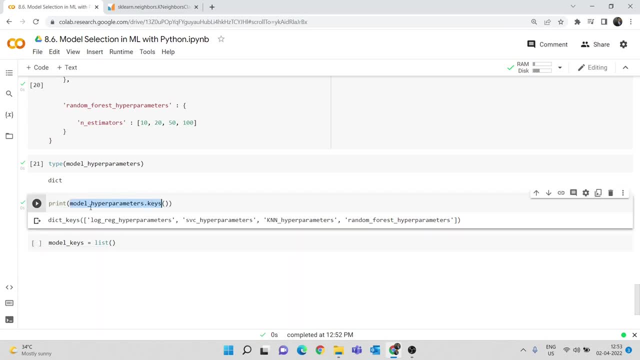 model, hyperparameters, dot keys, and i'm going to print this model keys, okay, yeah, so i have created a list which contain all these keys, so we need this in order to access, uh, the data that we have. okay, so how you can do this is like, if you, you know, copy this name: model. 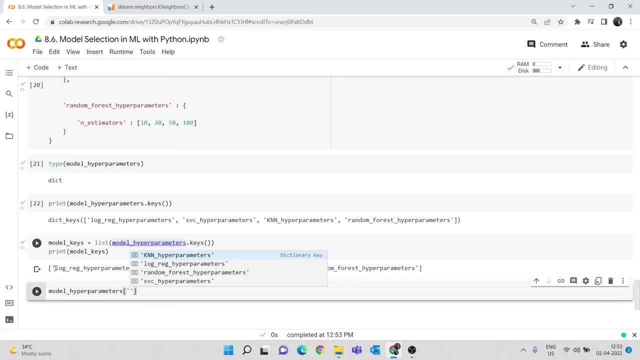 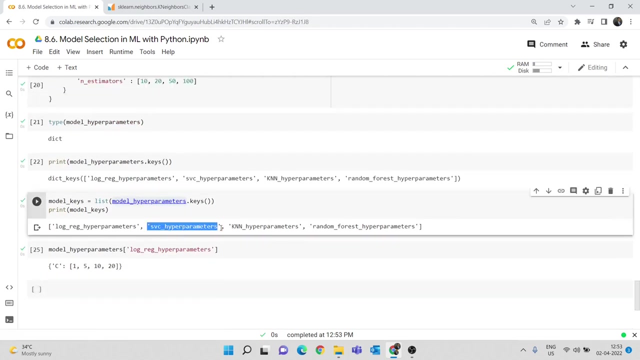 hyperparameters and if you save the name of a particular key, so this is my first key- i'll copy this if i paste it here. so if i paste this within the square bracket, i will get the corresponding value for this particular key. as you can see, if i just replace this with this spc hyperparameters. 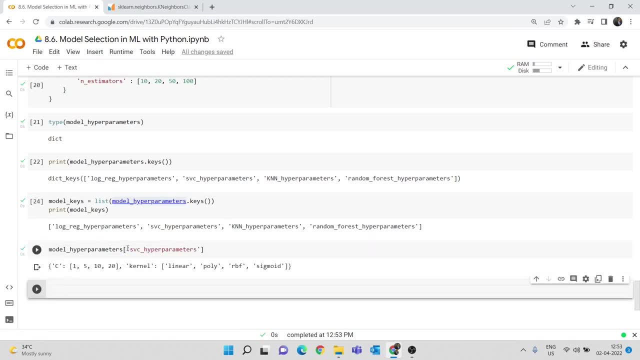 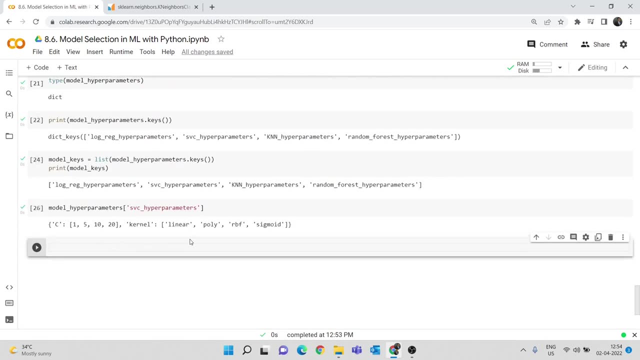 i will get the corresponding value for support vector machine classifier. so this is how we are going to access the individual hyperparameters for the models that we have created in this list. okay, so that's why i've created this list, called as model keys, and instead of using this spc or hyperparameters and something like that, we are going to use the. 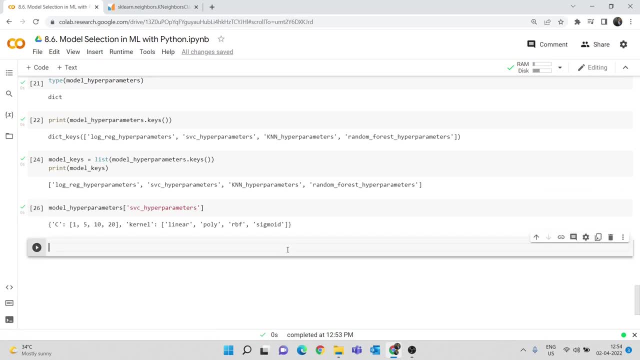 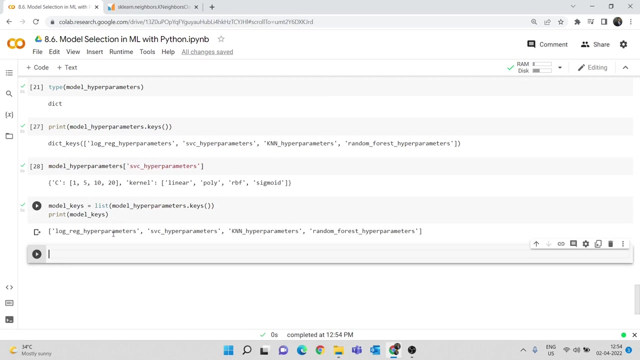 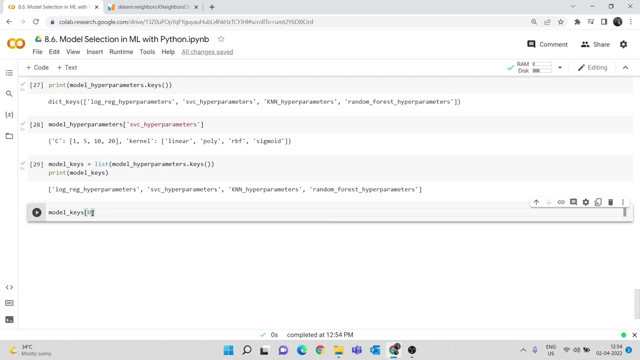 index of this particular list. okay, so let's say so, this is the list we have created. so let me just move this cell above. so this is my keys and this is the list that i have created. and we know that we can print the first value of the key using the index, right? so when i say model keys of zero, 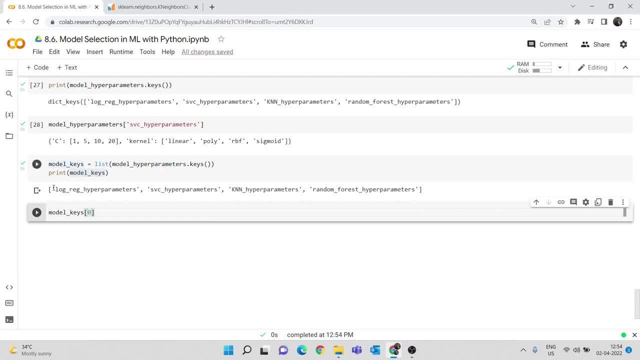 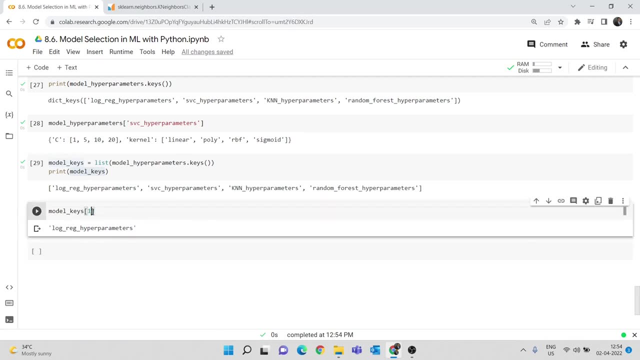 and model keys is the list that i've created. when i say zero, this first element will be printed. the first element is logistic regression hyperparameters. right, when i say one, the value with index, one is spc hyperparameters and two is for k nearest neighbor hyperparameters, and so on. so 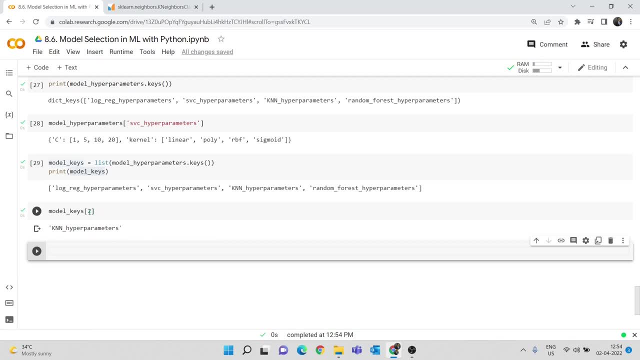 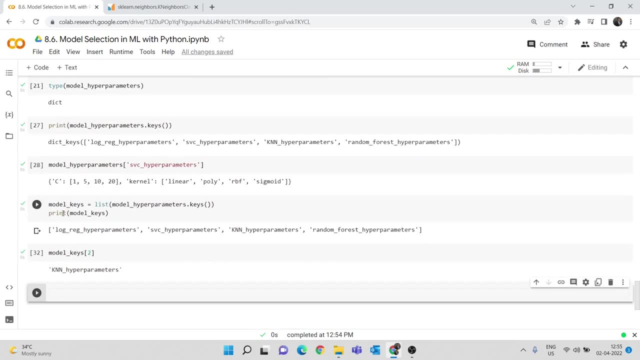 this is how we can print this and this is what i'm going to use. so i'm going to all these keys- instead of their name, i'm going to call them from this list called as model keys. so the important things that we have to do here are creating this list that contains the name of all the models, creating 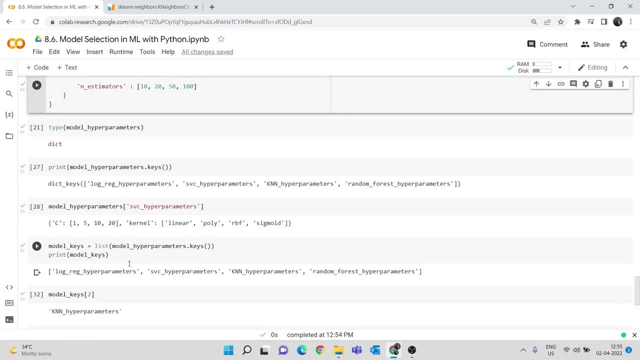 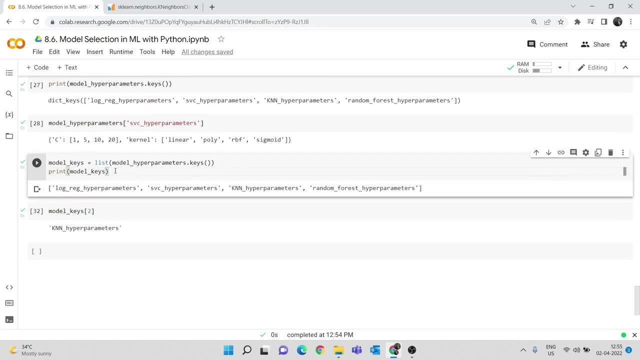 this dictionary and converting the keys into a list. so these three are like very important steps that we have to consider. so first is like creating the list. second is creating the dictionary and converting the keys in in the form of a list. so when i say model hyperparameters, 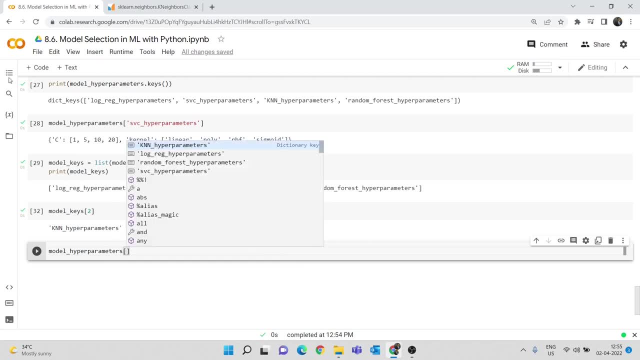 and within this, instead of you know like, instead of mentioning this spc hyperparameters or logistic regression hyperparameters, i can say model keys of zero. so when i say model keys of zero, so the value that i will get is: so this is how i'm going to access my hyperparameters. okay, so if i say uh, 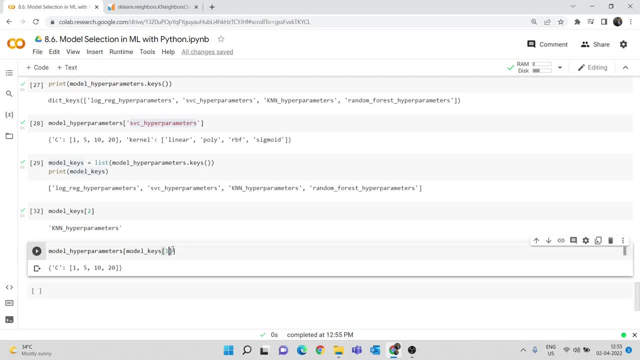 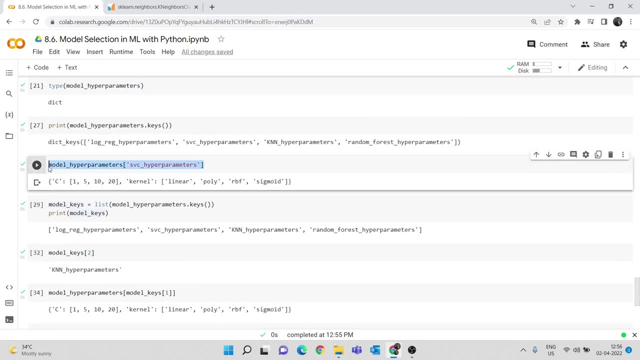 keys of one, i will get support vector machine class for hyperparameter. so what i'm basically doing here is, instead of saying model hyperparameters, i'm going to say model keys of one parameters of spc hyperparameters, i'm going to say model hyperparameter. model keys is equal to one. 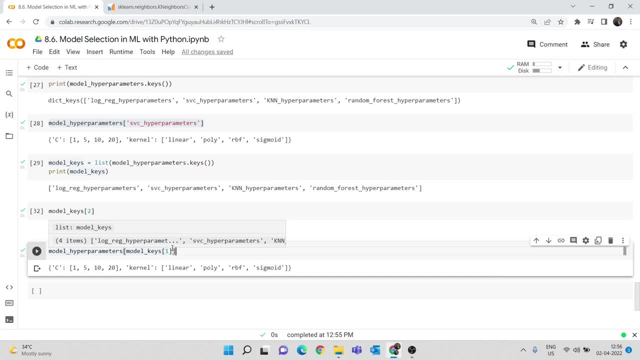 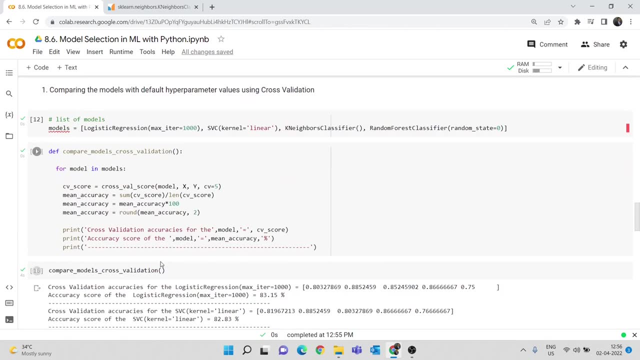 so we are just doing this in a uh, you know, in a different way. the reason is we will be creating, you know, another for loop, so we'll be creating a function and we'll be creating another for loop, like we have done for this one and uh, in that case, instead of you know, using the keys, as such it is. 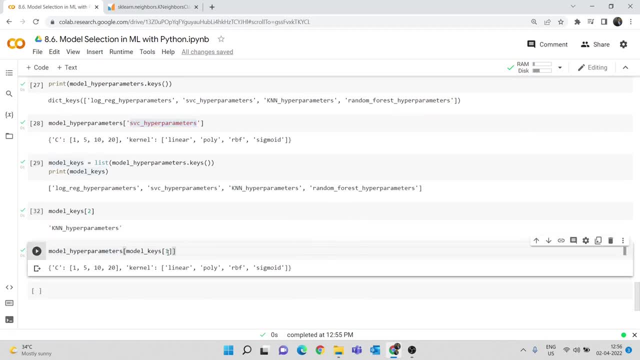 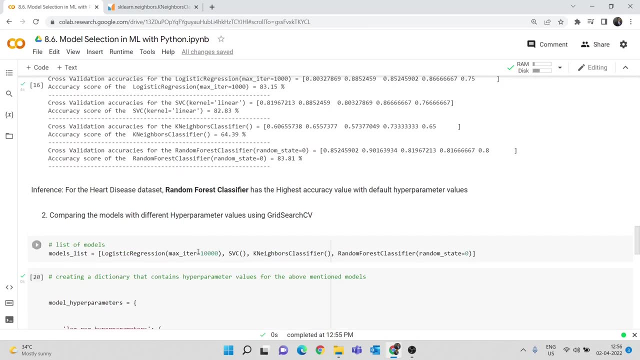 always better to kind of load it to a dictionary and call the values using this index. so you will understand why we are doing this. but you know these are all the steps that we have to do before creating that particular function. first is creating the list, and then creating the dictionary and converting the keys in the form of. 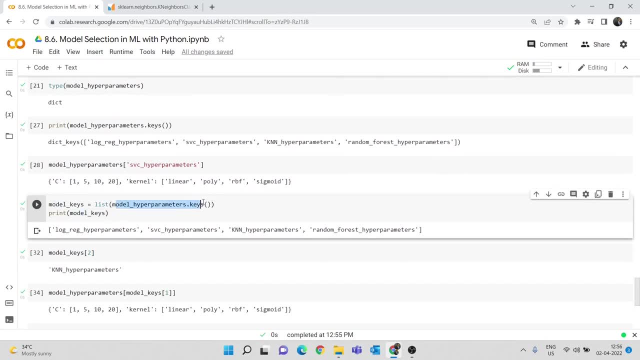 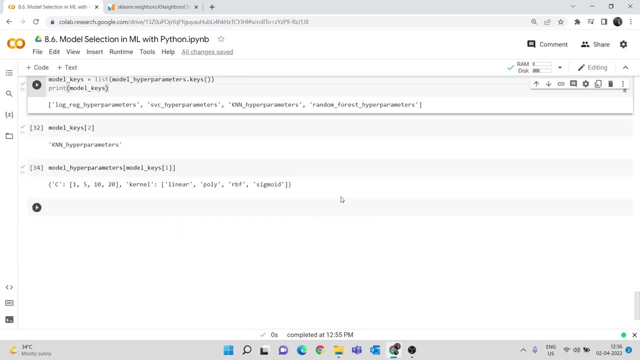 a list. okay, so as we have done here, so i'm taking this list and then converting all these values into your list using this list keyword. okay, and now let's try to create this function, that kind of uh, do this model selection, but with different type of parameters. previously we have trained our model. 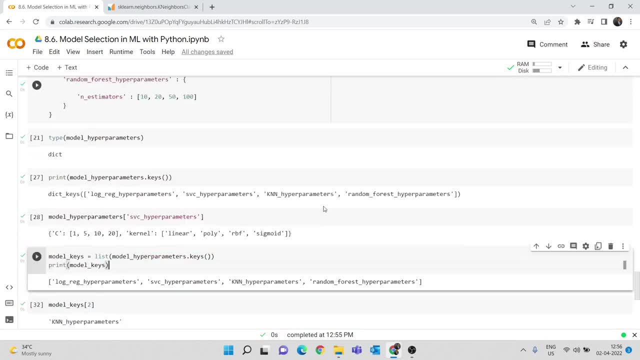 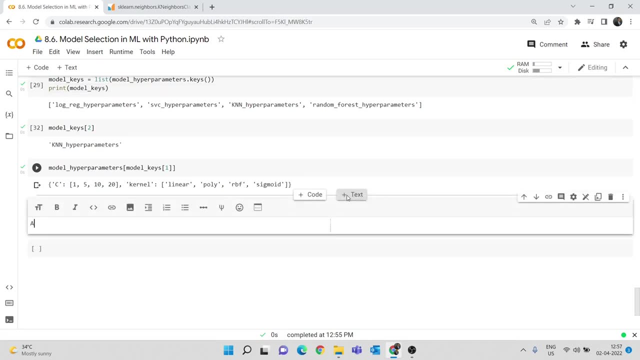 with only the default values right now. i'm going to consider different type of parameter values. so and yeah, so here i'll just make a text here as applying grid search cv. so grid search cv is the hyper parameter tuning function that we have, and this is how we are going to select our models as well, so i'll create a. 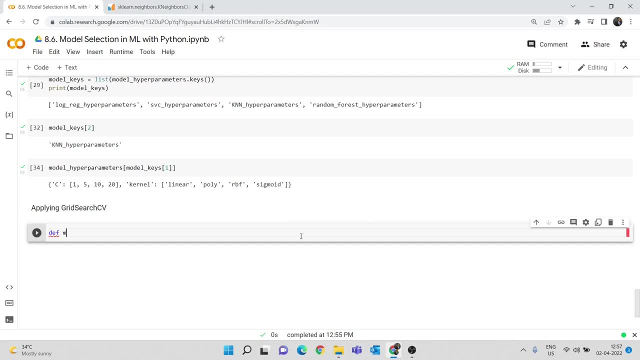 function as def. so def stands for define, which is used for creating a particular function. now name this function as model selection. okay, so model selection. or let me put this as like this: model selection. so let me just change the case of m and dn- sorry, m and ds- and the parameters that i give to this particular 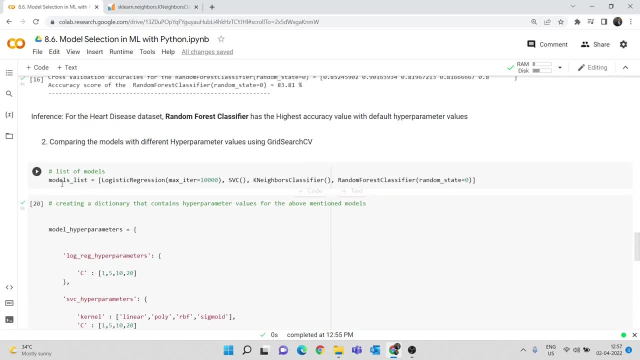 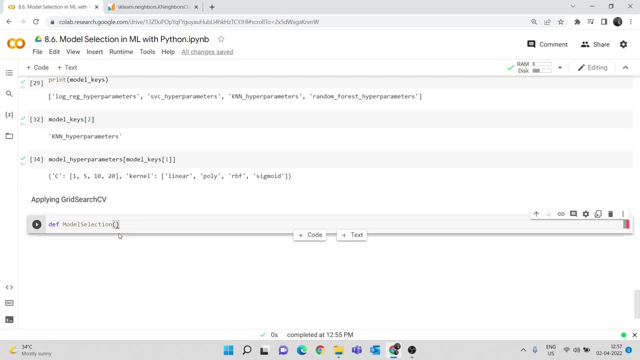 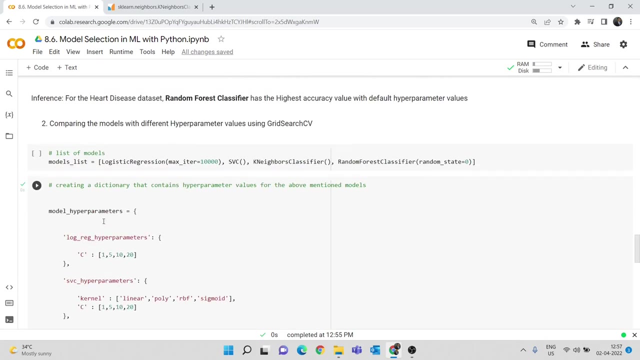 functions are the list of the model that you have, that i have created, and the hyper parameter dictionary that i have created. okay, so here i'm going to say list of models, or let me just put this as so. let's not use the same name that we have created here. let's put this as models. so first, 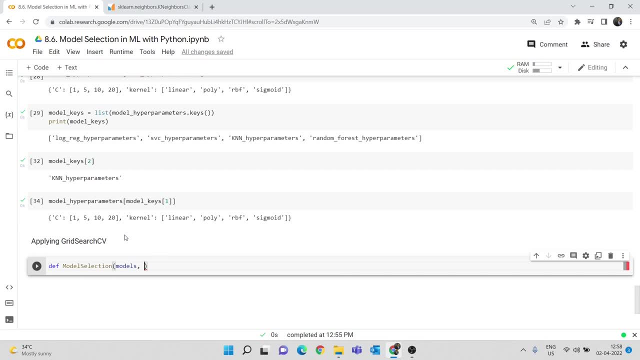 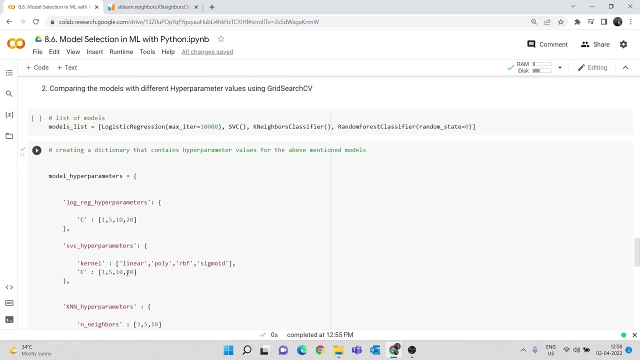 models and is hyper parameter, so let me just put this as hyper parameter. hyper parameter dictionary. okay, so i just don't want to use the same variable name that we have here, the model, hyper parameters, model list. so let me just put this as a list of models. 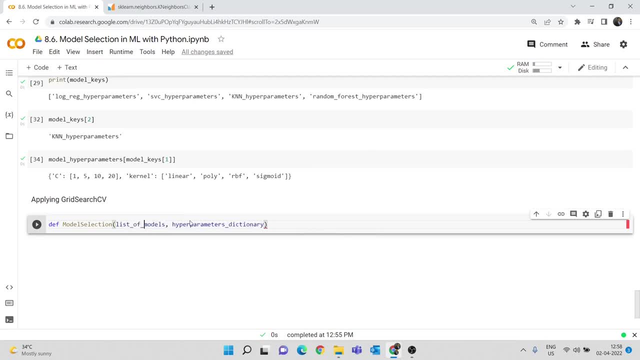 okay, so list of models and hyper parameters dictionary- okay. so i don't want to use the same thing because, like, it will be directly passed to it. so i'm creating a function that i'm mentioning, like that we have to give two parameters to this, so the first parameter is: 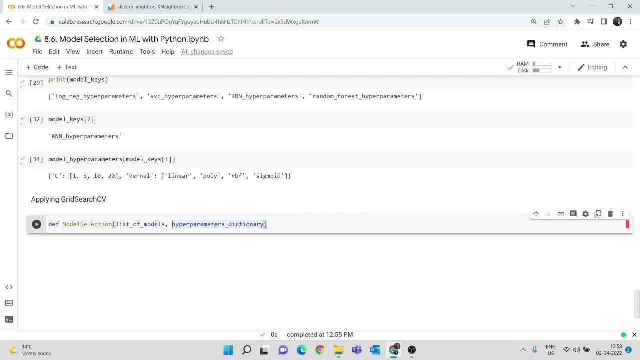 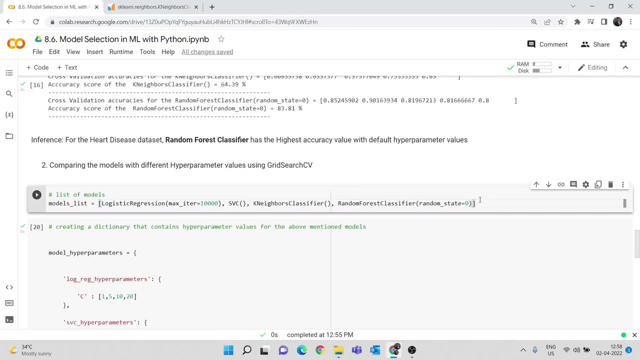 the list of models. second parameter is the hyper parameters dictionary, the two attributes that we have and the reason i'm creating this function is, if you want, you can add another model to it. so you can add, you know, another classification model to it and you can add the corresponding. 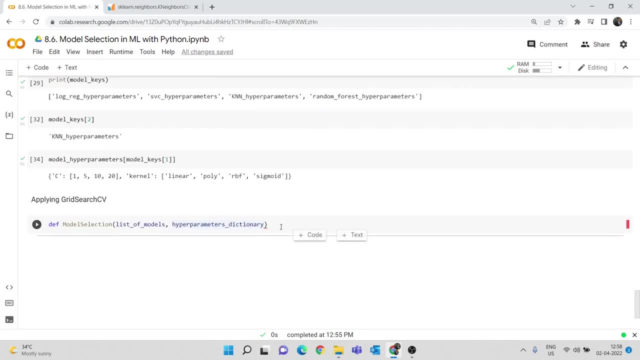 hyper parameters to that particular model as well. so that is this reason i'm creating this. so the name of this function is model selection, and here i'm creating an empty list. so result is equal to i'm creating an empty list. so this is where, so in this list only, we will store all the best. uh, you know, hyper parameters. 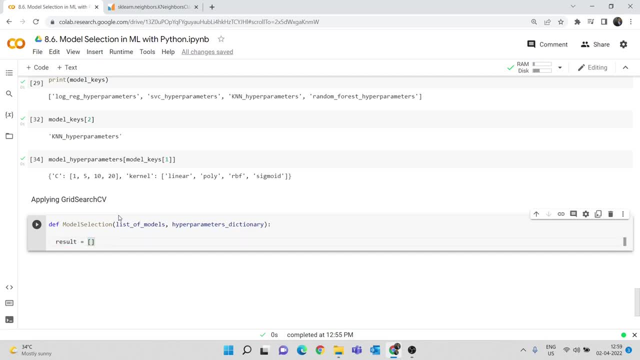 so we will like check which parameters has the best value, so we will be storing all those things in this empty list, which is this: result is equal to this square bracket. so this is how we can create an empty list. i'm going to say: i is equal to zero, so we need this. i, so this. i is uh, just for this. 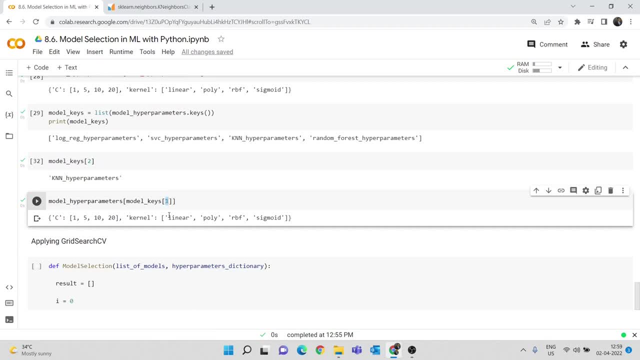 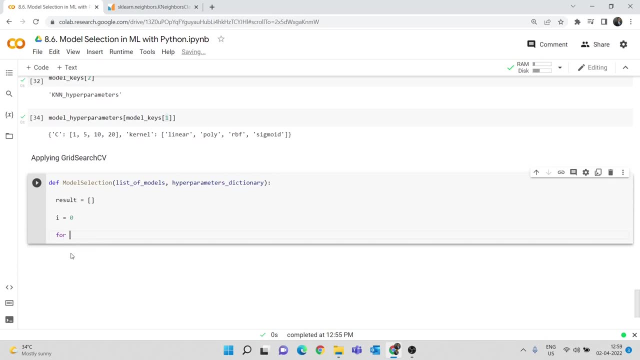 index. so we have seen that we will call the hyper parameter using this index rate. so for that, we are creating this i and i'm initiating this, i as 0, and this is where i'm going to create my for loop for model in this list of models. okay, for models in list of models. 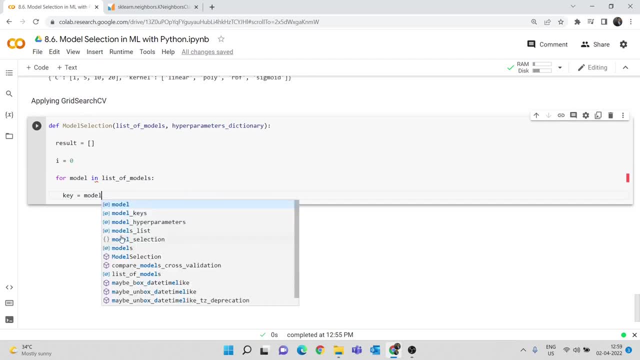 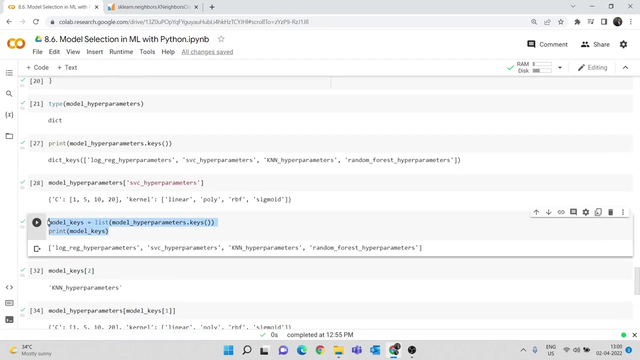 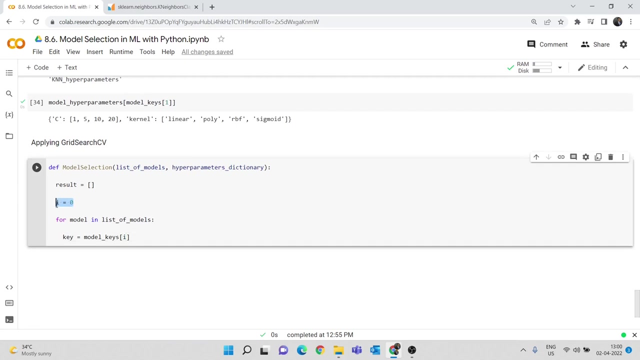 he is equal to model keys of i. so this model keys is nothing but the list that we have created here. yeah, so this is the list that we have created and i is the index. so the follow up when the you know follow up runs, for this first time, the i, the value of i is 0, so model keys of 0 is nothing but so when i say model, 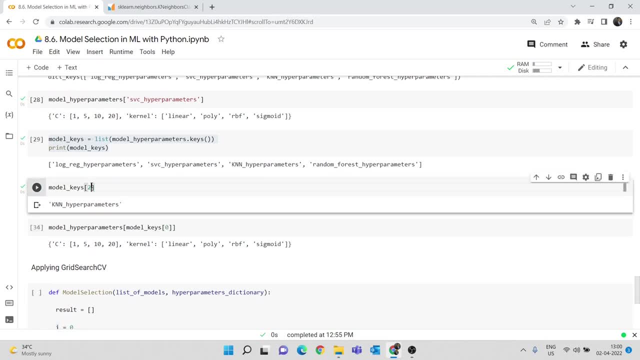 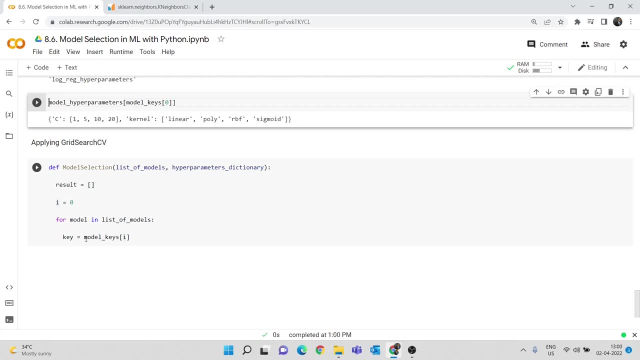 keys of 0, or when i say model keys of 0 here, the value that it will print is logistic regression, hyper parameters. right, so that is what i will get here. so when i say key is equal to model keys of 0, the value of key will be logistic regression, hyper parameters. and now the parameters. 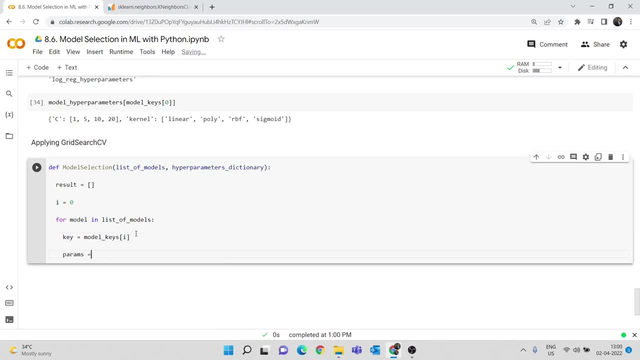 so we have to check what is the parameter. so i will create a variable as params. so this is where we are going to pass the parameters of this logistic regression model. so i will say: model, hyper parameter, model of keys, that particular index, right, so i can say this as the hyper. 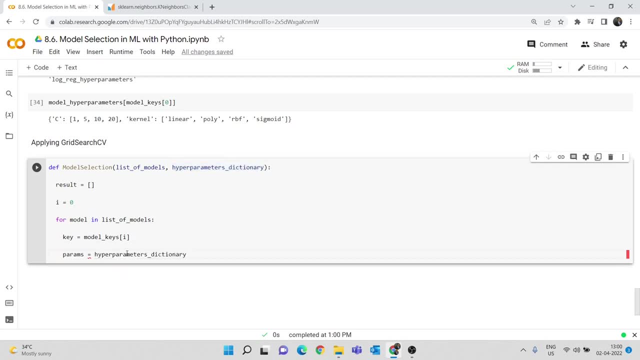 parameters dictionary. so if you do not understand what we are doing here just like, please hang on. so once i complete this, i will also explain you clearly on all the steps that we are doing here. so it is, i am going to say key, okay, and then i am going to increment this equal to 1 and i will also 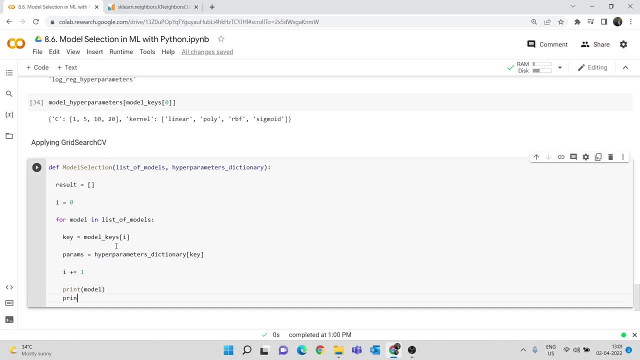 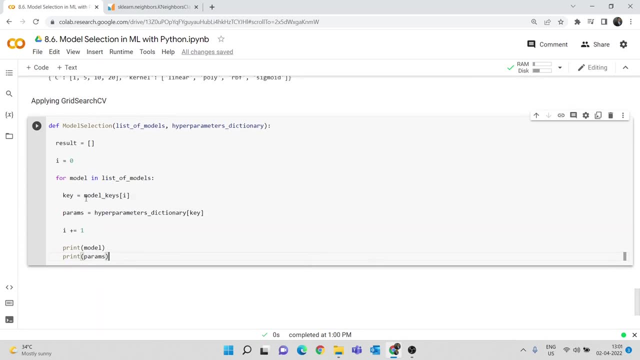 print the name of the model and i will print the hyper parameters that we are using using this params. okay, so what we are basically doing here is like a: we are just specifying the model that we are going to use using this for loop, and i'm just 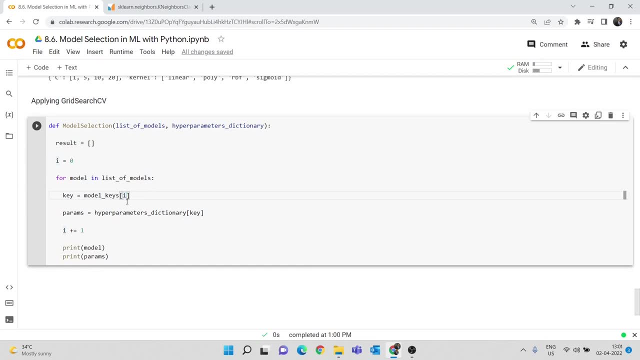 creating this index so that we can call that specific model's hyper parameters. so i'll also explain this again. but this is, for you know, combining that model and the hyper parameter of that particular model. the reason is that i cannot use this set of hyper parameters, right? 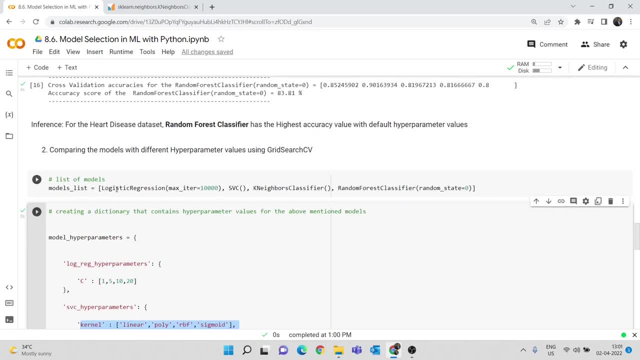 i cannot use this c and kernel while i am uh training the model with this logistic regression, right? so when i'm, whenever i'm training with this logistic regression, i should use this, uh, this set of parameters and like, while i'm training, training it with this spc, i have to. 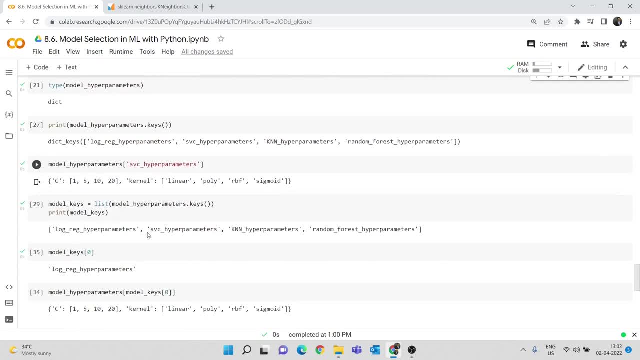 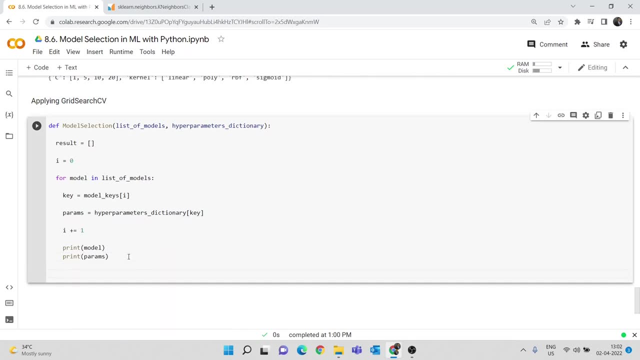 use this spc hyper parameter. so that's the reason, and, yeah, so that is why we are creating something like this. and once we have done this, we can, uh, you know, build our grid, search cv, uh, you know, function. so we'll create a variable as classifier. so classifier is equal to we have to use the grid. 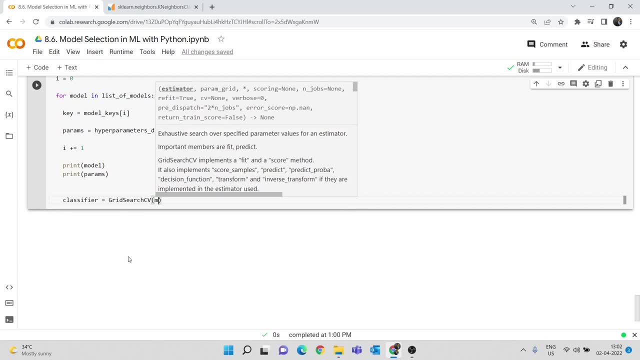 search cv function, grid search cv- and we have to give the model, so the first attribute that we have to give us, like the model which using which we are going to train our data. then we have to give the params, the parameter that we are considering and cv. so what is the cross validation? 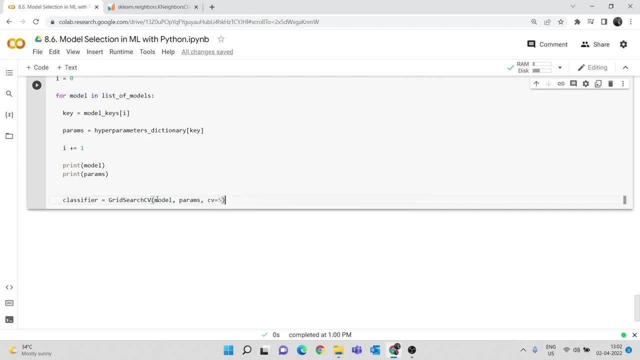 number of folds for your, this cross validation and so on. so this is like: uh, creating the instance of this grid search cv using this classifier variable, and now we have to fit the data to this model, fitting the data to classifier, and i'm going to say classifier dot fit. 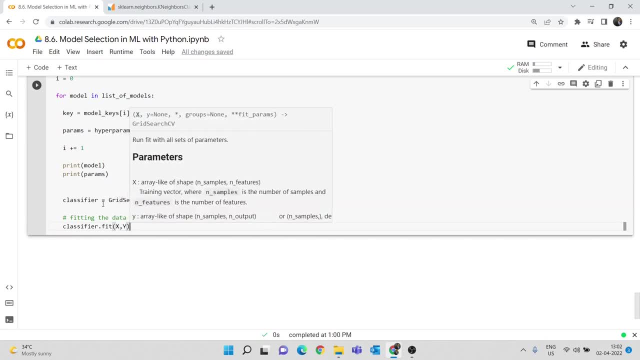 classifier dot fit x, comma y. so this classifier is nothing but the grid search cv. so when this form friends for the first time, so grid search cv will be applied for logistic regression and, uh, the logistic regression will be trained with the training data and test data. the result is: 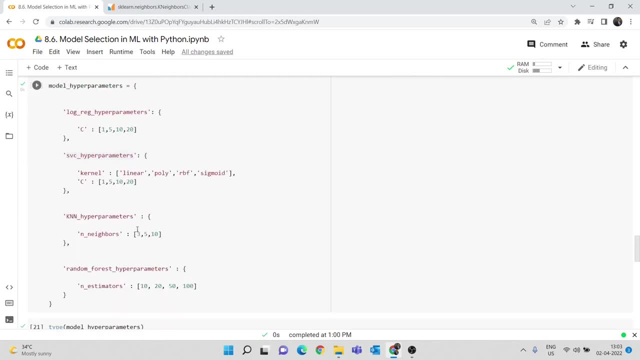 that we will get the accuracy score for all the different hyper parameters that we have used. so we will get the hyper like accuracy score when we use hyper parameter one and hyper parameter 5, 10, 20 and so on. so this is what it, you know, kind of happens. and finally, i'm going to store this, uh. 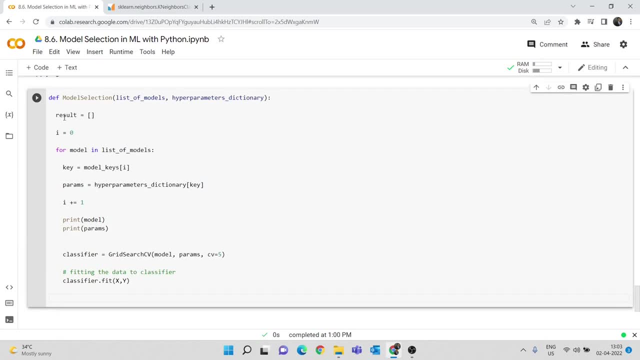 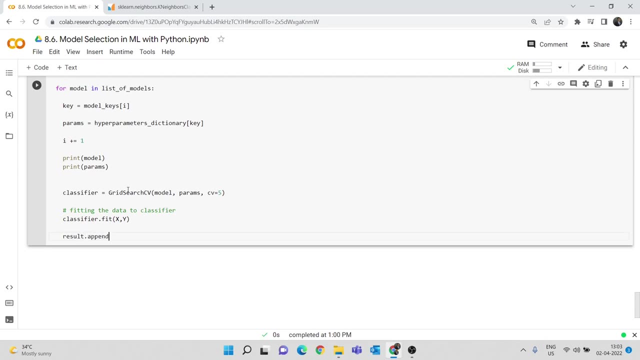 you know, paste result in the list called as a result. okay, so this is where we have created this empty list. i'm going to say result dot append. so append is the function that we use in order to, uh, you know, add a new values to our list. and i'm going to do this in again in the form of: 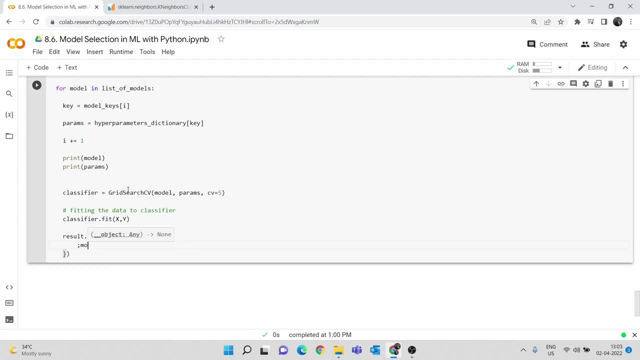 a dictionary, so i'm going to say model used, model used, so we have to mention model. so if you haven't watched my grid search cv video, the hyper parameter tuning with python, python video, please watch that video first and then only you can kind of you know, understand how. 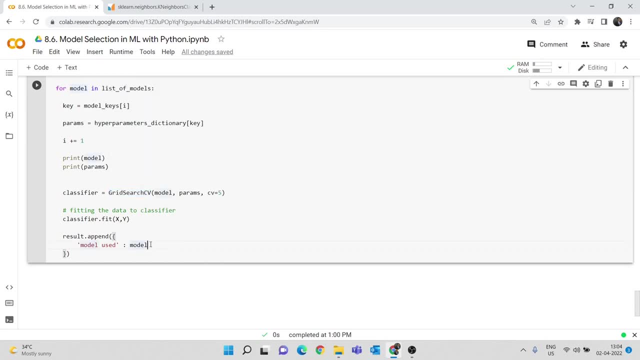 this grid search cv works and so on. so that is like very important. otherwise this may not make sense to you. and the next thing i wanted to add is the highest score for a particular parameter- so i used to score is equal to, i can say, classifier dot, best score underscore. so you have. 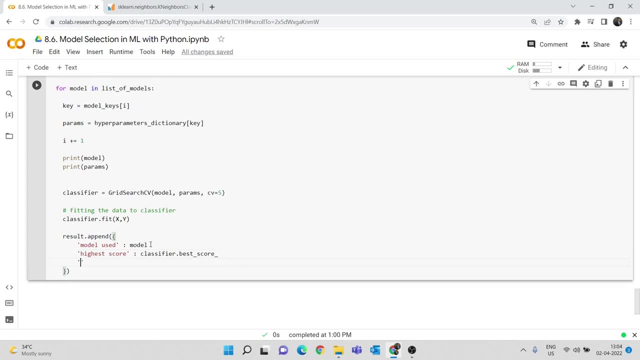 to mention this, underscore after score. and the third thing that i'm going to consider is best type of parameters- okay, so best hyper parameters is classifier dot. best params best- okay, so best params. this will be stored. and finally, let's create a simple data frame using this data frame. so let's create a simple data frame using this data frame. so let's create a. 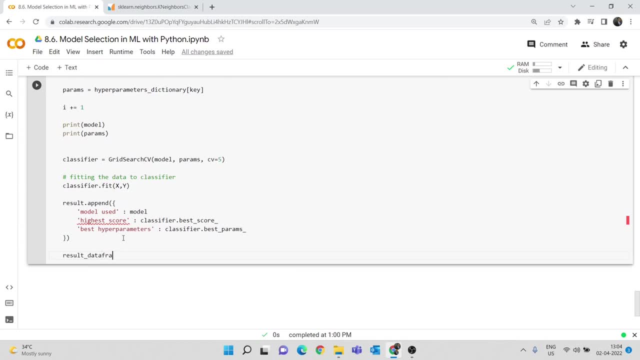 dictionary. so result data frame. i'm creating a data frame here which is equal to pd dot data frame and result columns is equal to first column that we will put is the model used for this jeweler. so these are the column names for my model, and the second thing that we have to consider is the is to score. 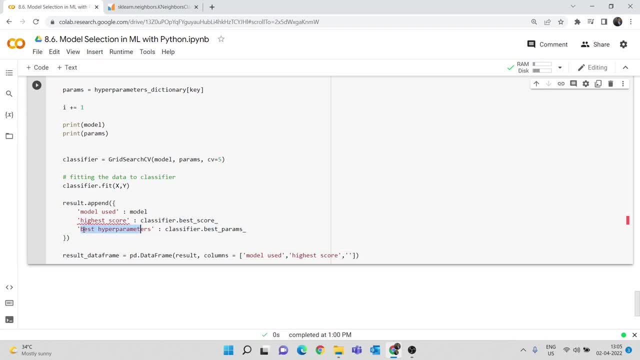 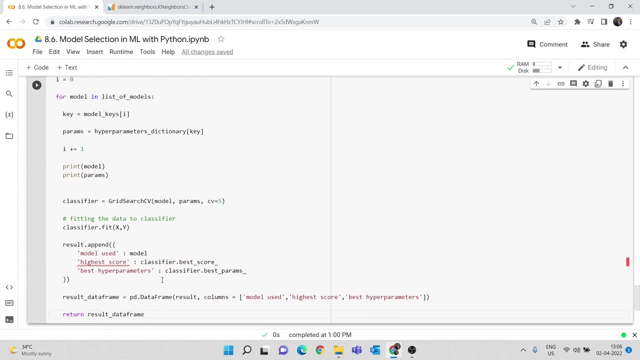 and finally, the best hyper parameters. okay, so we are just finding the uh hyper parameters for which we are getting the is result, and then we are storing it in a dictionary and finally we can return this, return this data frame, so return result data frame. okay, so this is the function that we are creating. okay, so I think everything is. 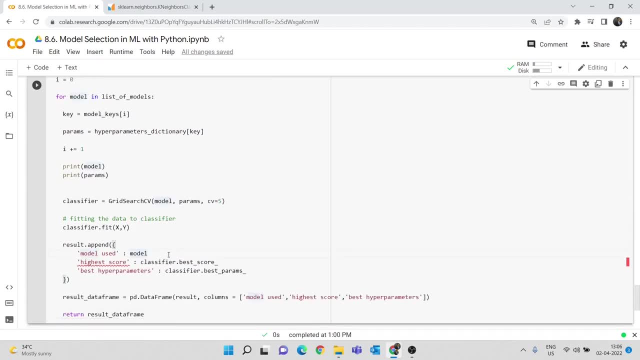 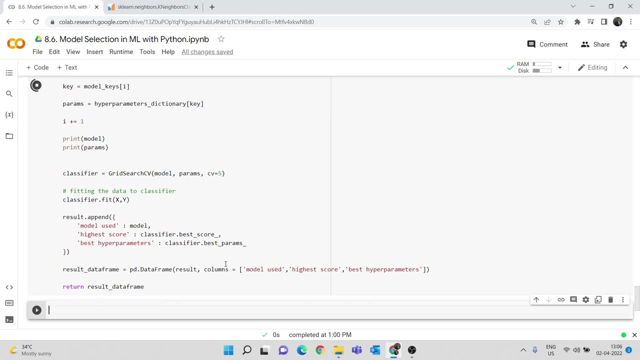 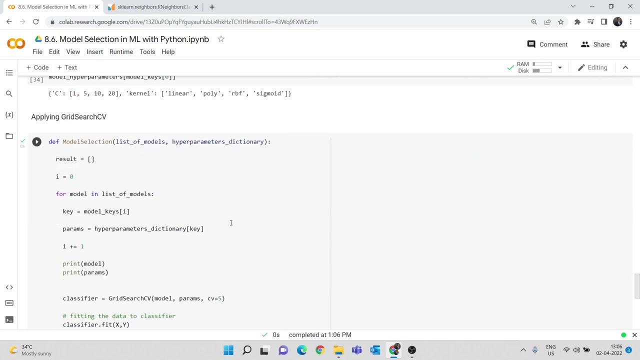 correct in this case. yes, to score. okay, so we have to put a comma here. these are different set of values. let's from this and now I'll call this model selection and now I'll pass my models that I'm comparing, which is my models list, and then this model hyper parameter. okay, 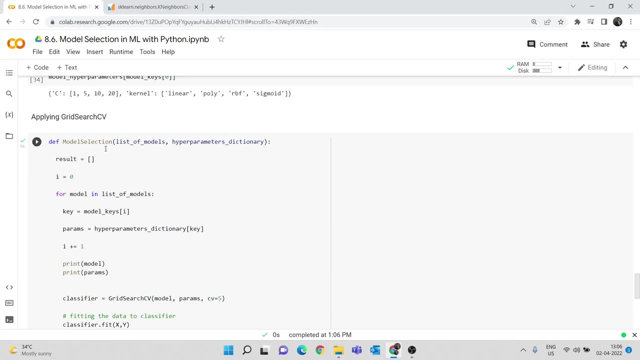 because these are the two parameters that we have to pass. one is we have to pass a list that contains the contains the name of the models that we are using, and then we have to pass a dictionary that contained the hyper parameter values. so the first is the model. 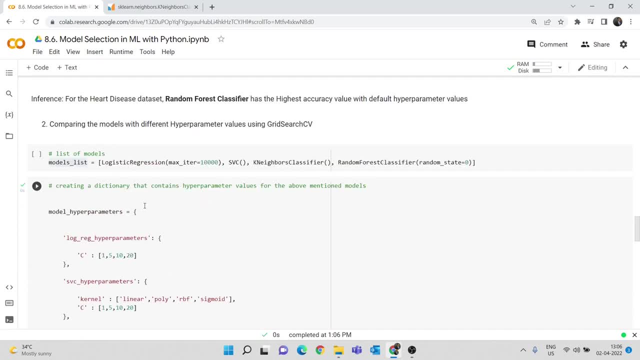 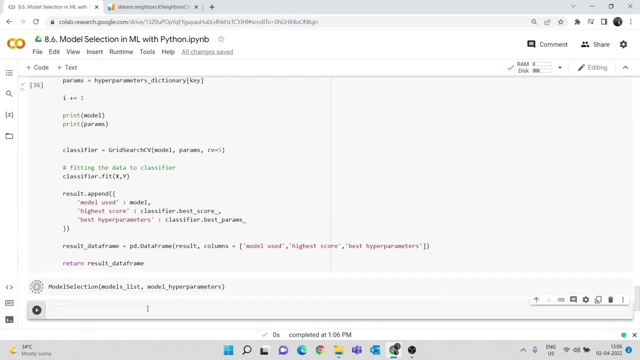 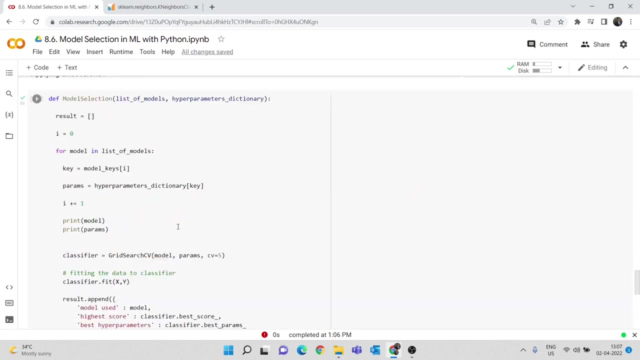 models list. The second one is model hyper parameters. We run this one. The models list is not defined. Okay, I think I didn't run this, Yeah, so I didn't run this in, So that is the reason I'll just run all these things again. 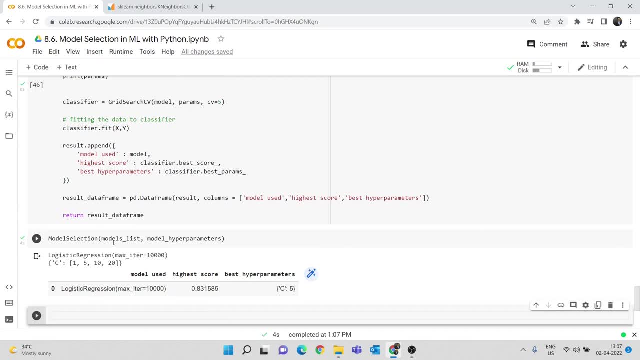 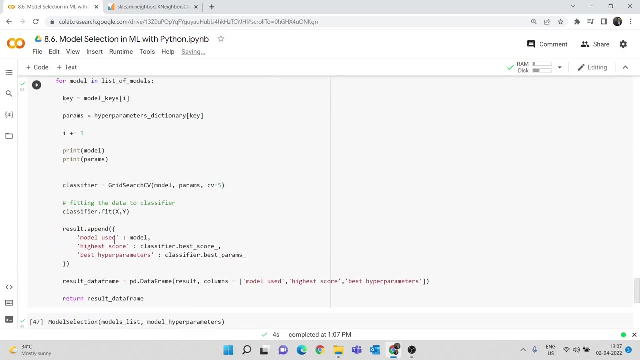 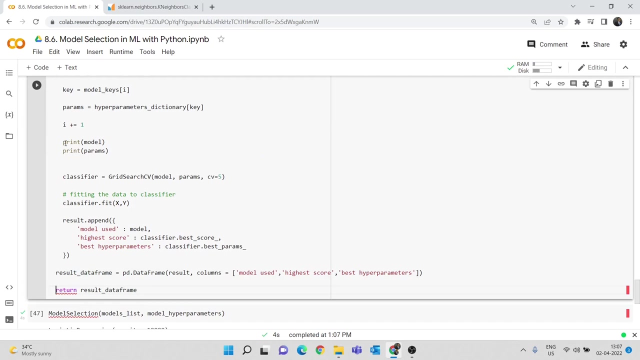 That's it. Okay. so there is some issue that's happening in this, for let me just check this one, Okay. so this: should this result thing should come out of the for loop. As you can see, there is a for loop that we have yet, So come out of this. Let me run this again. 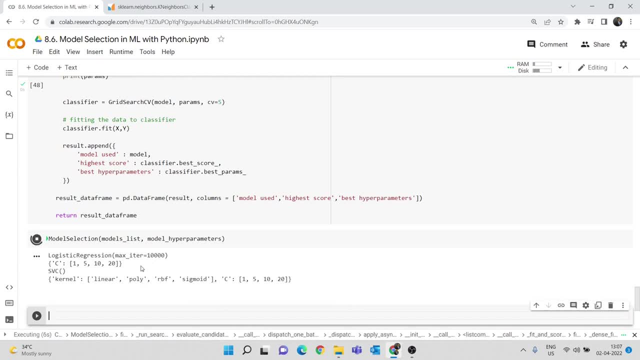 So training the support active classifier will take a bit more time because we are considering like two set of hyper parameters in this case. So what happens is like in the first set of cases, logistic regression will be trained for these different hyper parameters. c is 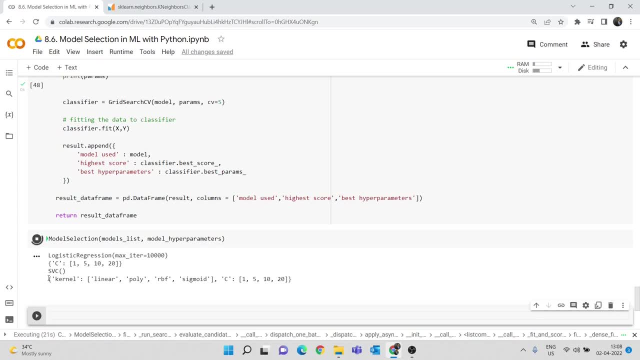 equal to 1, c is equal to 5, 10,, 20 and so on. And after that, for support active classifier we will train with, the kernel is equal to linear and c is equal to 1, then kernel is equal to linear and c is equal to 5, then linear 10, linear 20, and then after that, 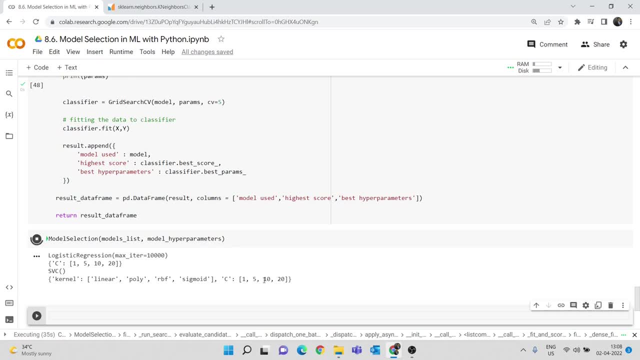 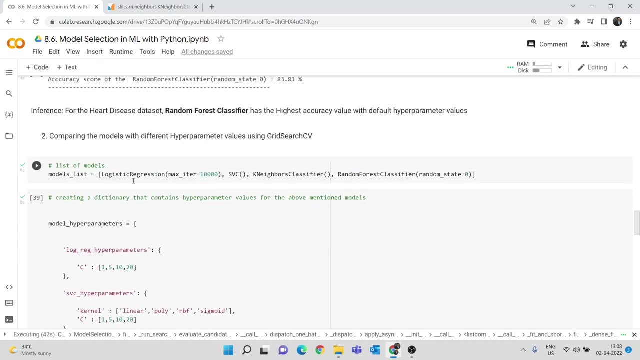 kernel, poly And c value of 1,, 5,, 10,, 20,. all this will be trained individually, and so on. So what happens here is so we have already created a list which contains the four models- logistic regression, SBC, k-nearest neighbor, random forest classifier- And we have created the 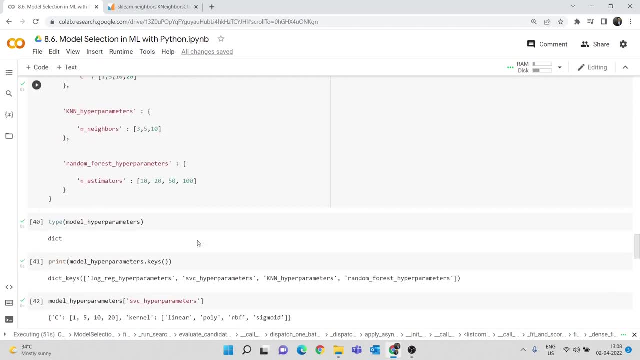 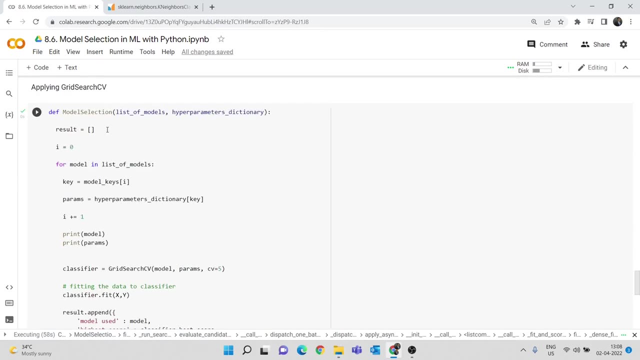 set of hyper parameter for the corresponding models as well, And then we have created this list called as model keys. So these three things are important, as I've told you before. Now we have created this function called as model selection and the two attributes. 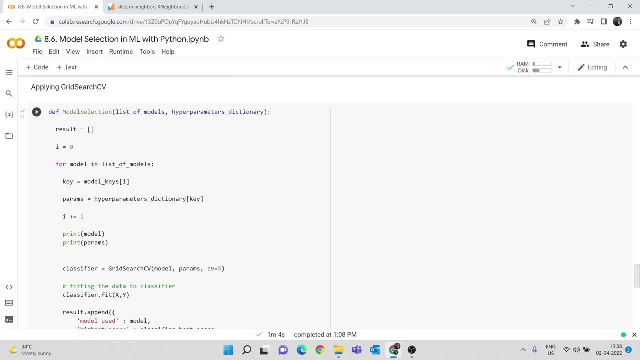 or parameters that this particular function takes are list of models and hyper parameters, dictionary. So you have to pass these two values to it And, within this function, what I'm doing here is I'm first creating an empty list, called as a result, And I'm creating 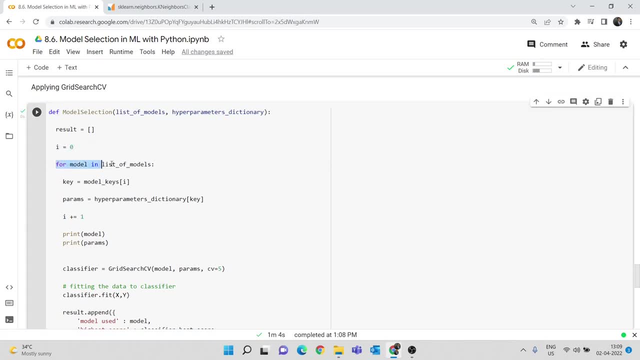 this i is equal to zero, And after that I'm performing this for model in list of models. So when the for loop runs for the first time it will check like what is the first value in this list of models? So the first value in the list of models is this logistic regression: 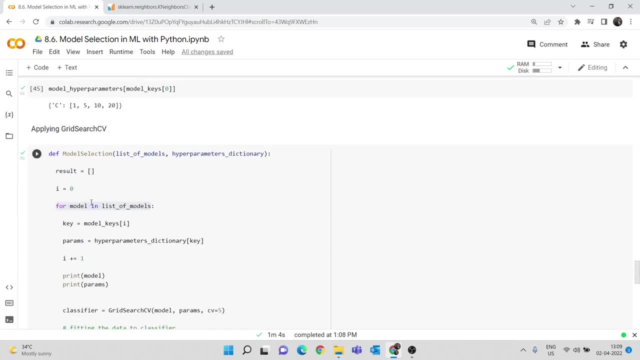 maximum meter 10,000.. So this model value will be logistic regression: maximum meter 10,000 and key is equal to model keys of i. So when I say model keys of i, the first time the for loop runs, the i value is zero because I have initiated the value here. So model: 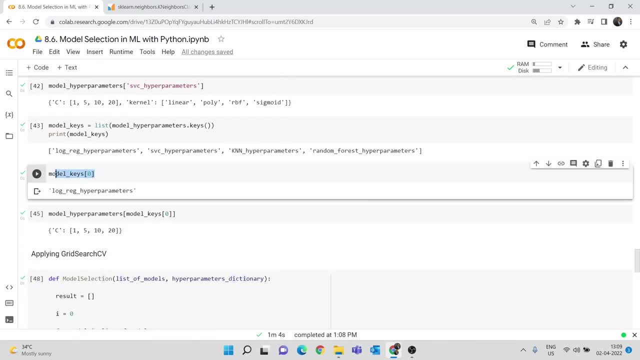 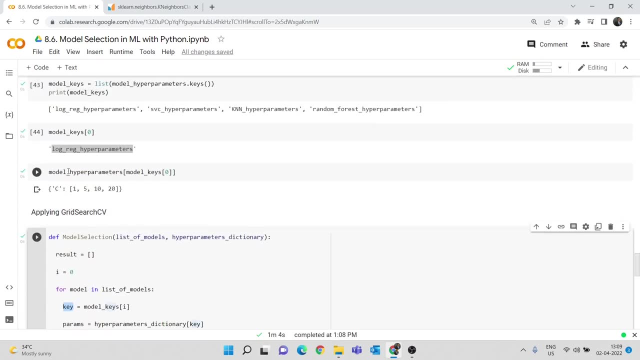 keys of zero is nothing, but it's same, or saying model keys of zero, which is equal to logistic regression hyper parameters, And so here the value of this key will be this logistic regression hyper parameters. So I have initiated that params. So here we are, passing the parameters of this logistic 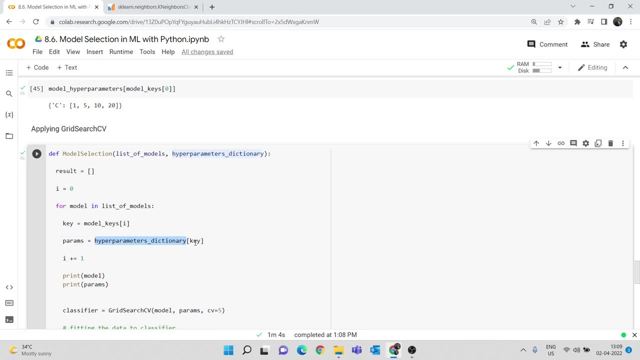 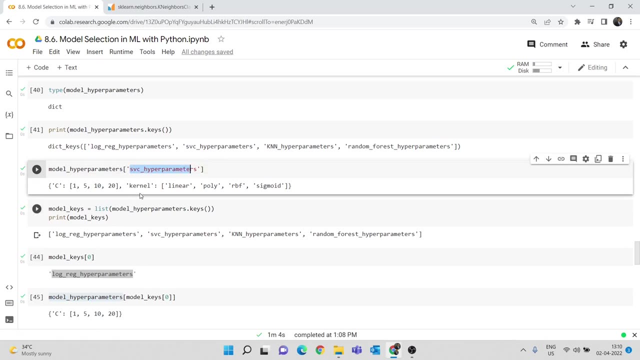 regression. So I'm calling that by parameters dictionary, which we are passing key. So it is similar to seeing model hyper parameters. Within this we are saying that logistic regression hyper parameters, Okay. so let me just copy this and paste it here. So it is like similar. 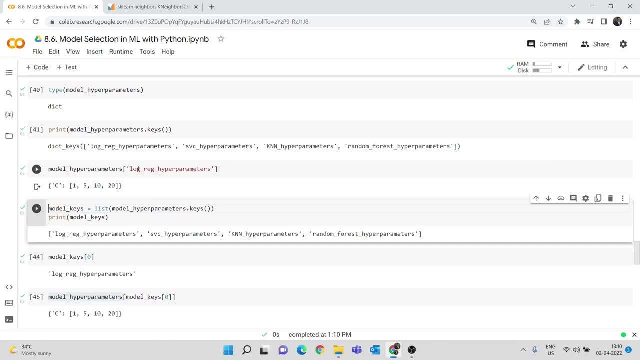 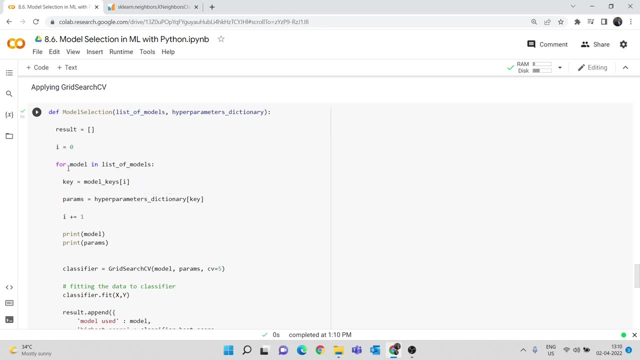 like same way of saying this. So instead of saying model hyper parameters of logistic regression hyper parameters, I'm going to say params- hyper parameter dictionary key. So it is like both of the same things. So, as we are doing this in for loop, this is more efficient way of doing this. And after: 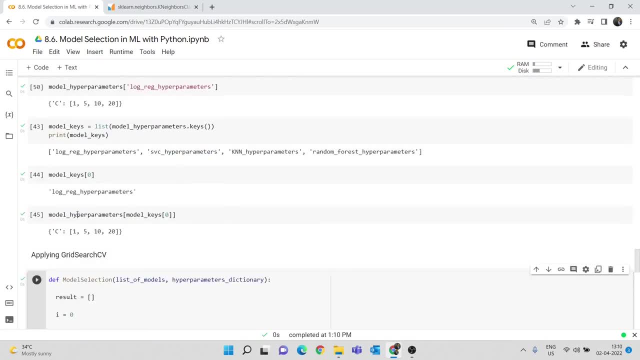 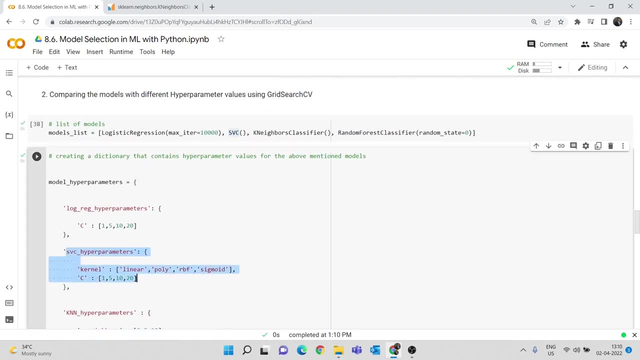 that I am incrementing this i value. So the reason is that the second time the for loop runs, it will take the model as SVC and it will automatically choose this SVC hyper parameters. If you don't increment this, i plus i is equal to i plus one. So in that case, what happens? 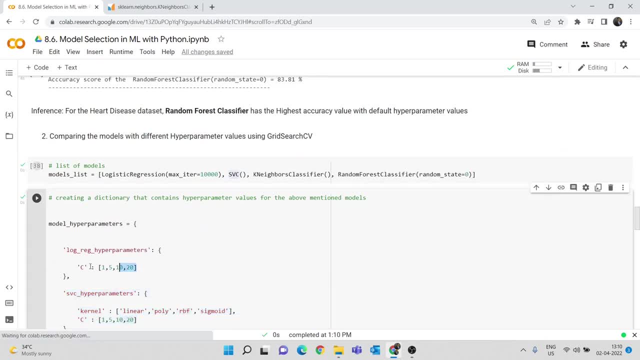 is that the model that is trained will be SVC and hyper parameter will be considered as these hyper parameters. So we don't want that right. So we want logistic regression and the corresponding logistic regression parameters, svc and this hyper parameters. so that's why we are incrementing this. i so first, 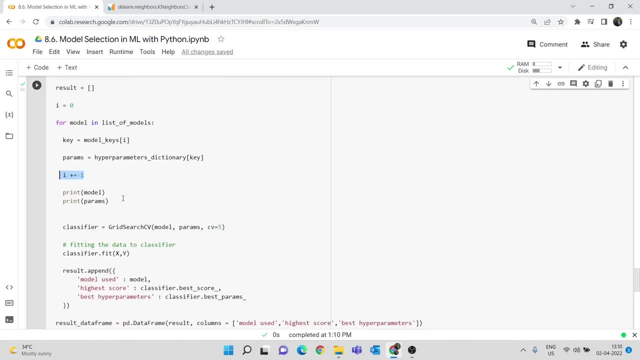 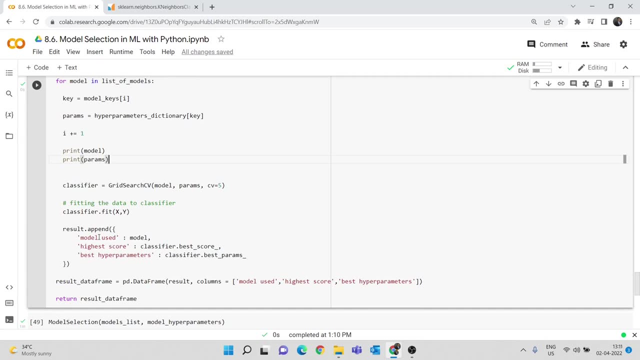 we have initiated this and we are incrementing this, and every time we are just printing the models and the parameters that we are using. so we are printing it and after that we are training a grid search, cv, and, and we are printing the best results and so on. so this is the first. 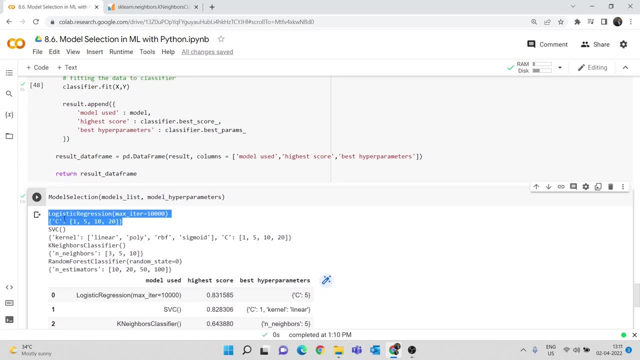 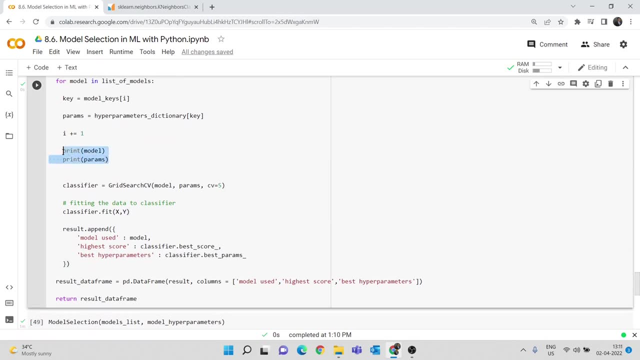 set of value for which the grid search cv is trained first. with you know, it will train the logistic regression model with c value 1, 5, 10 and 2: 1. so this is what we are printing here. print model and print params is what is happening here. so this is when the for loop runs the first. 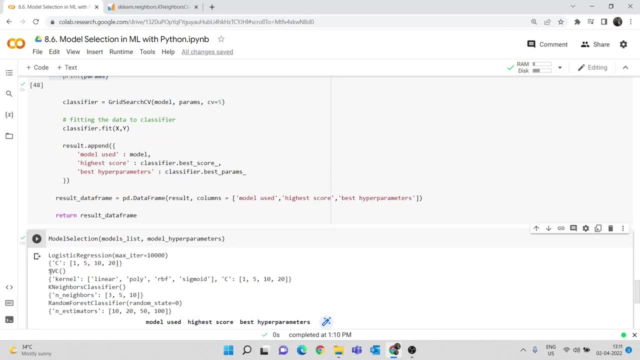 time and after that we are training us. so the for loop, so totally the for loop, runs for four times. the second time it runs it will train our supported classifier and it will check for this. these different hyper parameters, linear, poly, rbf and sigma, these values. so third time it runs. 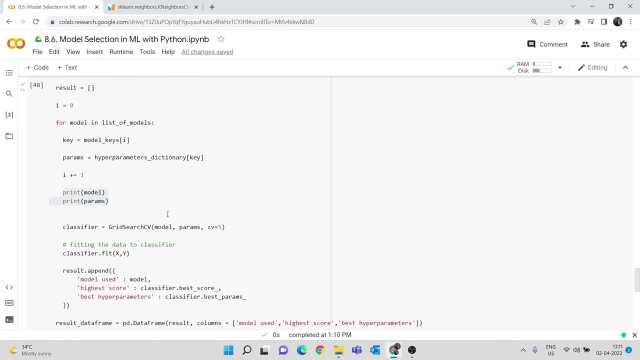 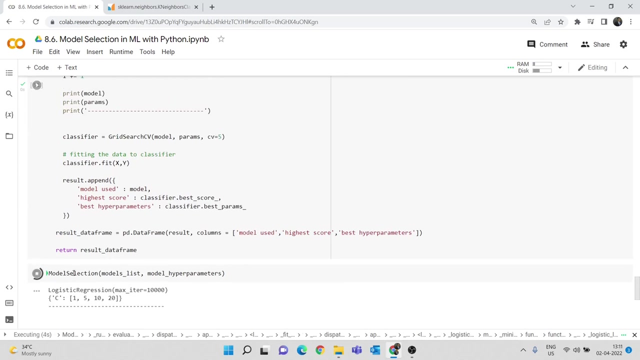 it will train with this k- nearest neighbors classifier, and so on. i'll also, you know, put another dotted lines here so that you kind of understand the count of this for loop. let me run this again. okay, okay, so this will take some time. okay, so this is when the follow branch for the first. 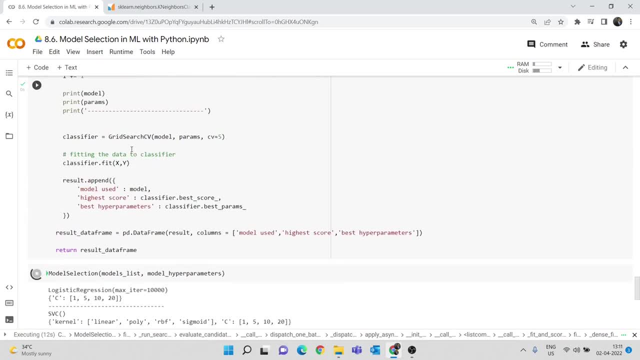 time. this is when it runs for the second time. so here we are passing this grid search cv. so again, if you want to understand this performance or how this grid search cv works, please watch my videos on hyper parameter tuning- uh, like a theoretical video- as well as the 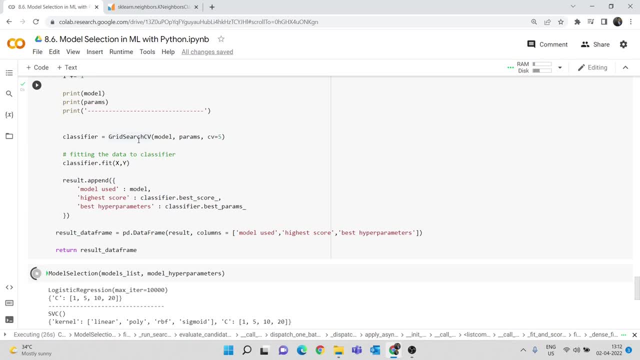 amazon video that we did. i'll also give the link of that video in this video description, so you just have to- you know, watch all the videos in my modulate. there are like five or six videos, so please watch all those videos. uh, this is like 8.6, so watch all the five. 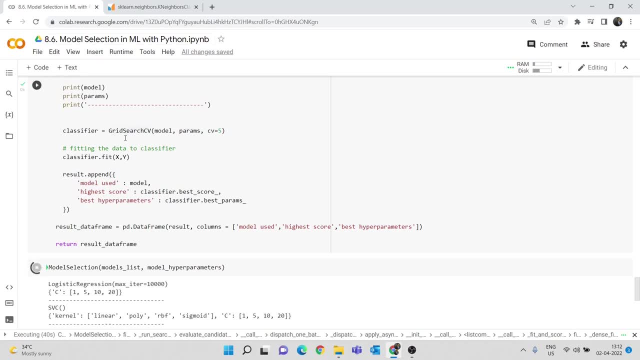 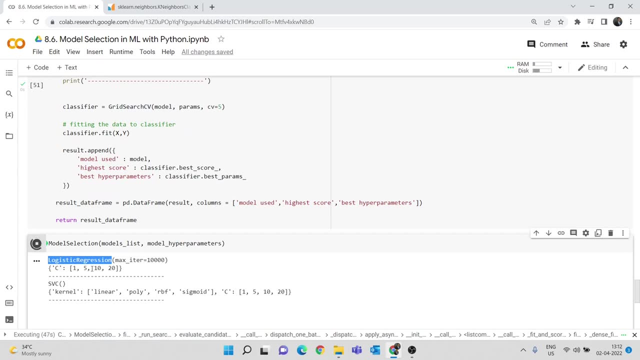 previous videos. so then only you can understand this clearly. so grid search cv. what it basically does is so it will take a model like logistic regression and it will try to find the accuracy score when we are using, like this, different type of parameters. so when you are using, c is equal to 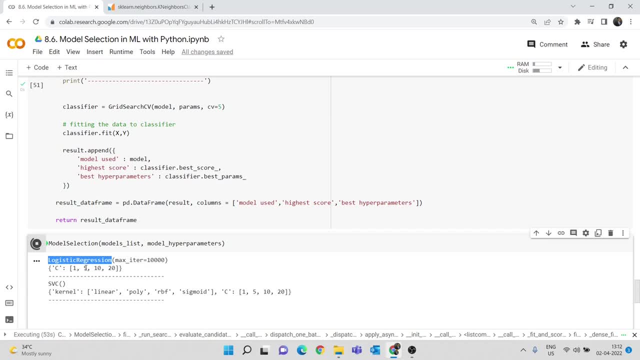 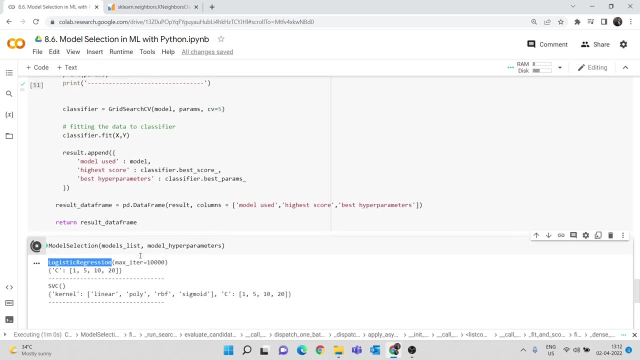 one. you will have an accuracy score like, let's say, 80, and let's say, when we are using the hyper parameter, value of c is equal to 5, we will get a different accuracy score and so on. so it will calculate all those accuracy scores. so each time the follow prints we will check this for each. 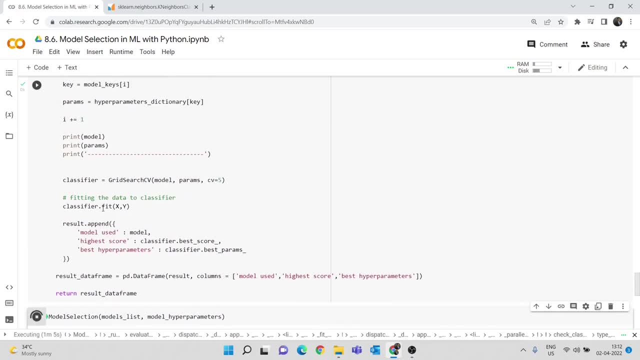 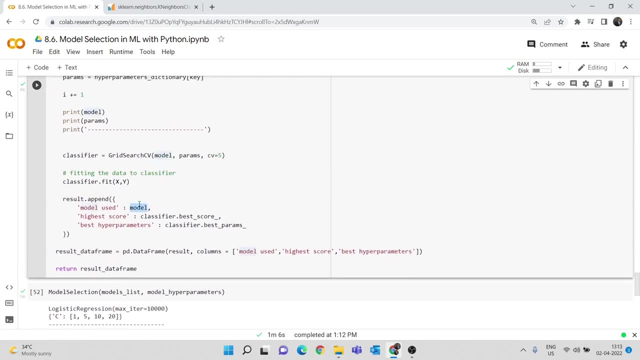 model that we are considering. after that, once we are, you know, completing this training and so on, we are finding the best results. so i am saying, like model used is equal to model, so this model is nothing but the values that i am taking from the list of models. so this one, so there's logistic. 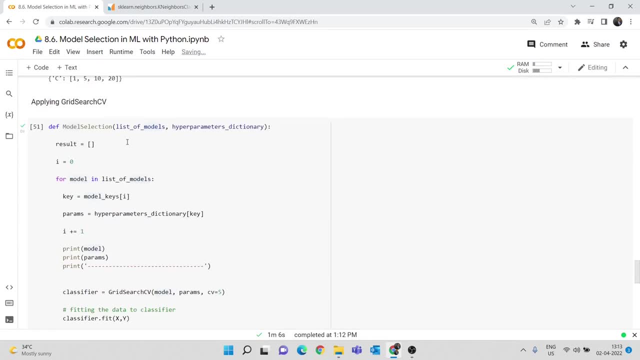 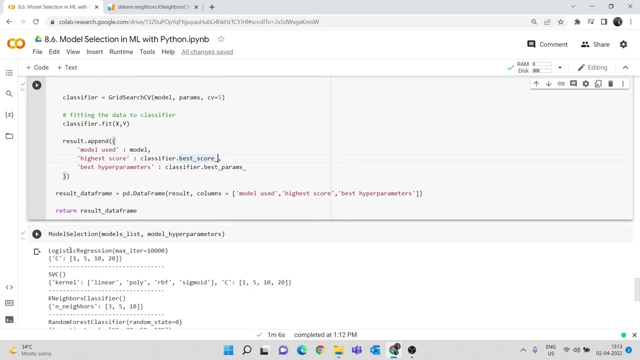 regression. so first time the value for this model is model, and then we have this classified or best score. so what happens is like it will tell you what is the highest accuracy that particular model has read. so what is the for all these five, oh sorry, four considerations of this hyper? 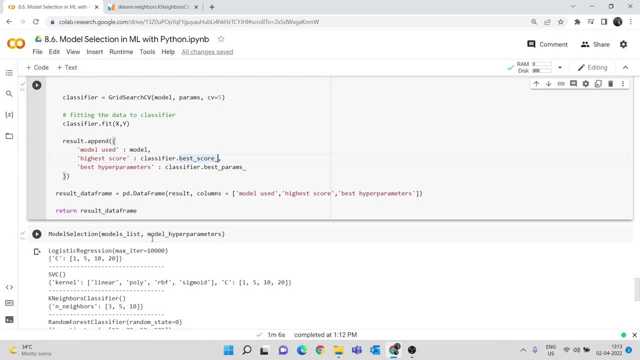 parameter for 1, 5, 10 and 20. what is the highest accuracy that you are getting and what is the best parameter? so best parameter means for which hyper parameter you are getting highest accuracy, whether you are getting the is accuracy when using pi or you are getting is accuracy while using 20. 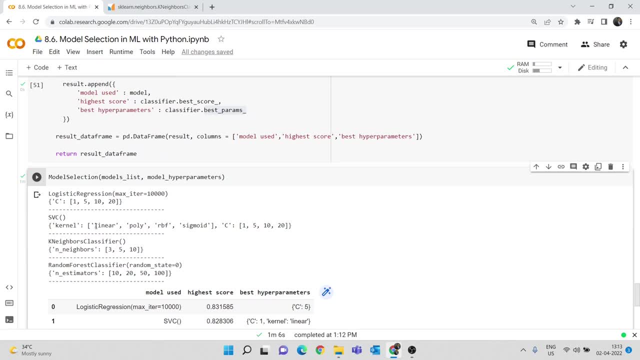 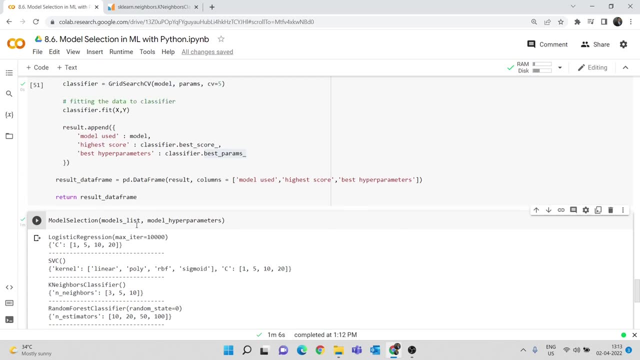 and so on, and similarly we get for all these things. so for which set of, for which combination of this kernel and c you are getting is to value, and you know what is the is accuracy and so on, and we are just loading it in a pandas data frame, right, and we are creating this column names as model used. 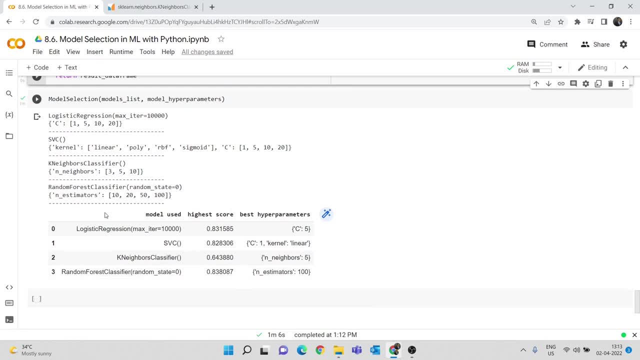 is for and best parameter. and this is our final research. okay, so, as we can see. so we have used like four models. so this is the first column name of the model used: what is the is accuracy for that particular model and what is the best hyper parameters for that model. so 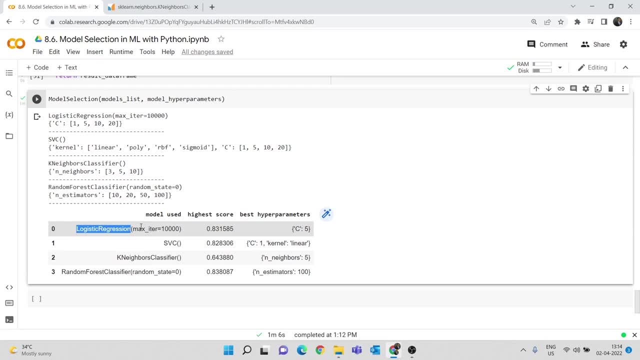 uh, how we have to infer this is when using logistic regression. the highest accuracy score that we are getting is 0.8315, which is equal to 83.15 percentage. so this is, in this, uh, zero like in the range of zero to one. so this is actually the percentage. 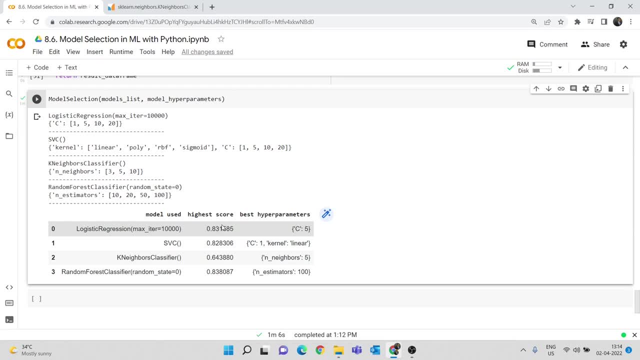 value. you can just uh calculate this one and you are getting. this is accuracy of 83 percentage when you are giving the c value as 5. and if we come to the next one, when you know when, using a supported classifier, the is accuracy that you are getting is. 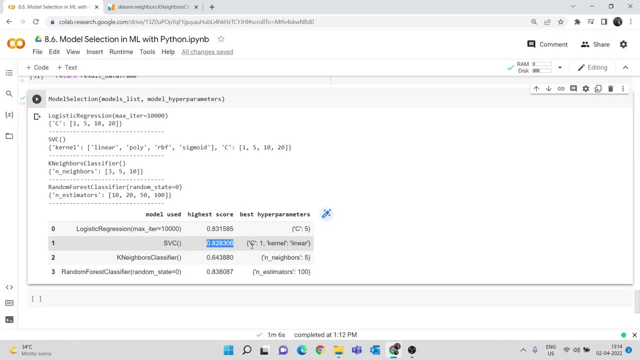 82.8, almost 83 days, and you are getting this highest value while you are giving the hyper parameter values, as c is equal to 1 and kernel is equal to linear, so while using this hyper parameter, you are getting the highest value. so this is for k nearest neighbor. so instead, like if you use 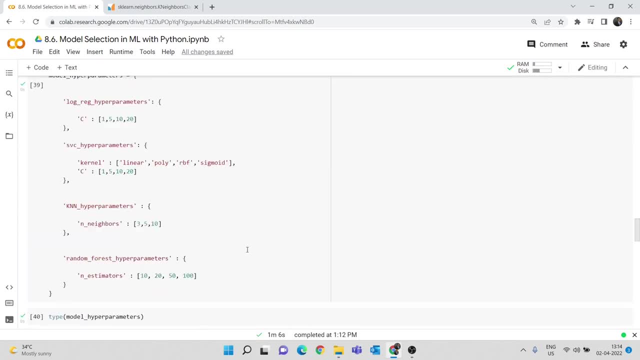 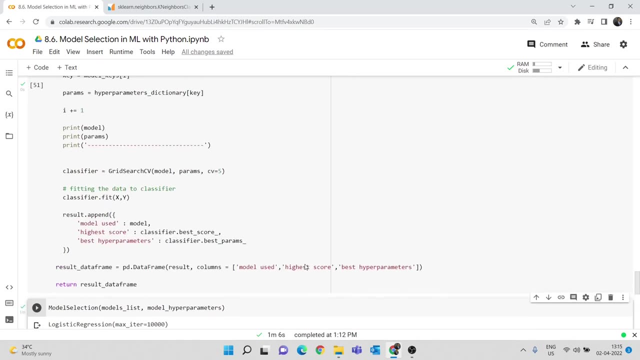 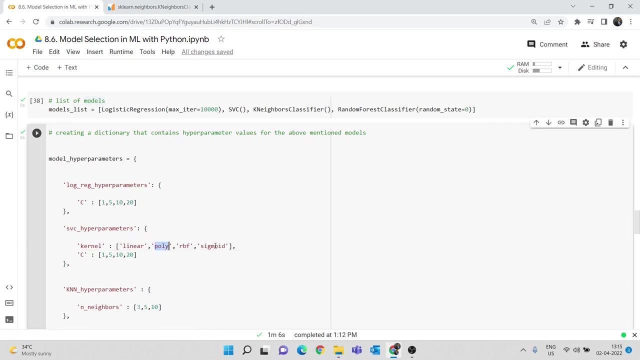 different k nearest neighbor values like uh, as we have mentioned here, 3, 5, you will get less values. sorry, i think. like the value is 5, right, okay, so n neighbors value is 5.. so instead of using a n value, use 3 and 10. you will get less value. Similarly, if you use poly RBA for sigmoid and if you 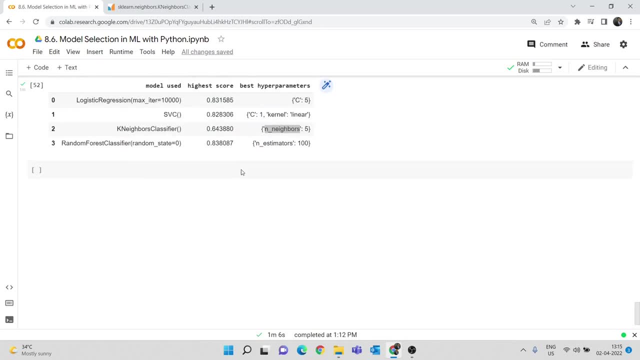 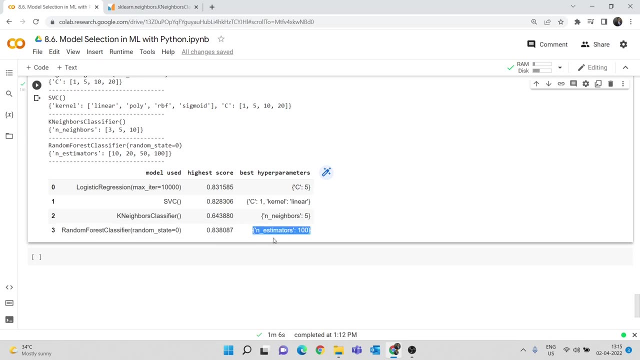 use like 5, 10 and 20, you will get less lesser accuracy score. So that is what we are understanding from here and for random forest classifier, 83.8 is the highest accuracy that we are getting and we are getting that when we are using the n estimator is equal to 100.. If you use 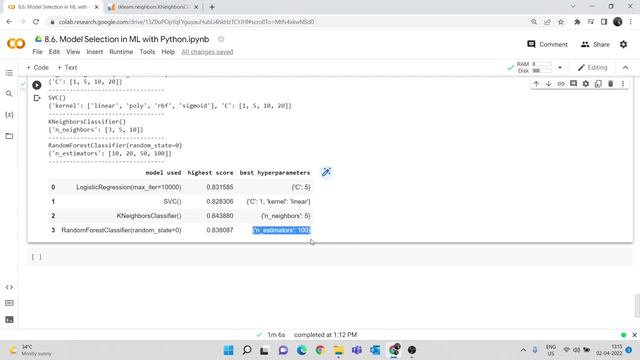 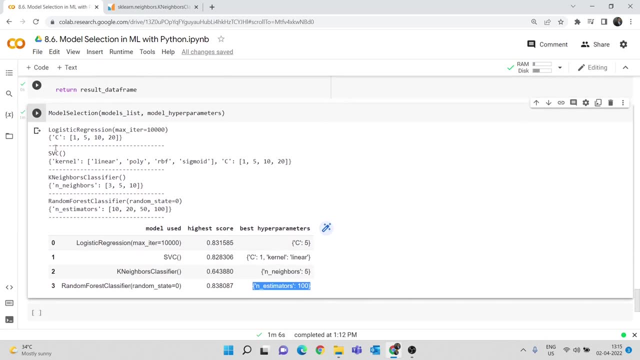 like 50,, 40 or 30, we are not getting highest accuracy. So this is how you can compare different, not only like models with default hyper parameters, but with different set of hyper parameter values. So these are all the different hyper parameters that we have. 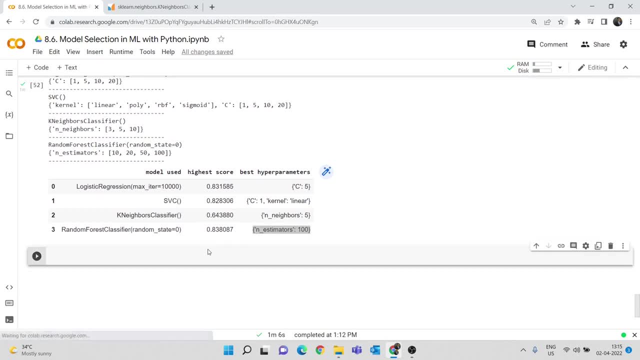 considered and, once we have, you know, come to this conclusion. So now we will split our data into our training data and test data and, instead of training it with logistic regression or SPC or k nearest neighbor, we will train our random forest classifier model and the 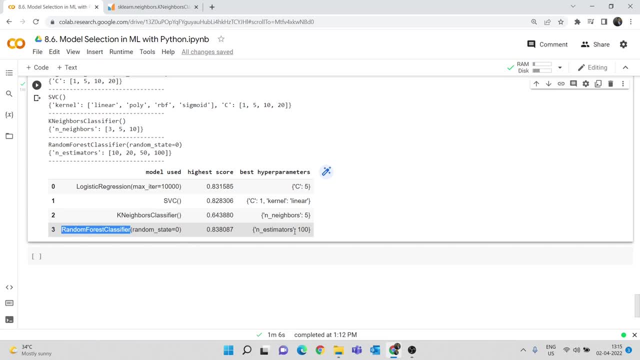 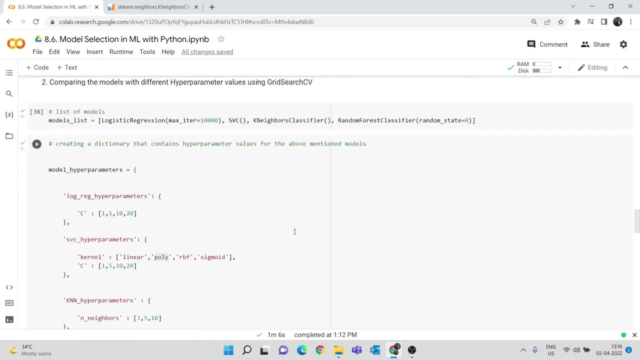 important thing is we will choose this: n estimator is equal to 100.. So this is how you can kind of do model selection as well as hyper parameter tuning for multiple models. So in this case I have just considered like few hyper parameters So that this code kind of looks. 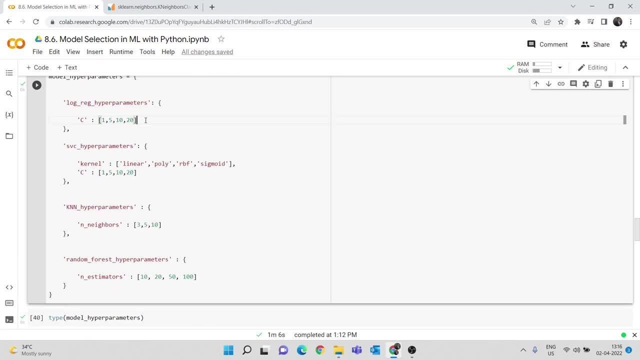 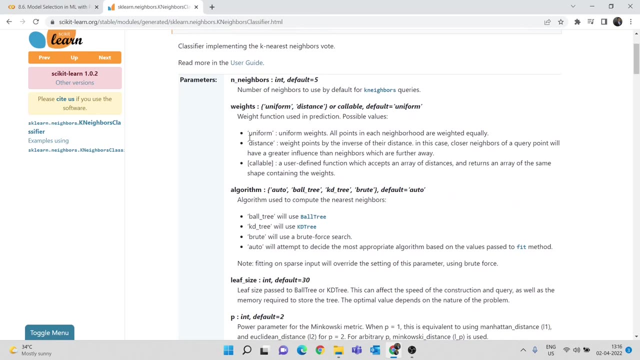 simple. So, apart from the c, we also have different hyper parameters for logistic regression and for k nearest neighbor, as well as for random forest hyper, like random forest also. So if you see this, you know k nearest neighbor. we also have this different set of values. 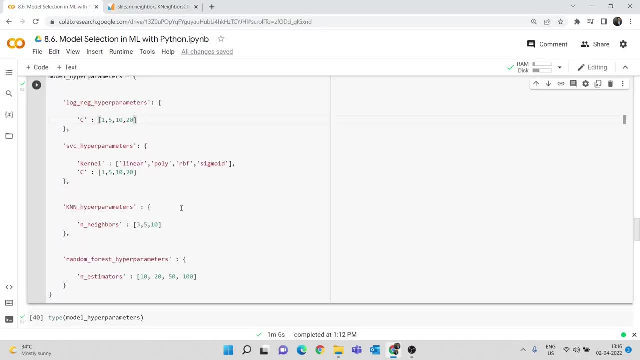 that we can consider. So along with this, you know n neighbors, so you can just put a comma here and you can just create a list with all these values as well. So this is just similar to this. kernel and c. So here we have considered two hyper parameters in. 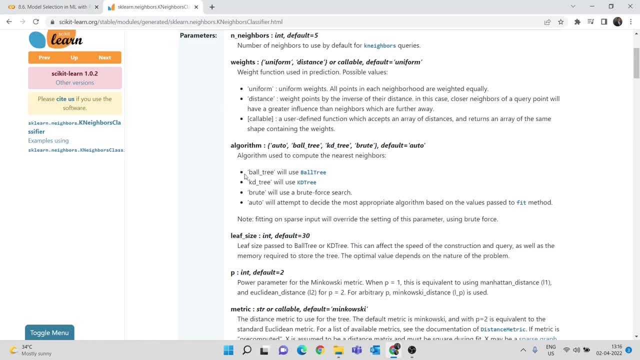 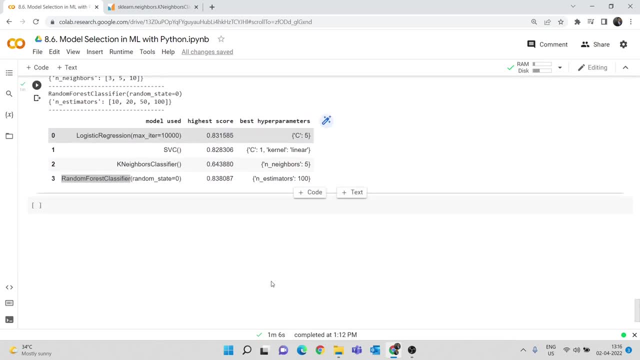 other cases. we have just considered only one hyper parameter. So you can also use these hyper parameters as well and you can train that for that combination as well. So this is how you kind of you can do this model selection and hyper parameter tuning. So once you have done that, once you have find you know which is the best model. 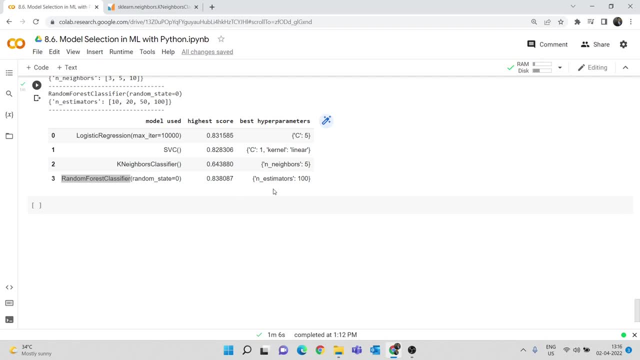 and best hyper parameter. do a train test, split and train with that particular hyper parameter. So what will be the next step here is: I will split by x and y, So I have this x and y right, So I have this x and y. So I will split this x and y to training data and test. 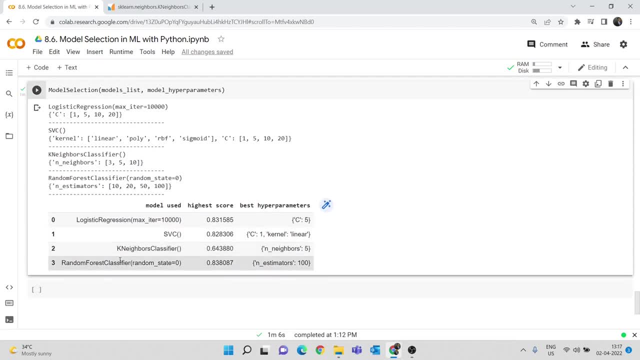 data. So I will train my training data with my random forest classifier and I will pass my n estimator value as 100. So this is the best result I get. So this is how we can, you know, do this model selection in python. So let me just put a text here as my inference. 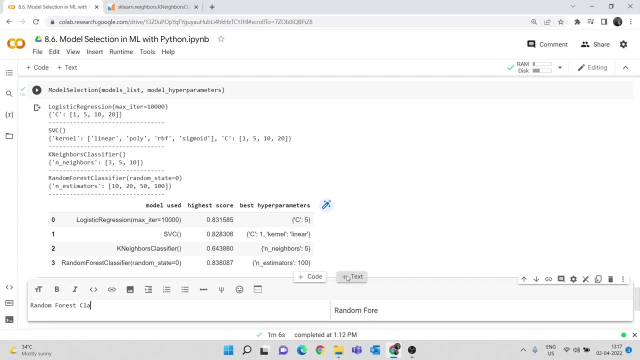 random forest classifier seem to have the highest accuracy. Let me put this as random forest classifier with n estimator value as 100.. So this is how we can do this model selection in python. So let me just put a text here as my inference: random forest classifier. 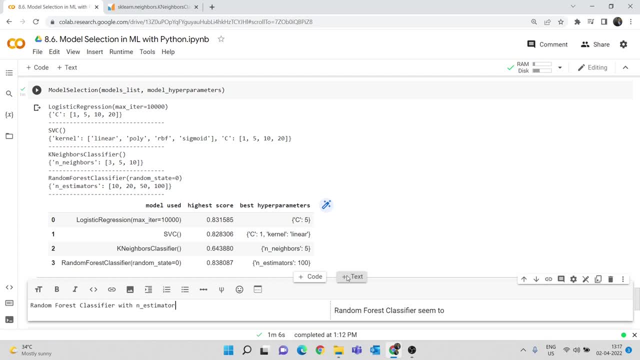 with n estimator value as 100.. So let me just put n estimators is equal to 100 as the highest accuracy. okay, okay. So yes, accuracy, and it is not like this, only the result that you get. So if you consider different hyper parameters, there can be different results. 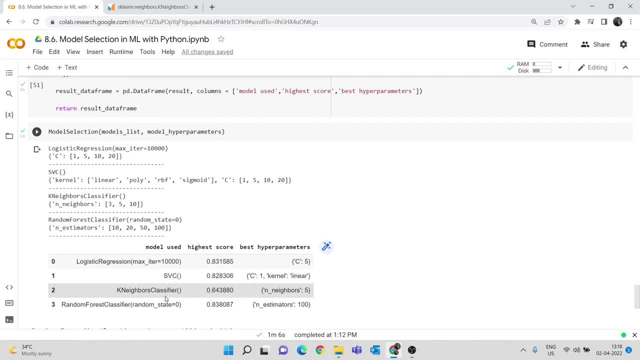 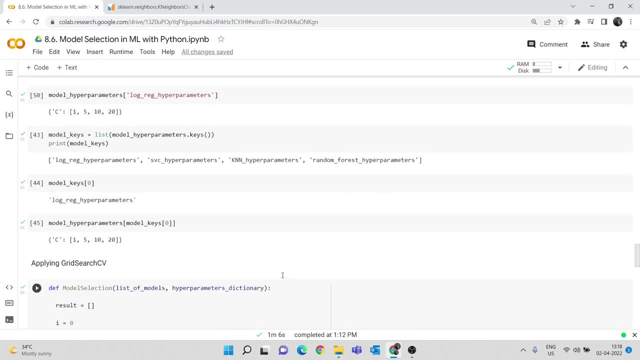 also. You may also get like: container receiver can also be a good model, but it is like highly unlikely hyper parameter. you may you may get a different result in this case. i just considered only like uh, one parameter in each case, except for spc, where we are considered two hyper parameters. 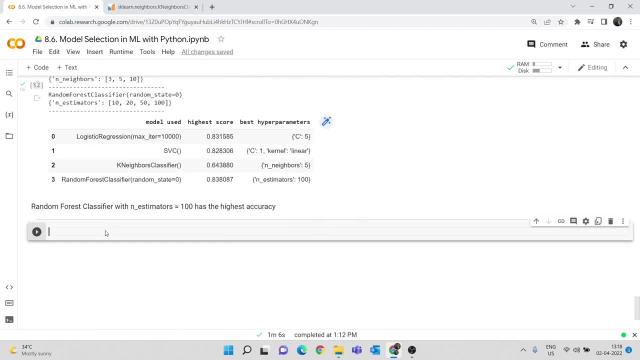 so you can try that will, where you can, you know, consider different hyper parameters as well, and i hope that you have understood all the contents uh covered in this video. and that's it from my side and i'll see in the next upload. thanks for watching.